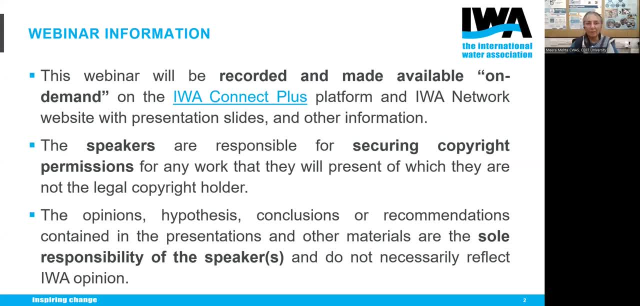 Connect Plus platform, an IWA network website with presentation slides and other information. The speakers will be responsible for securing copyright permissions for any work that they present and which they are not if they are not the legal copyright holder. The opinions, hypothesis, conclusions, recommendations in these presentations and other materials are: 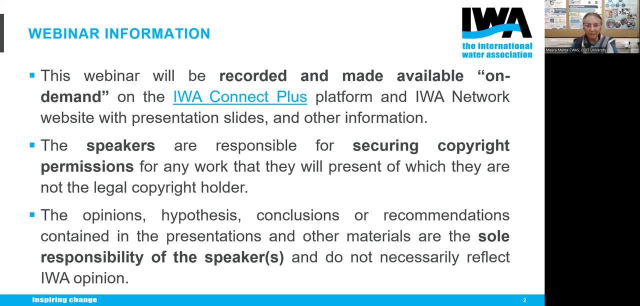 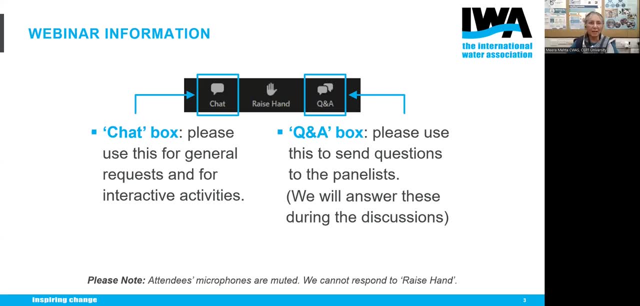 their sole responsibility of the speakers and do not necessarily reflect IWA opinion. Just to give a before we actually start on the webinar, there are two facilities that are provided. One is chat box and the other is a question and answer box. Please feel free to participate actively in this and the attendees microphones are muted. 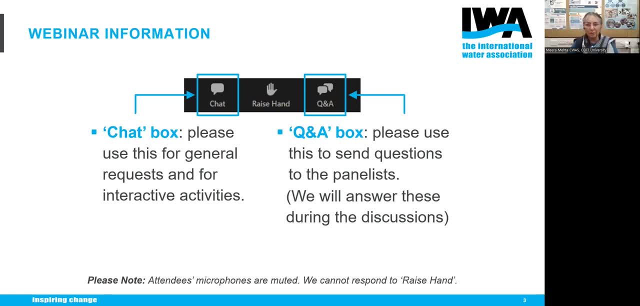 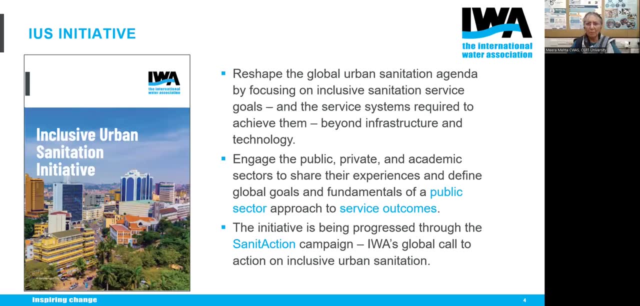 but you can participate through this activity and your questions will be taken up to the extent that it's possible. This is also part of the Global Inclusive Urban Sanitation Initiative of the IWA. This is it focuses particularly on inclusive sanitation service goals and the service systems that are. 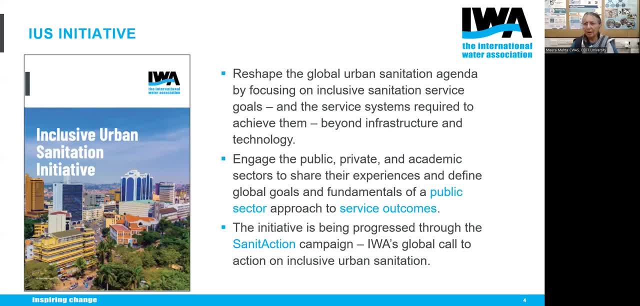 required to achieve them, And it emphasizes that it's not enough to focus on only infrastructure and technology, but look beyond to other aspects, And the major aspect that today will be discussed is on looking at data systems that are absolutely essential for monitoring of these services. 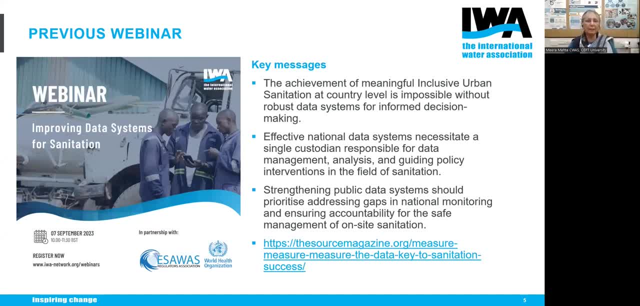 We had done, in fact, a webinar at the last IWA event in Kigali and which focused exactly on the same topic, on improving data systems for sanitation. There was very active participation and some of the speakers that are there today, in fact, were also. 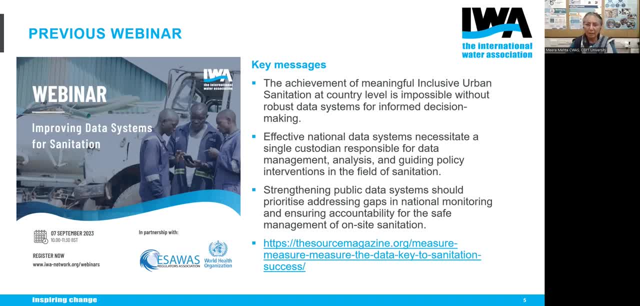 participating in that And we had contributions from Bangladesh and from Uganda at that workshop, at that seminar. So this is really a continuation of that workshop to take forward the discussions and particularly focusing on inclusive sanitation agenda and looking at sanitation whole sanitation service chain and sanitation systems that look at not only 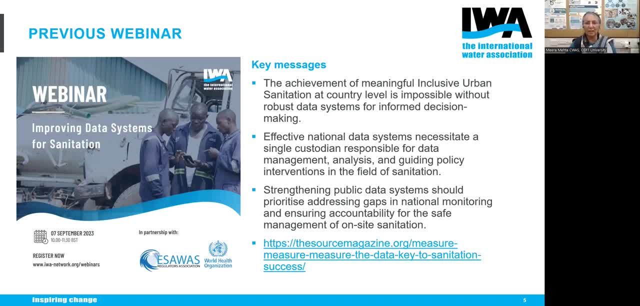 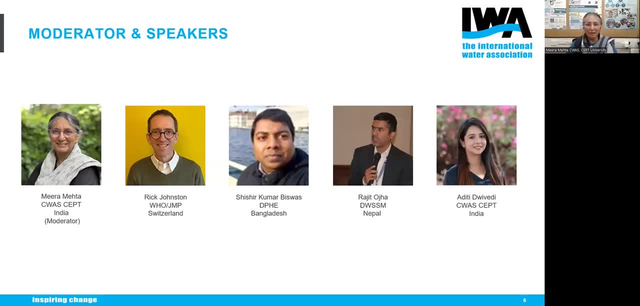 sewerage, as was in the past, but also look at on-site sanitation systems. We are going to have four speakers and I will introduce them as we go along, but they are from Rick Johnson from WHO, Shishir Vishwat from DPHE, Bangladesh. Rajit Toza from Nepal, DWSSM. 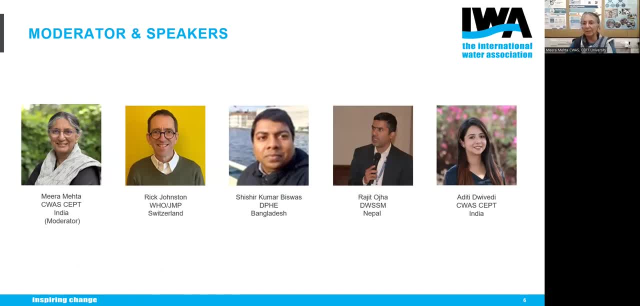 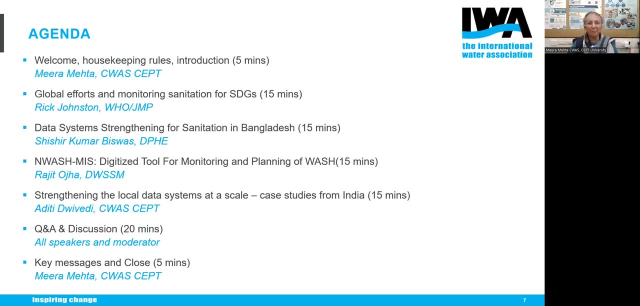 and Aditi Dwivedi from CWASEP here in India. So this is broadly the agenda We will have. first, after the welcome, we'll have presentation by Rick from WHO-JMP on the global efforts particularly. Then we will have the presentation from Bangladesh looking at data systems. reasoning for sanitation. 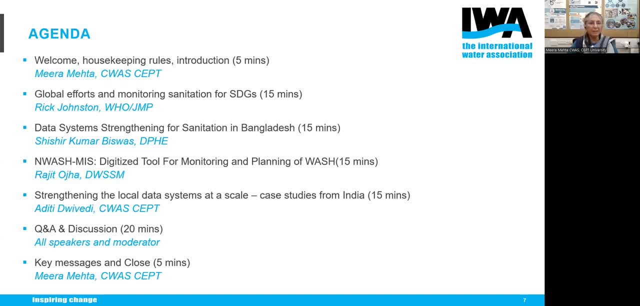 the activities that are ongoing in Bangladesh by Shishir Kumar. Rajit Toza, then, will present for NWASH-MIS and the activities that are ongoing in Nepal And, lastly, not last but not the least, the presentation from Aditi Dwivedi, from here at our institute, CWASEP, looking at cases from: 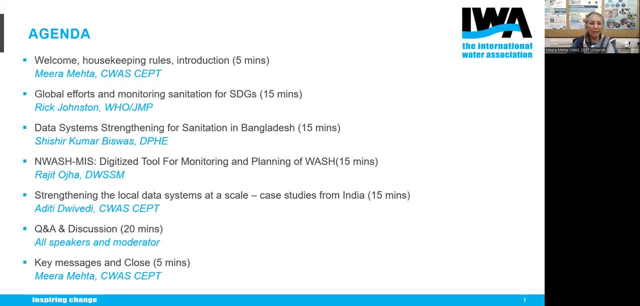 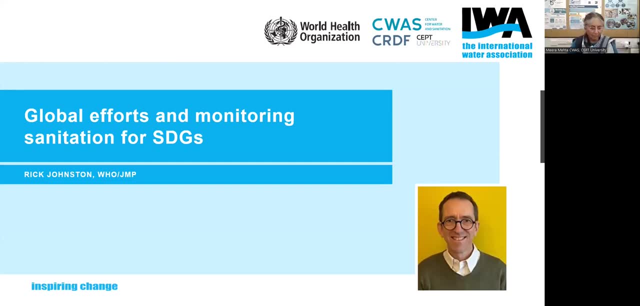 India, where similar activities have been going on, And we'll end with question and answer discussion to the extent possible, So I'll now invite Rick to have the first presentation. We are really fortunate to have Rick Johnson join us for this webinar. Rick has been with WHO for 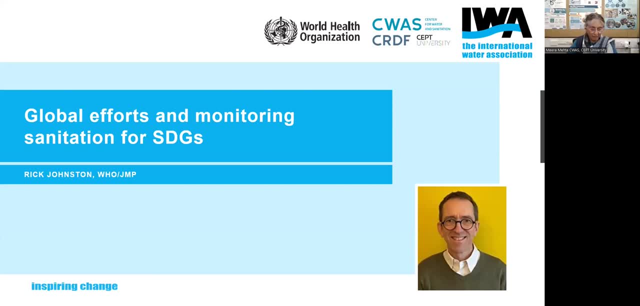 decades and leads the work on sanitation for the JMP. He has been at the forefront in developing approaches to respond to the new thinking in sanitation And, on a more personal note, Rick has always been very open to feedback and discussions Whenever we've approached him for any 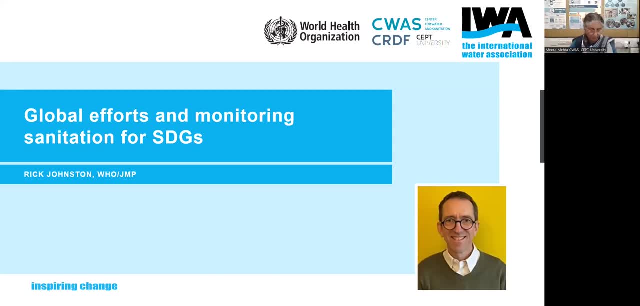 work, any activities, he's always there to help us. I would request Rick to then start the presentation. Thanks so much, Meera, for the kind words, And it's always been a pleasure to engage with you as well. So I am Rick Johnston. I'm with the. 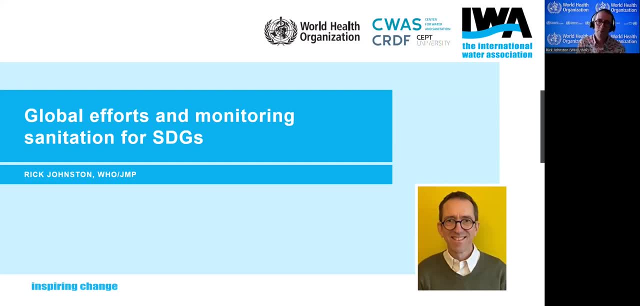 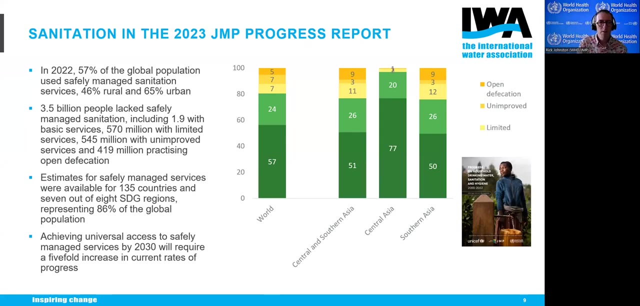 WHO. I lead the WHO side of the Joint Monitoring Program, which is joint with UNICEF. My colleague Tom Slaymaker leads on that side, And today I wanted to talk about our work on monitoring sanitation at the global level. Good, So, last year the JMP published a progress report And you can 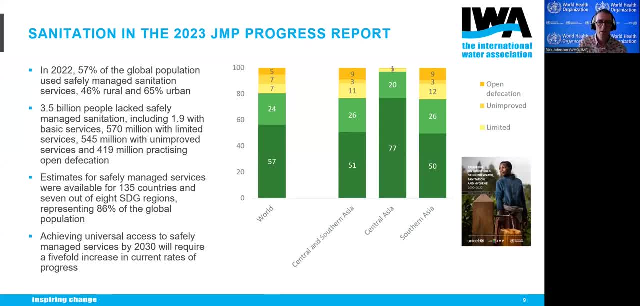 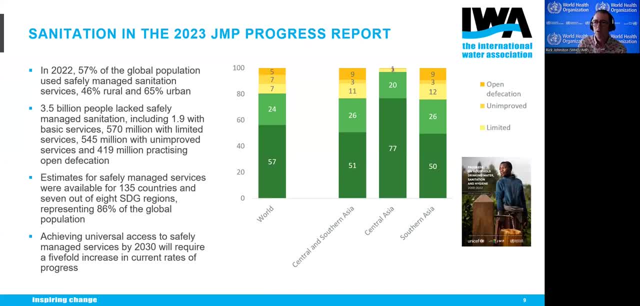 is safety-managed sanitation, So in 2022, about 57% of the global population used safety-managed sanitation services. It was higher in urban than in rural areas, but that means that there were about 3.5 billion people who didn't have safety-managed. 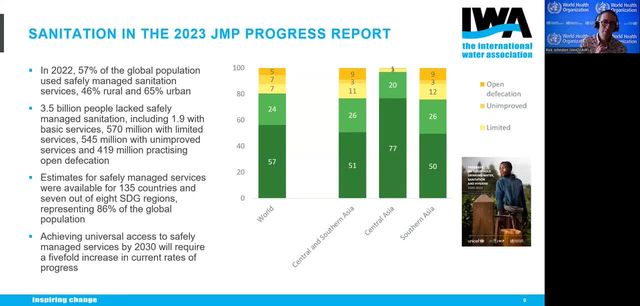 sanitation services, including 419 million practicing open defecation. So the data coverage continues to grow from report to report. We had estimates for 135 countries in last year's report. that represent about 86% of the global population, So that's pretty high. 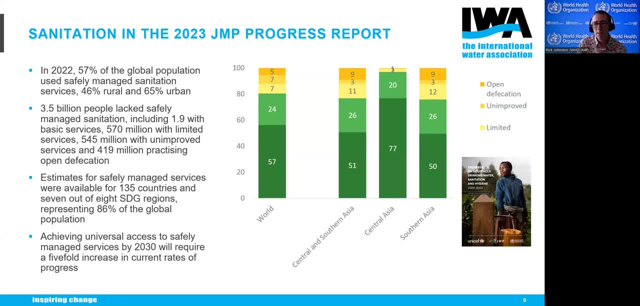 coverage. It also allows us to look at trends and we can see that the rate of progress historically has not been fast enough to get to 100% by 2030.. In fact, to reach that level we would have to be moving five times faster than the historical rate of progress. So there's 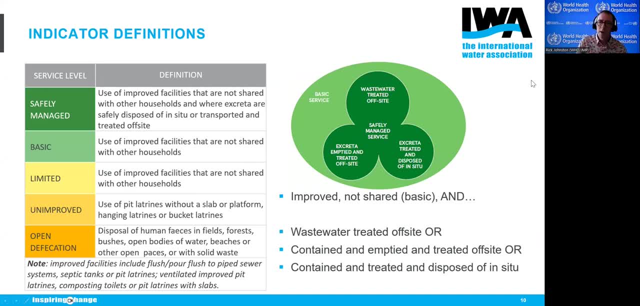 definitely need for acceleration. I just wanted to remind people about the definitions. The JMP uses this service ladder with different service levels, ranging from no service at all and open defecation up to safely managed at the top. The top three rungs: safely managed, basic and limited. those are all households that are using improved sanitation. 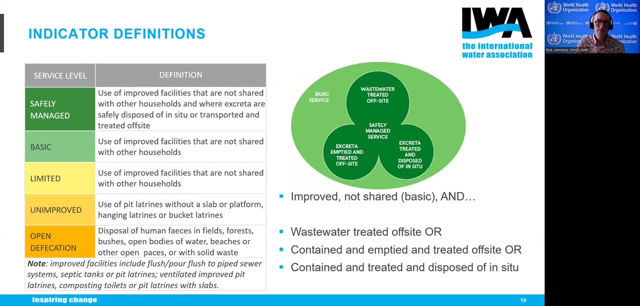 facilities. If they're shared, it counts as a limited service. If they're not shared, it's a basic service. But in order to be safely managed- there are different ways to be counted as safely managed. It has to be improved and not shared first, but then it could be waste-washed. 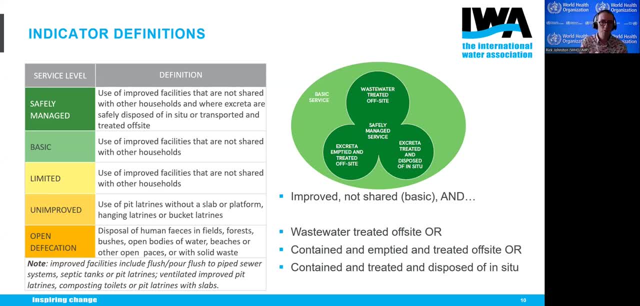 or it could be water that's treated offsite, That's, through a sewer connection that reaches a treatment plant that provides at least secondary treatment, Or it could be an onsite sanitation facility that actually contains the waste safely, and the wastes are either emptied and treated. 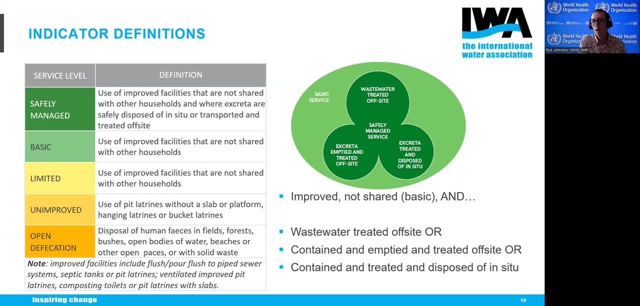 offsite- You can think about fecal sludge management and trucks and FSTPs- Or it's contained but it's not emptied and it's treated and disposed of in situ. So we call those three different pathways into safely managed sanitation. 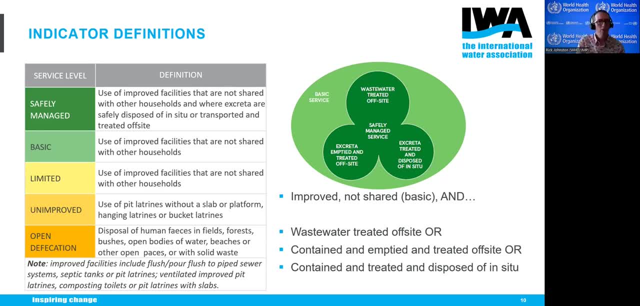 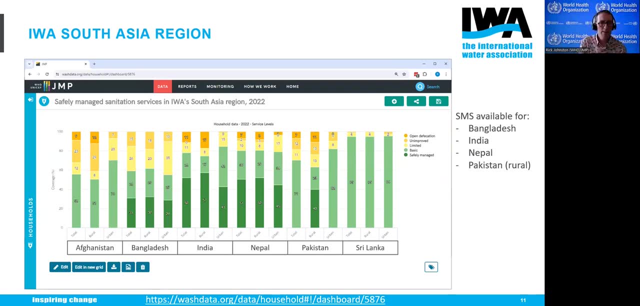 I'll talk a little bit more about them on the following slides. The JMP has a website where you can look at country data or regional data. There's a little dashboard below where you can see the six countries in IWA's South Asia region. 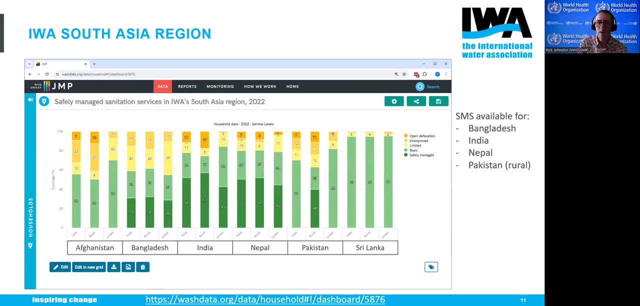 For three of those countries- Bangladesh, India and Nepal- there were enough nationally representative data to produce estimates for safely managed sanitation, And in those three countries it was possible to have also an urban-rural disaggregation, which always tells a better picture because you can really see which populations are having services and 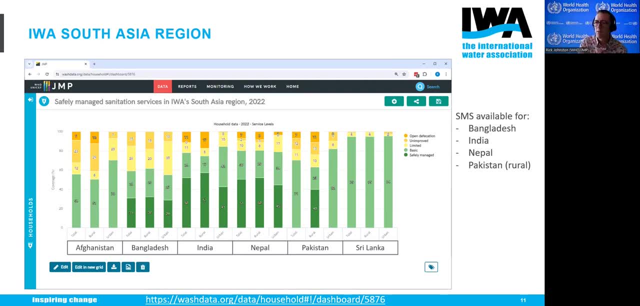 which ones are not. Also for Pakistan. you can see one of the bars has dark green. That's because there were enough data to make an estimate for safely managed sanitation in rural areas but not in urban areas, Whereas the other three countries- Afghanistan, Pakistan and Sri Lanka. 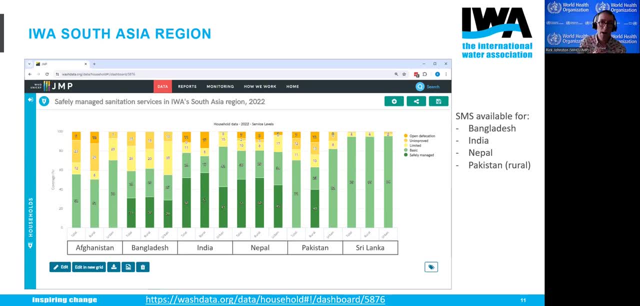 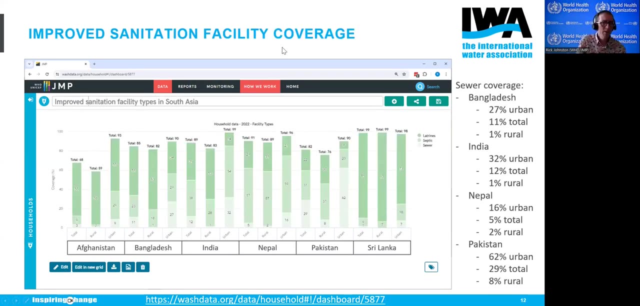 we didn't have sufficient national information, either at the national scale or urban or rural, to get safely managed, But we did have enough to track the other rungs. so basic, limited, unimproved and open defecation. So what's missing then? What are the data? 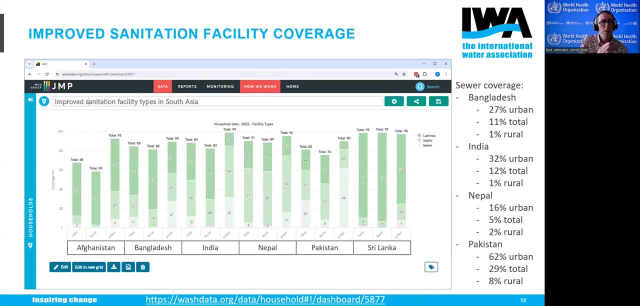 that are needed. Well, first I wanted to show what types of improved sanitation facilities are being used in these countries, And I know the colors aren't very different here on this graph. but the dark green- darkish green- represents improved latrines. The middle color: 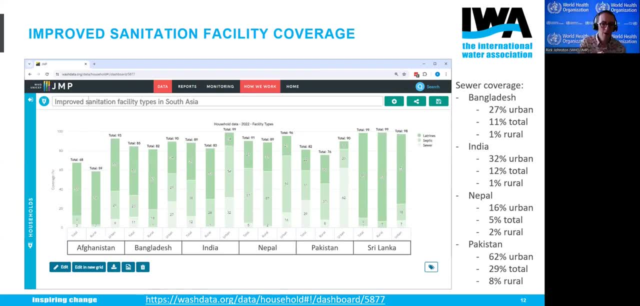 is septic tanks And the lightest color at the bottom is sewer coverage. And the thing that you can see quickly from this graph of these six countries is that sewer coverage is not very high in any of these countries. It's always higher in urban areas. In rural areas it's negligible in 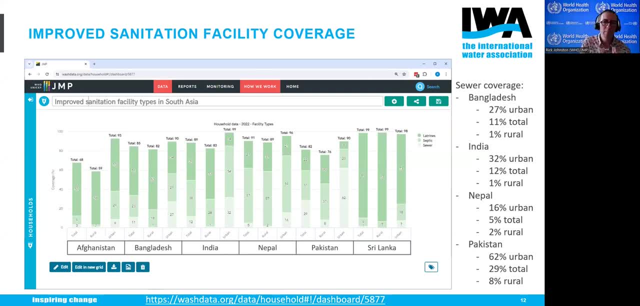 these countries, except for Pakistan, which seems to have about 8% of the rural population connected to the sewer lines, And indeed in Pakistan the urban coverage at 62% is the highest region in the world- And in other countries, even in rural, even in urban areas, we're talking about less than half. 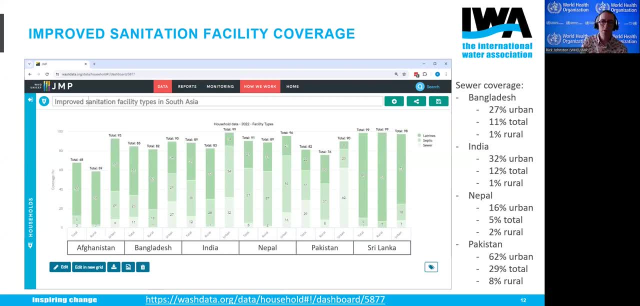 maybe up to a third, a quarter of the population having sewer connections, And what that means is that, okay, it's possible to have safety managed sanitation through sewer connections and if there are national data on wastewater treatment plants, But the majority of the 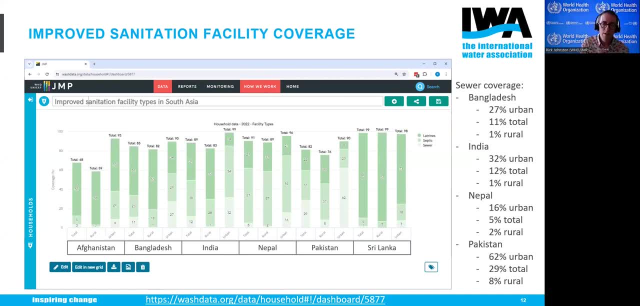 population doesn't have that. They're using onsite sanitation, So that has different data implications. It means you need to know well, are those onsite sanitation facilities really functioning? Are they containing waste? Are they filling up? What happens when they fill it up, When they get? 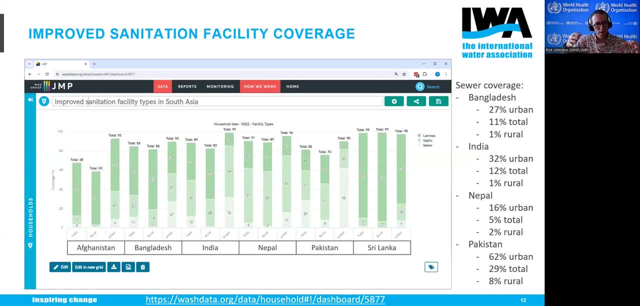 emptied? where does the waste go If they don't get emptied? do they get buried and stored in situ, Or do they get unsafely handled? So that's a very different kind of data question. then, And just before I leave this, I wanted to mention also that not only is onsite sanitation 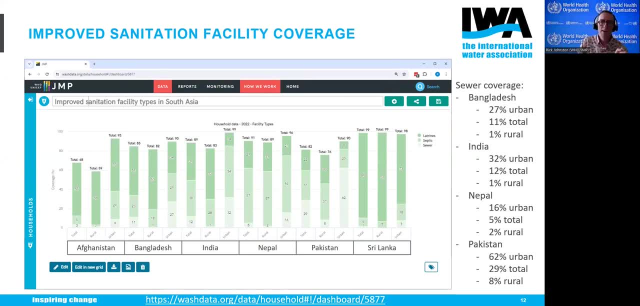 higher than sewer sanitation. growth in onsite sanitation is higher than sewer sanitation. It's higher than growth in sewer sanitation at the global level, even in urban areas. I'm not sure about the six countries in this region, So I mentioned data coverage and data gaps. 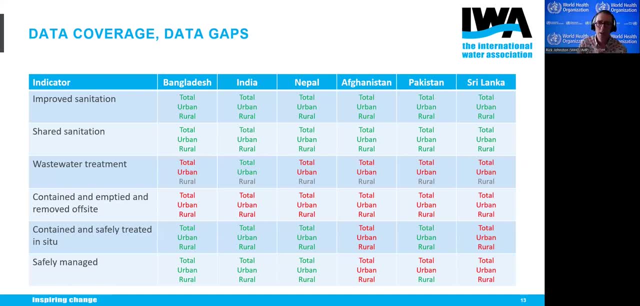 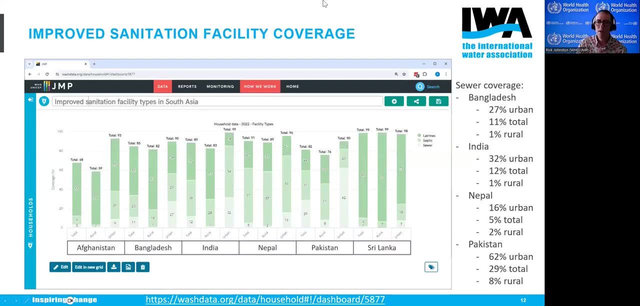 The first two rungs here show for these six countries the basic indicators that were used in the MDGs of improved sanitation and shared sanitation. data are widely available. This is routinely captured in all kinds of household surveys and we have data trends. oh, I'm sorry, I went the wrong way on the slide. Here we go. 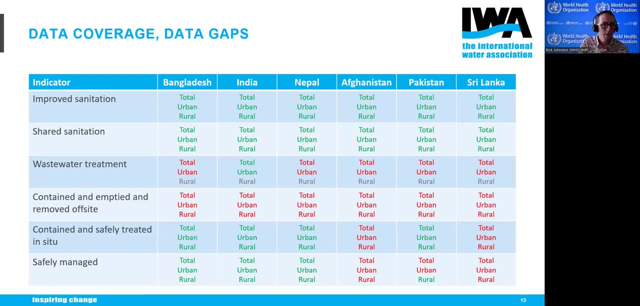 So improved and shared sanitation. full data available For wastewater treatment for the sewer population. only India were we able to find nationally representative data about wastewater treatment from centralized wastewater treatment plants. I've grayed out rural because the rural coverage is so low with sewer, but still it would be nice if nationally representative data. 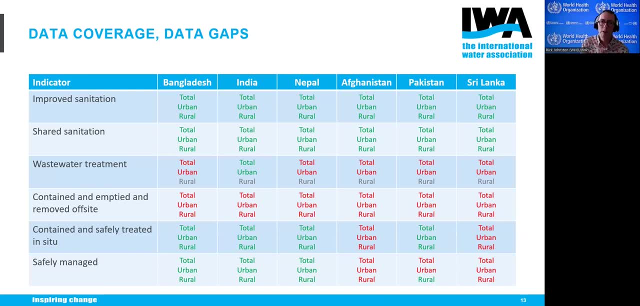 were available for the other countries. even though sewer coverage is not very high in urban areas, still it's growing And, as we saw in Pakistan, it's already quite high. Then the next two rungs about whether onsite sanitation facilities are contained and either emptied and 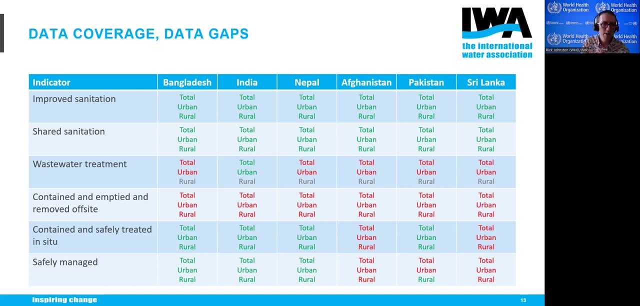 removed offsite or safely treated in situ. we see that in none of the countries do we have nationally representative data on what happens when these septic tanks, these pit latrines, are emptied and taken offsite. We have a lot of nice examples of a few municipalities. 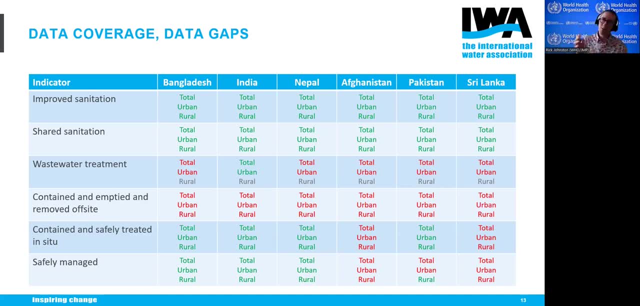 a few FSTPs that are either working really well or maybe aren't really working well, but we haven't found a national picture yet for any of these six countries, So hopefully in the future that data gap could be filled. Whereas safely treated in situ, we do have. 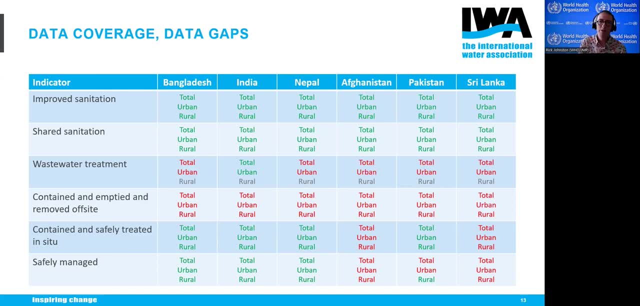 examples of countries collecting nationally representative data through household surveys, such as the multiple indicator data. We have a lot of examples of countries collecting nationally representative data through household surveys, such as the multiple indicator cluster surveys, the MIX, that have been fielded in Bangladesh and Nepal and Pakistan, or in other national surveys. 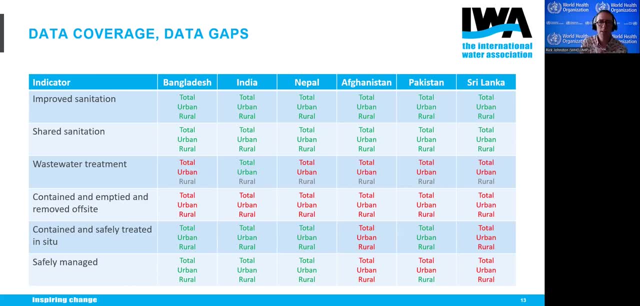 like the Indian National Sample Survey or the Bangladesh National Hygiene Survey- both of those from 2018, that collect data on containment and emptying and what happens when these systems are emptied. So the bottom line, then, is that safely managed sanitation data were only available for. 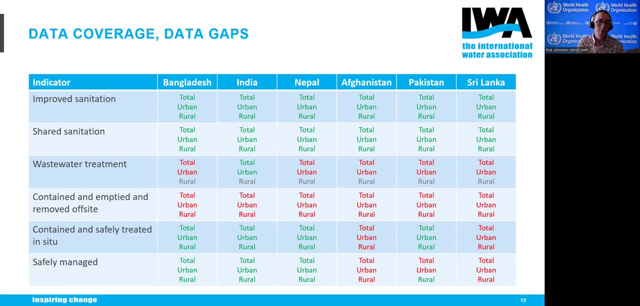 the countries basically that had data on treatment in situ and that's because that's the dominant form of sanitation used by people in those countries. That's why, for Pakistan, we don't have safely managed sanitation, because most people are using sewer connections and we haven't found national data on wastewater treatment. 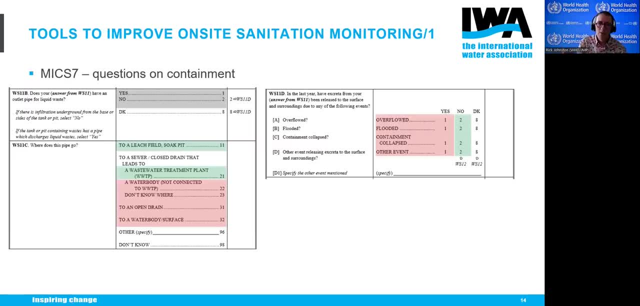 Okay, so how to fill these gaps? Household surveys are one tool- It's not the only tool, but it's one tool- And I mentioned the MIX surveys. They now contain three questions about containment: How to fill these gaps? Household surveys are one tool- It's not the only tool, but it's one tool- and I mentioned the MIX surveys. They now contain three questions about containment. How to fill these gaps. Household surveys are one tool and I mentioned the MIX surveys. They now contain three questions about containment. How to fill these gaps. Household surveys are one tool and I mentioned the MIX surveys. They now contain three questions about containment. 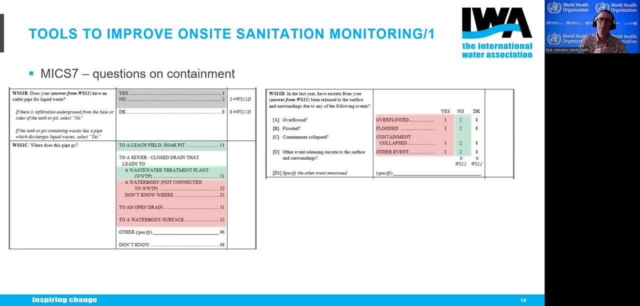 What does your septic tank does your pit latrine? does it have an outlet pipe? What does that connect to? Has your septic tank or pit latrine overflowed or flooded or collapsed during the last year? So those kinds of data can tell us if the systems are effectively containing wastes. 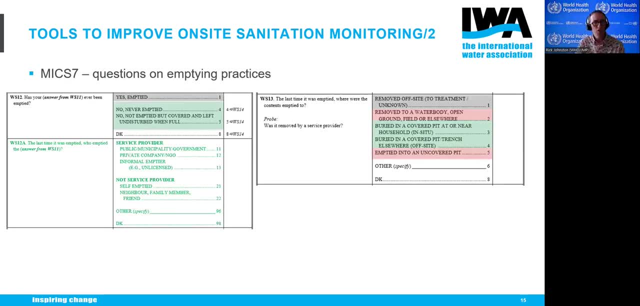 Then there are also questions about emptying practices, some of which are leading towards safe management and some are not. So if people say that they've never emptied it, that can count as safely managed. safely managed If they've emptied it and then they've buried it nearby in a covered pit or a. 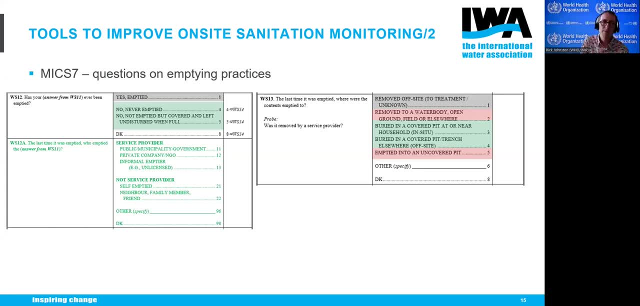 covered trench, that can also count as safe management. If they say it was emptied but then it was discharged into an uncovered pit or a water body, clearly that's not safely managed sanitation. If they say it was emptied and removed off-site, it could be safely managed. but you 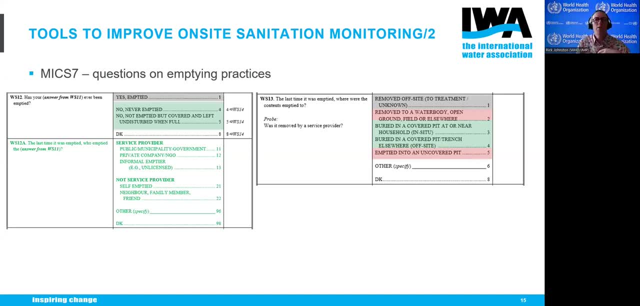 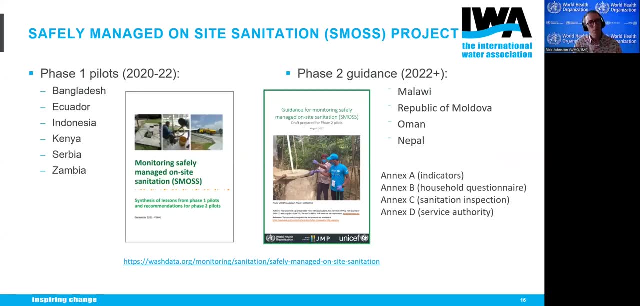 don't know, Then you would need to have additional information about, you know, the trucks and the treatment plants that the households aren't in a position to give, So you would have to combine that with other data. So we've had a project for the last four years now called Safely Managed. 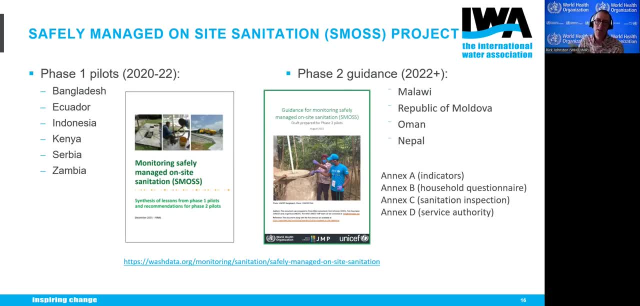 On-Site Sanitation that tries to look at all these steps of the sanitation and what type of sanitation chain and what types of data could be used to plug gaps along the way. looking at containment, emptying, transport, treatment and disposal. We finished a phase one set of pilot. 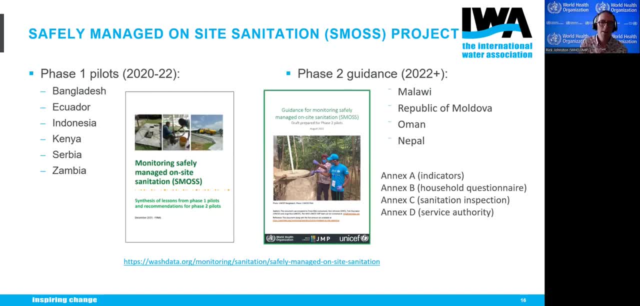 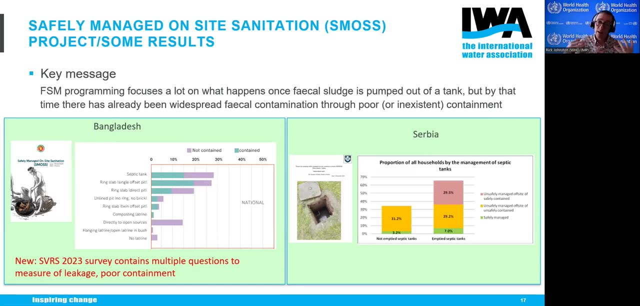 countries, including Bangladesh, And are now working in a set of phase two pilots, including Nepal. So this region is definitely well represented in our SMOS project And there are a number of resources available on the website that you can see there. Just some key findings from the SMOS project are that there's a lot of 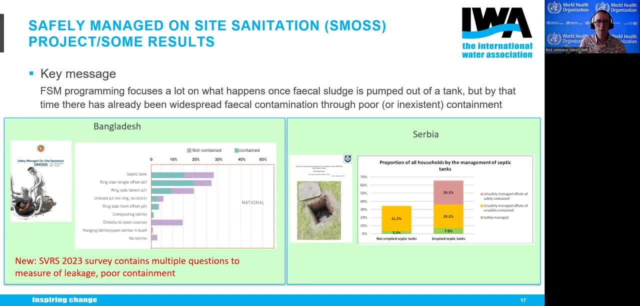 FSM programming around what happens when the trucks come and they empty the containment, Where do they go And what kind of treatment happens And what about the sludge. But there's less focus on what happens before the trucks come. You know, is that containment? 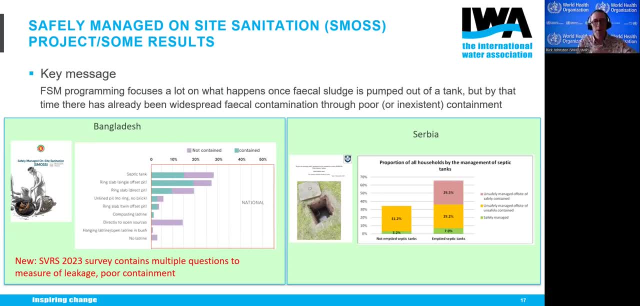 Is that really containing waste Or does it really have an open pipe that's leading to an open drain, Because you can have the best FSM in the world? but if that tank has been discharging untreated waste into the environment before the truck comes, you know it's a hazard and it's 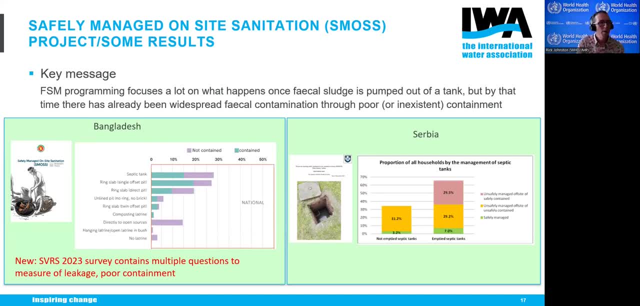 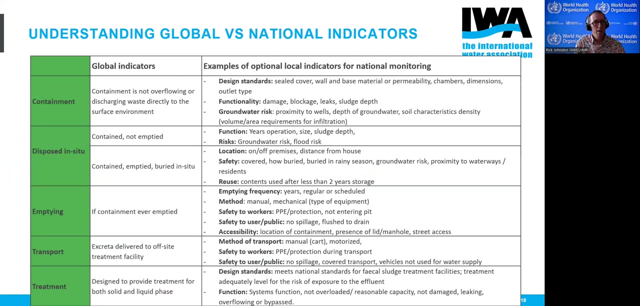 certainly not. safety managed sanitation, And both in Bangladesh and Serbia, inspections of the facilities found that many of them were not safely containing wastes. In Bangladesh, and also new questions about containment and leakage in a new big national survey that should give additional information about containment in that country. I think I'm 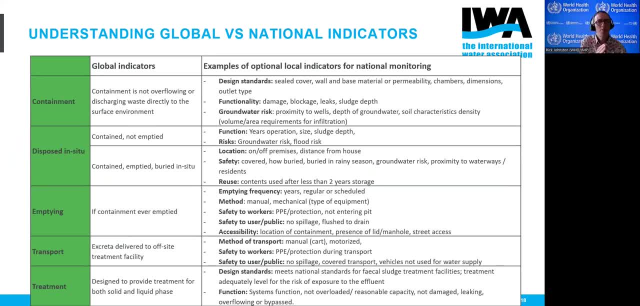 going to skip the details here, but just to note that, through the SMOS pilots, we found that it's important to distinguish between the global indicators, which are relatively simple and few, and the local indicators, which are necessary for national monitoring purposes and local monitoring. 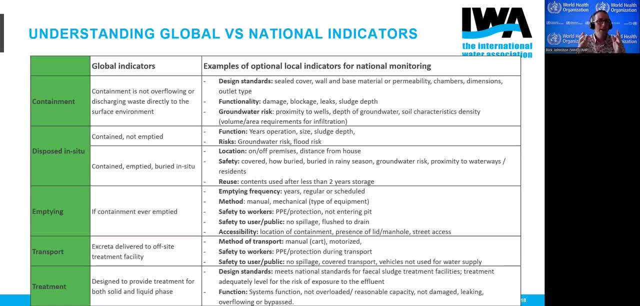 So thank you. So things like groundwater risk, safety to workers, PPE, numbers of years of operation, the size of the tank, that's all really important national information. None of that is necessary for safety, managed sanitation at a global level And in fact the global systems couldn't possibly. 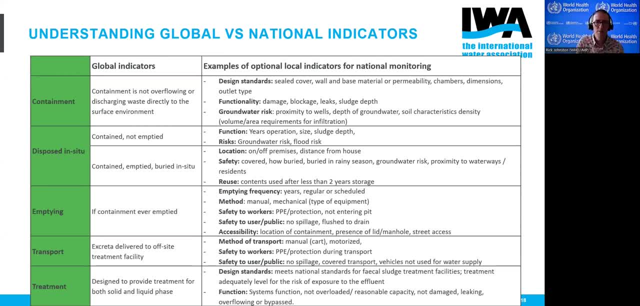 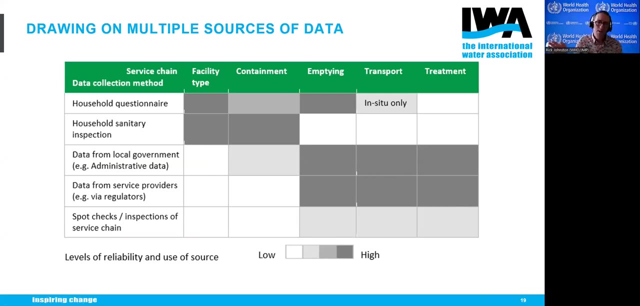 accommodate that much detail because each country will have its own different systems. So that was a key finding of the pilot- was to understand Which bits are necessary for global and which bits are necessary for local. Another key finding is that we need data along the entire sanitation chain, from the type of facility. 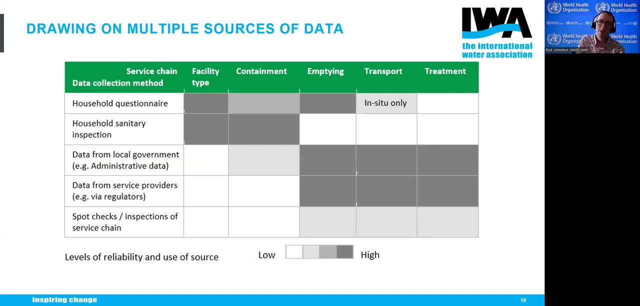 to the emptying, treatment and transport. but different data sources can serve for those different stages And when you're closer to the facility and the containment, the data are more reliable if they really come from households themselves through a questionnaire or some kind of inspection by someone coming to visit. 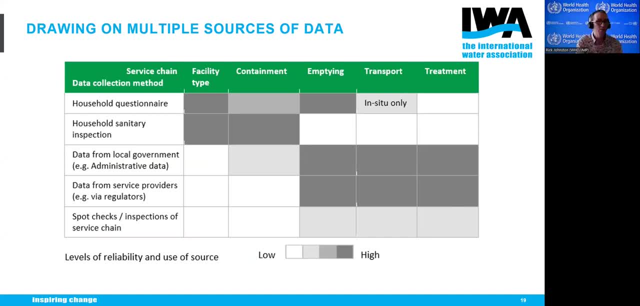 More than from regulators or administrative data. But once the waste leave the household and we get into emptying, transport and treatment, the household doesn't know what's happening there, And the better sources of data are coming from administrative sources or regulators, So the trick is to be able to combine those to make one coherent story on sanitation inspections. 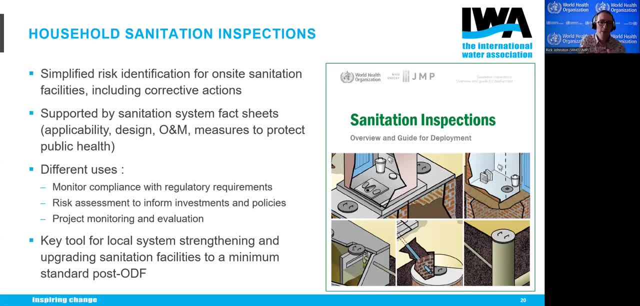 The W H O And the J M P Have been working together to come up with these simple checklist to visit sanitation facilities and see: are there risks, Are there corrective actions that could be taken. There's been a lot of experience with this in water infrastructure. 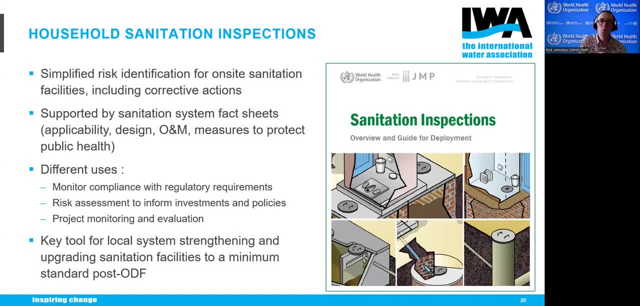 and now we're looking at developing similar tools for assessing sanitation infrastructure, And those could be used to monitor compliance with regulatory requirements or to perform risk assessments or to track progress in a project, And we see these as a key tool for local authorities to use to strengthen and upgrade sanitation facilities, For instance, in an ODF program. 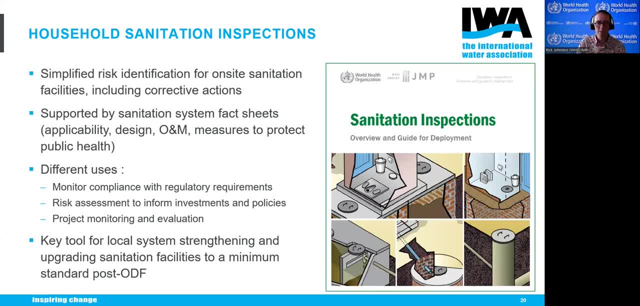 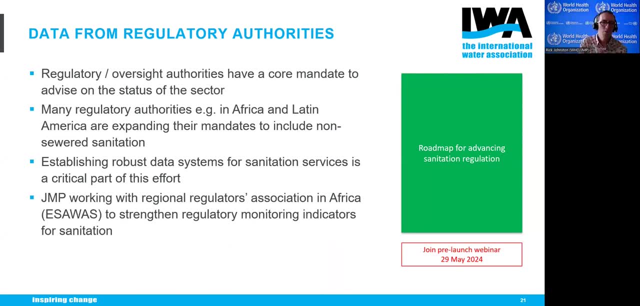 to monitor against slippage and to look at higher levels of service. And finally, we see that regulatory authorities are a key tool or a stakeholder to collect this type of information, either directly collecting it themselves or harvesting it from other partners They have. 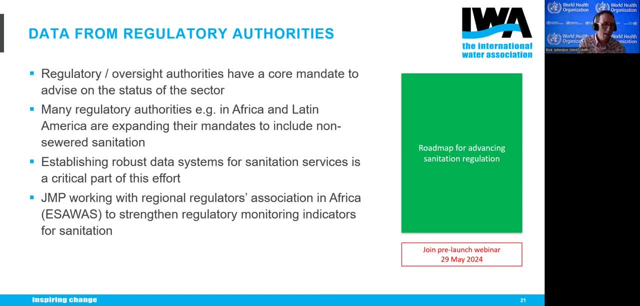 the mandate to advise on the status of the sector. The mandate in many cases includes not just the status of the sector but also the status of the sector, And so in many cases just sewer connections but also non-sewered sanitation, And we do see many regulatory 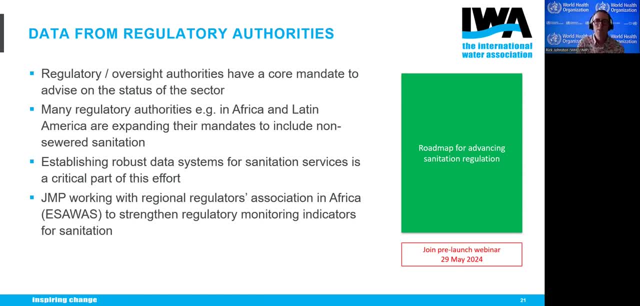 authorities are expanding their work to explicitly cover non-sewered sanitation as well, And that creates new data challenges. I know we're going to hear from Nepal about NWASH and the ambition there to build a national MIS that includes the sanitation services, but also in Bangladesh. 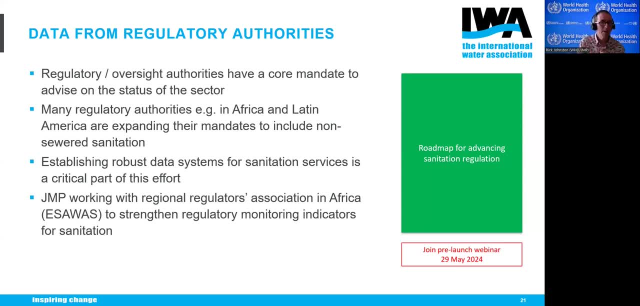 and India. I know you have really advanced database systems, So I'm looking forward to hearing those experiences. Just wanted to mention that globally, we do engage with regulators around the world and also with regional networks of regulators. There's a very strong one in Africa called Esawas And I think there could be some value or interest in maybe. 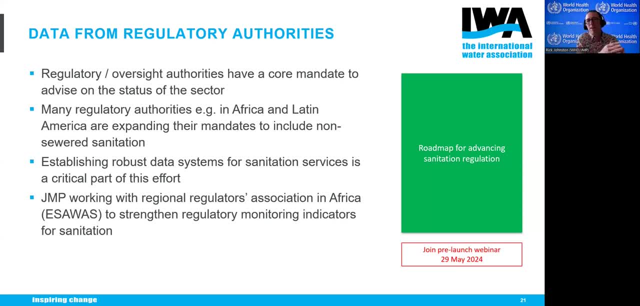 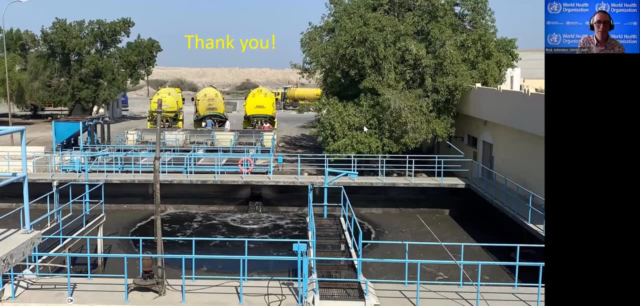 establishing such types of networks in South Asia or East Asia, where there's a lot of interesting work happening. So with that I thank you And I turn back to the moderator, I think, for the next presentation. Thanks, Rick, very much for an amazing overview of all the activities that have been done by WHO in. 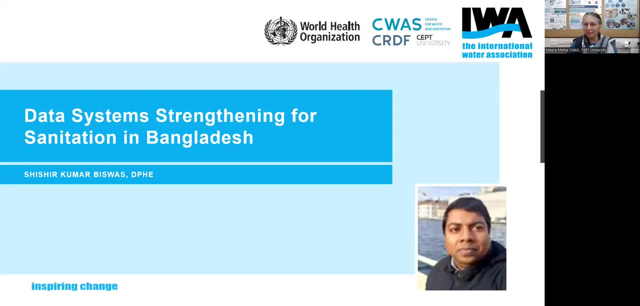 improving the whole monitoring system, And I think your reference at the end to looking at national data systems is certainly something that actually, hopefully, will be highlighted by our next set of speakers. So thank you very much, Rick. I'm not sure about regulators in this region, but maybe it will come up in the discussions during the 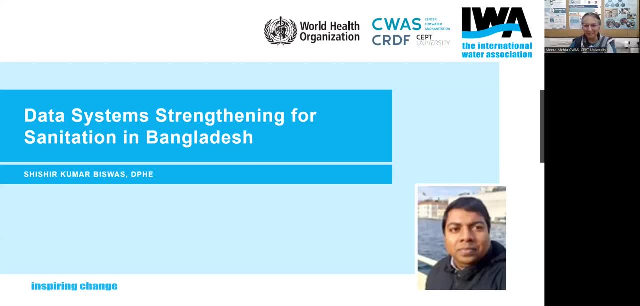 presentations and after that, Certainly in Africa it is relevant, but we'll have to see what kind of system do we need for South Asia? So thanks, Rick Again. I would now like to invite Dr Shishir Biswas. He's an executive engineer with the Department of Public Health Engineering. 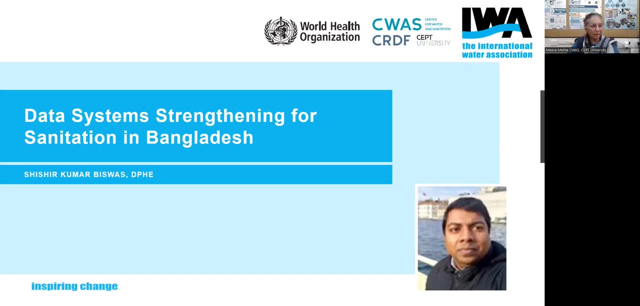 He's been involved in establishing establishment of web based sanitation and waste management dashboard of for 61 district towns and integrated management of what is known as IMI's- that system in Bangladesh. He, so he's really has the kind of experience that we were talking about. that is needed for. 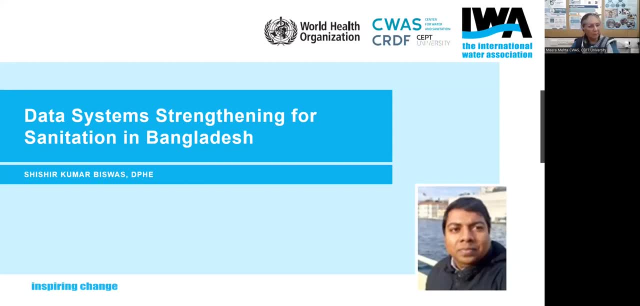 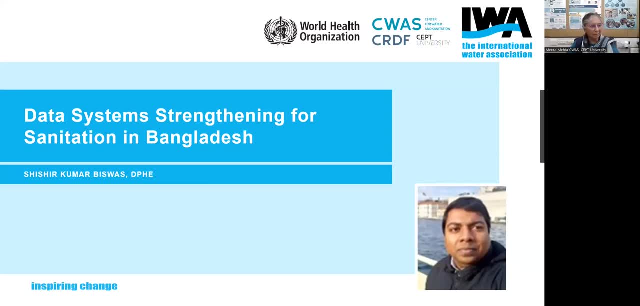 BWET, and he has impressive background in terms of civil engineering and Master's degree in that. So let me invite Shishir to make his presentation on Bangladesh. Thank you very much. moderator. This is Shishir Kumari-Bishwas, Executive Engineer, Department of Public Health and. 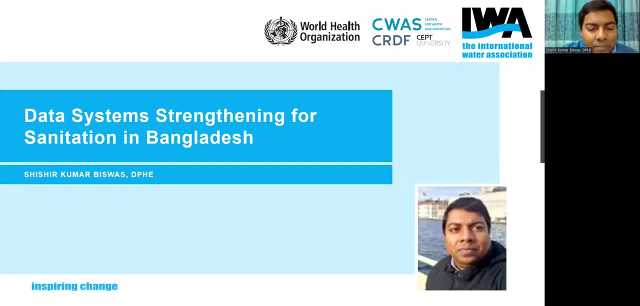 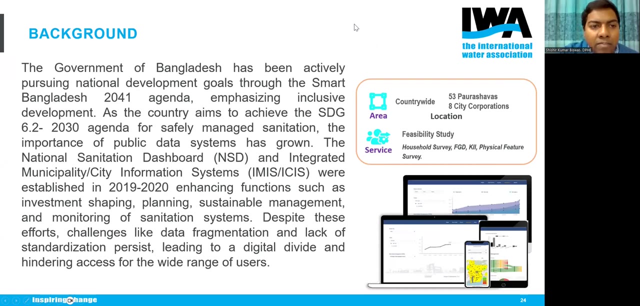 Ochiblog: health engineering. Now. thank you very much for inviting me for sharing my experience on data system strengthening for sanitation in Bangladesh. So the government of Bangladesh has been actively pursuing for national development goals through the Smart Bangladesh 2041, as in the emphasizing inclusive development as the country aims to achieve. 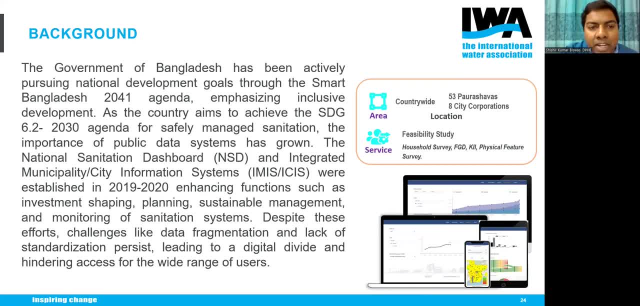 the SDG 6.2 in 2030,, as in the for safely managed sanitation, the importance of public data system has grown. The National Sanitation Dashboard, as I mentioned, and the integrated municipalities and city corporations system information were established in 2019 and 2020,. 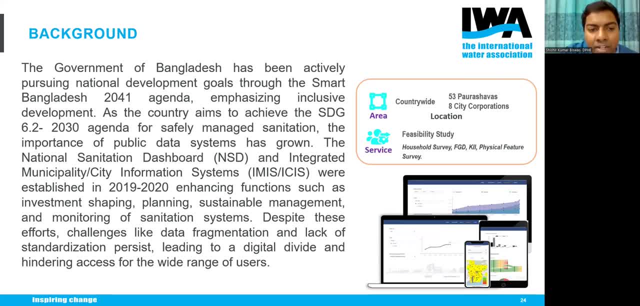 enhancing functions such as investment shaping, planning, sustainable management and monitoring of sanitation. Despite this efforts, challenges like data fragmentation and lack of standardization persist, leading to a digital divide and hindering access to wide range of users And the right side- some picture is here We have, I mean, under DPHG, we have conducted 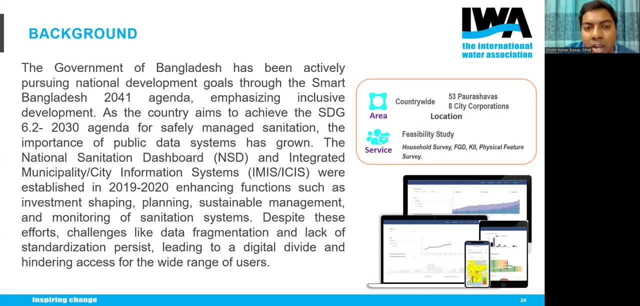 a comprehensive standardization. We have a survey for extracting sanitation data specifically for a faecal sludge management system and municipal solid waste management system in 53 district towns, municipalities in Bangladesh and eight city corporations. Most of the people I mean Abrahan people. 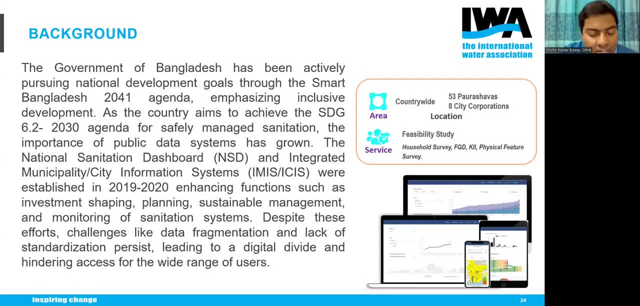 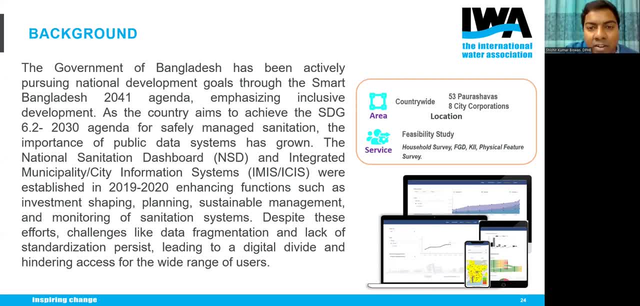 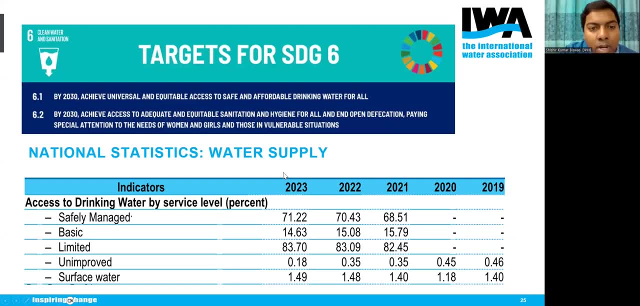 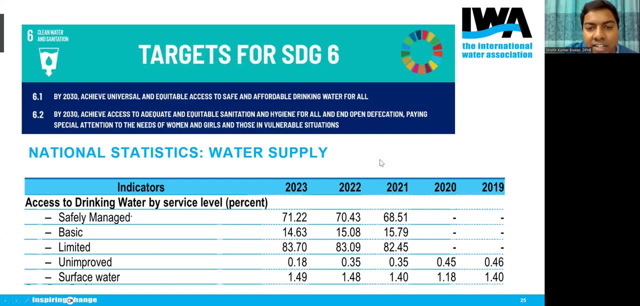 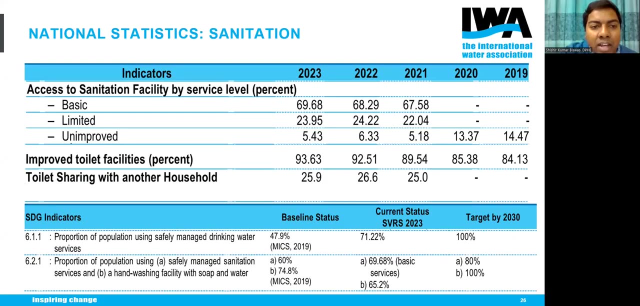 by Bangladesh Bureau of Statistics Our census just completed in 2021.. According to the census, there is the water supply statistics: the safely managed water supply system in 2023 is at about 71.22%. And if you consider the sanitation system, apart from the safely managed sanitation system, 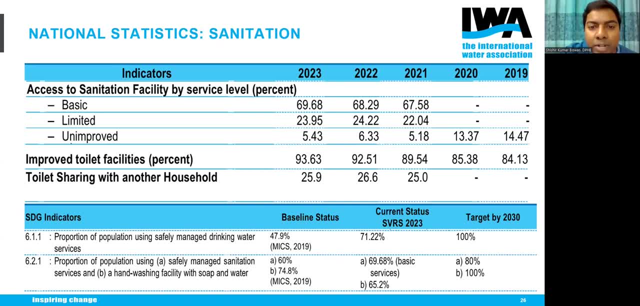 we have the basic sanitation: 69.68, limited 23.95, unimproved 5.43.. But what? I'm telling that, apart from the safely managed sanitation, because still now we are really working on the shared latrine though- 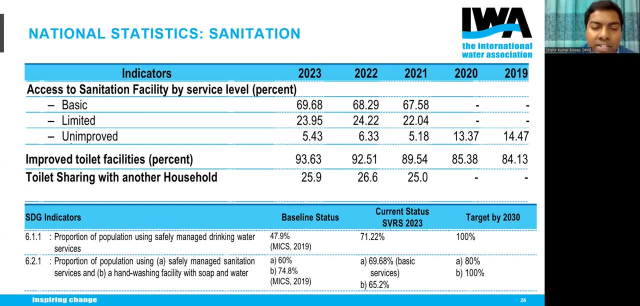 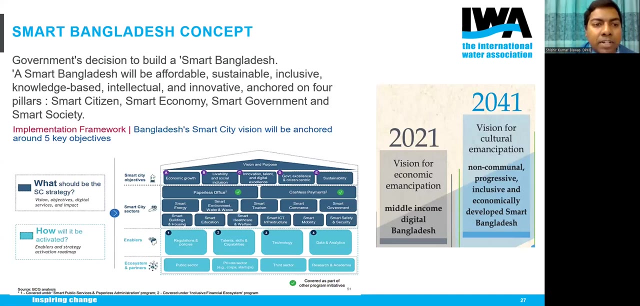 those are really improved And we have provided different facilities under different projects. That is 25.9%, But according to the GMP report, the safely managed sanitation in Bangladesh is only 39%, So there is still a gap. So now the Bangladesh government has introduced the concept. 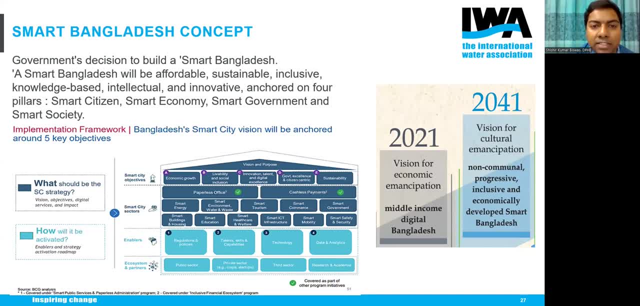 that is smart Bangladesh. A smart Bangladesh will be affordable, sustainable, inclusive, knowledge-based, intellectual and innovative, anchored for four pillars: smart citizen, smart economy, smart government and smart society- Previously the vision for economic emancipation and now the target for reaching in 2041, the cultural emancipation: non-communal, progressive 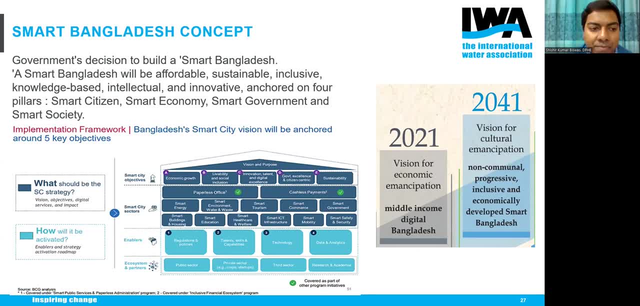 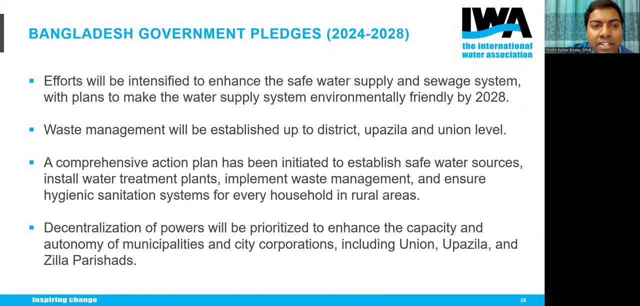 inclusive and economically developed, smart Bangladesh. Now, where is the future for the population? A new perspective in the case of the. from the beginning of the pandemic a year ago in the arenas, the community went to the main construction sites and also the HCBS building and frontage and construction sites. 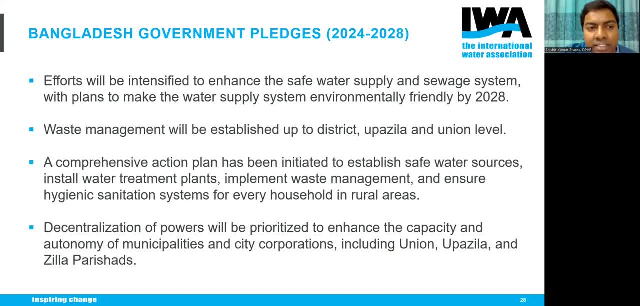 intensify to enhance the safe water supply in swiss system, with plans to make the water supply system environmentally friendly by 2028. waste management will be established up to district, to pojola and union level. one thing i need to mention: that in balance. you know that. 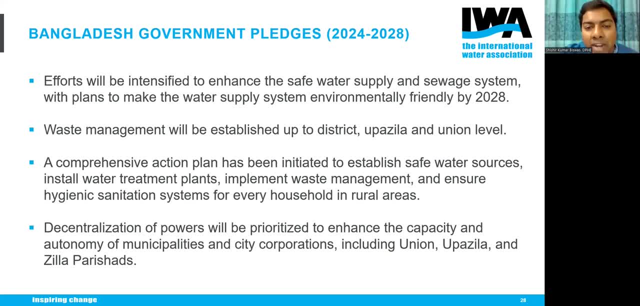 the very small country. land is really scarce here, so separately providing facilities for sanitation- only non-sweat sanitation system, also a central sewer system, is very difficult. that's why our government is thinking for integrated development activities, considering the municipal solid waste management and also the fecasas management system for both urban. 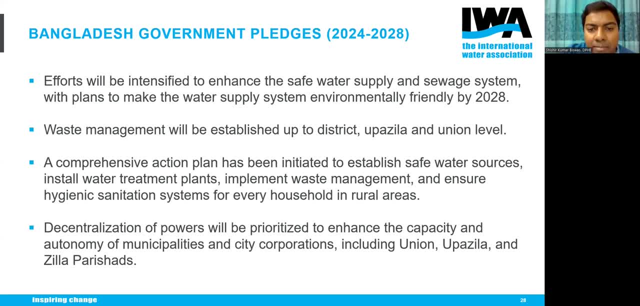 peri-urban and rural areas. the comprehensive action plan has been initiated to establish safe water resources, tall water treatment plants, implement waste management and ensure hygiene, sanitation system for every household in rural areas and decentralization of the powers, actually the delegations of powers of local government. 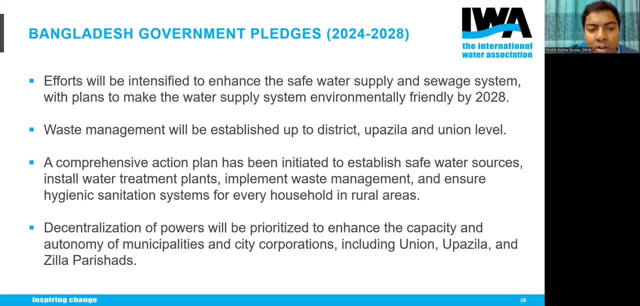 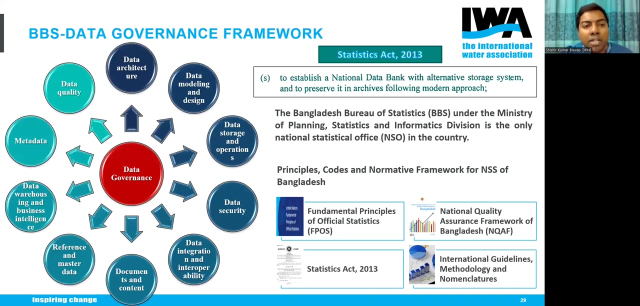 institutions, uh specifically our city corporations, municipalities, uh union level and upojala level and jila level. those are very, very much important. otherwise the accountability, transparency of data and sensitive and standardised information will not be given in the system as in the real time development activities for all will not be possible. that is also very important for bangladesh. 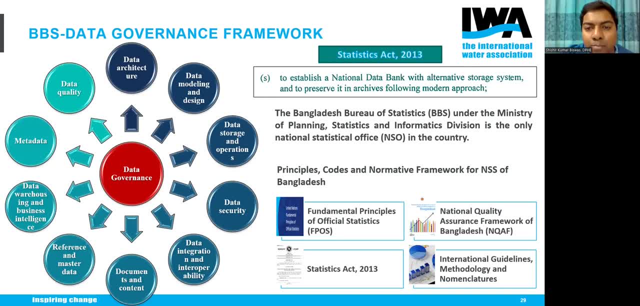 government, so now agreeing to the statistics act 2013. our bangladesh bureau of statistics is the only national statistical office in the country. they actually collect data: uh census data, data of different segments, different attributes and also, as I have mentioned, that for water. 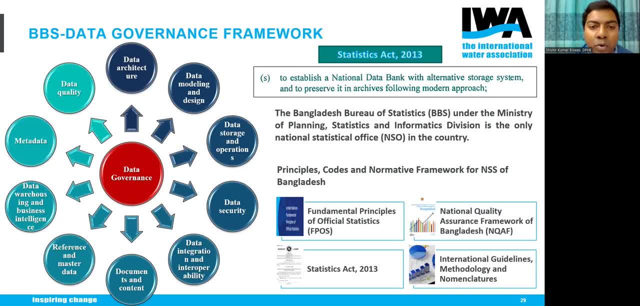 supply, sanitation, urban, rural, peri-urban, all of those. But you know that it is not really possible for only Bangladesh Bureau of Statistics to collect data only by themselves. They share data from different other organizations and Department of Public Health Engineering, since once throughout the country for providing the services of water supply. 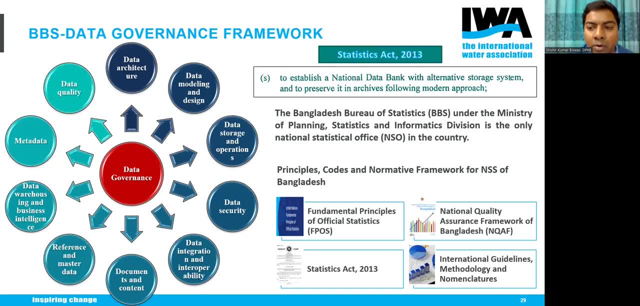 sanitation waste management drainage system. we share our basic data, collected data every year. we are collecting through different project activities and also from our revenue activities. We share those data to our Bangladesh Bureau of Statistics and they really update their data every year. 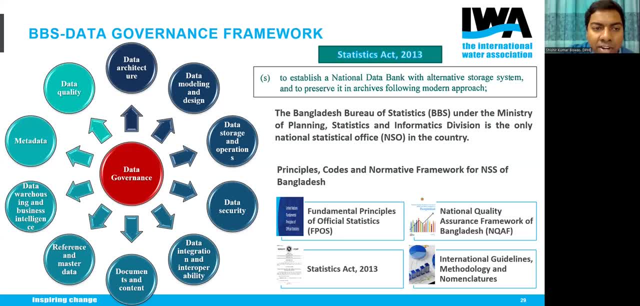 So data Governance framework they have established very, very much important, because only data, any types of data collection, is not at all to present and represent any specific services. that can be said that yes, it is the national database. It is not possible. So screening and under a framework screening, and that is also very, very 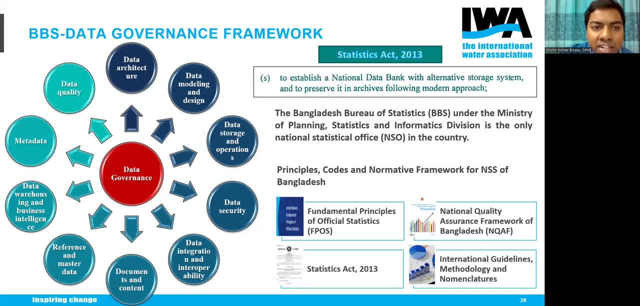 much important. We have the Data structures, data architectures, data modeling and design, data storage and operational data security, data integration and interoperability. All of those are really integrated. on this data governance, We have other regulations and frameworks: how to execute, how to utilize this and sharing and. 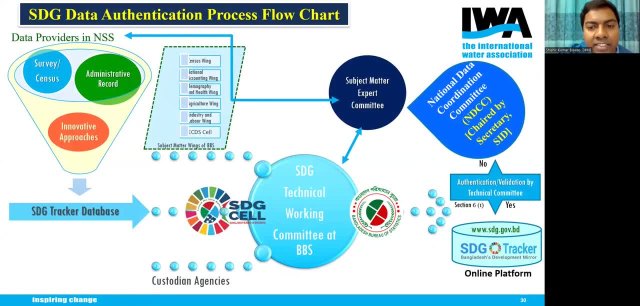 utilizing two different government agencies and non-governmental agencies. So here is a flow diagram. you know that we are also looking for achieving the goals of sustainable development goals, So our Bangladesh Bureau of Statistics actually follows a process: the survey, census, administrative records and innovative approach. 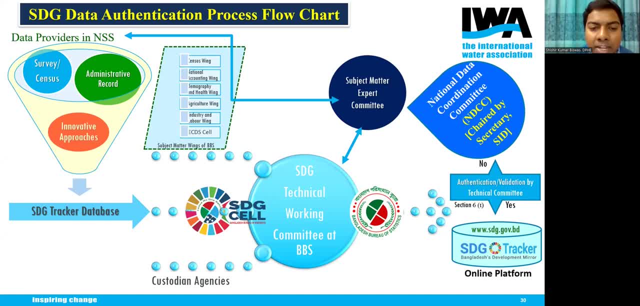 Absolutely, And they provide those data. Now we have the access to information and some other divisions Monitoring and controlling by our prime minister's office. We have the SDG cells. So after their technical support, their screening and validation, those goes to our online. 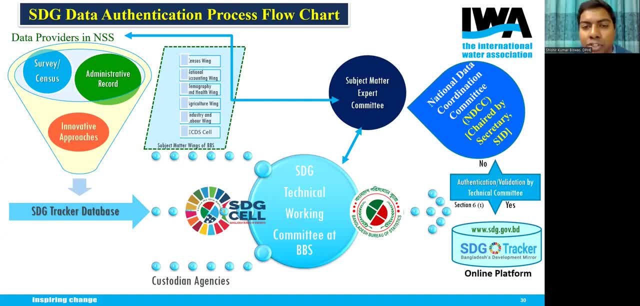 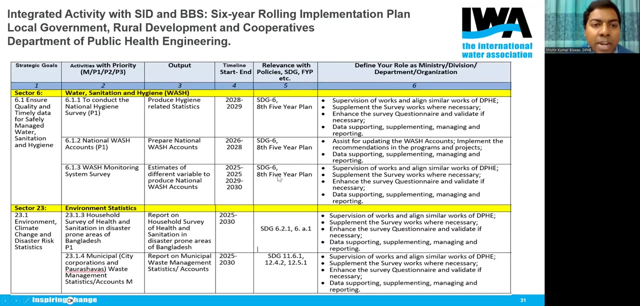 platform, that is, the SDG tracker, And those are also shared to the respective agencies. I'll share it as some slides who are actually getting those information and sharing their respective information To These specific sector? I mean what sector? So, as I mentioned, that the mainly controlled by our SDG affairs under prime minister's office. 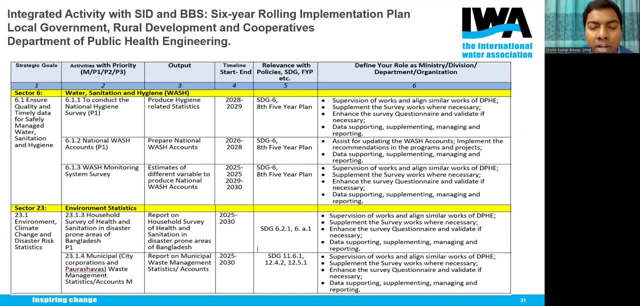 So Department of Public Health, Engineering and some other losses and city corporations have received some specific designated activities, some assignments for achieving the goals of six point one point one, six point one point two, And also supporting with the wash that Those are some environmental statistics, household survey of health, sanitation in disaster prone areas in Bangladesh and municipalities. 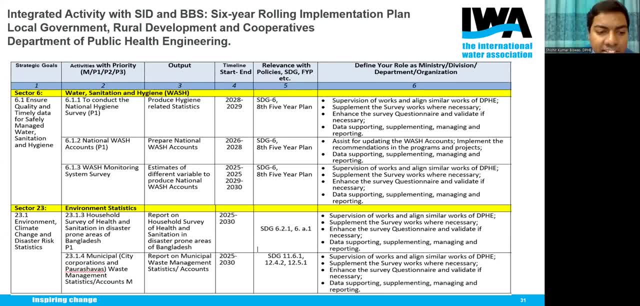 And both of us- I mean municipalities and city corporations- waste management and sanitation get us. We have to collect those specific information Under a very specific question here, with using different tools and innovative ideas from rural levels, urban levels, municipalities and city corporations. 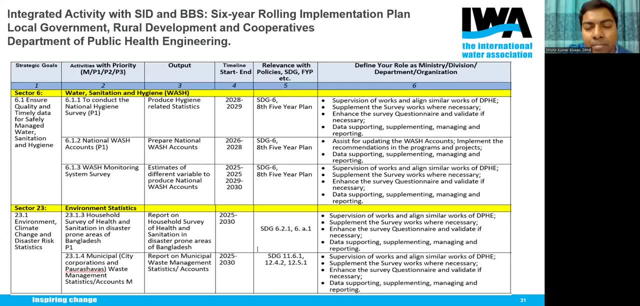 And preserve it to our DPHE platform. you know that we have already established a citywide inclusive sanitation cells. We have integrated server and the connection with that server to our DPHE platform. So we have integrated server and the connection with that server to our DPHE platform. 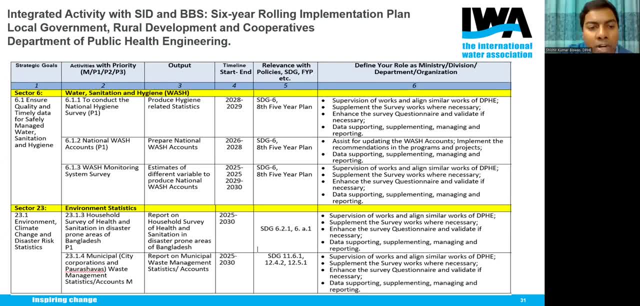 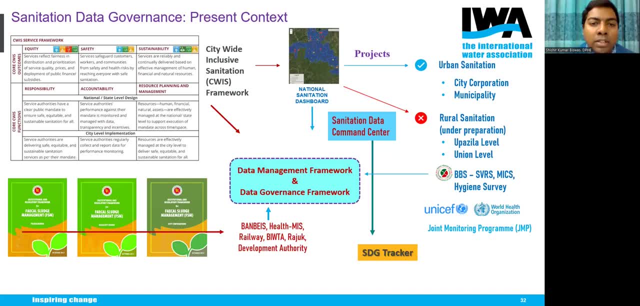 So we have integrated server and the connection with that server to our DPHE platform. We have integrated server and the connection with that server to our duplex which is across Bangladesh group statistics For screening and level of activities. So again I am going to 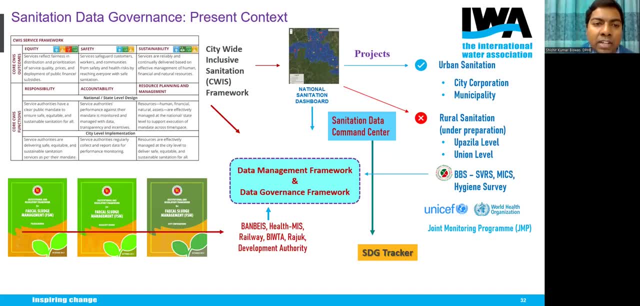 The feasibility studies we have completed And based on The criteria of citywide inclusive sanitation, We have our framework, different frameworks and also implementation plan, selecting different criteria and Our indicators or series: A comprehensive Study, Handling and monitoring 154: 00.. 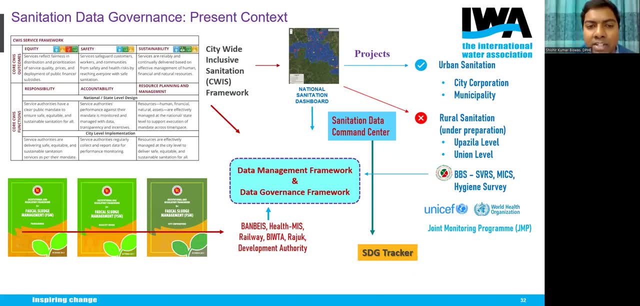 had been conducted during 2019-2020 and up to June 2021, and accumulated all of those data in our open source website, that is SANBOARD- S-A-N-B-O-A-R-D, So anybody in any other country can easily access the information of the SANBOARD. what types of data actually we have accumulated in? 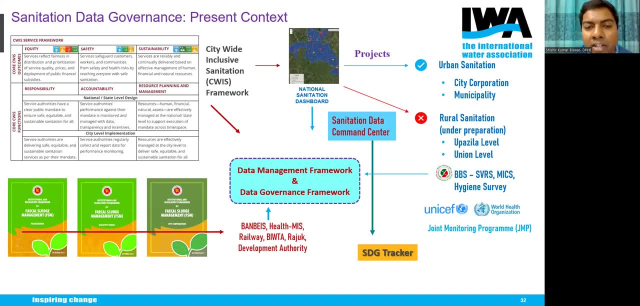 it. Sheet flow diagram also and the flow pattern of sheets from the containment system, from generation, till the disposal systems with the Schencky diagram can easily be identified, including the percentage, the values of every components of this value chain. But we are in quite lagged behind in rural sanitation system since the Bangladesh Borob. 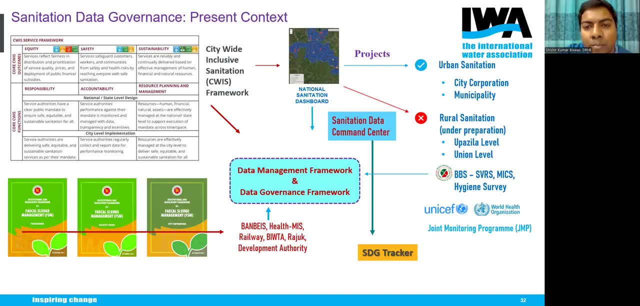 Spree statistics collects through census data, the rural information. but we are now trying to establish a framework and also a master plan for rural sanitation. also, and hopefully the regular data collection will be started from our rural and will also be included to our 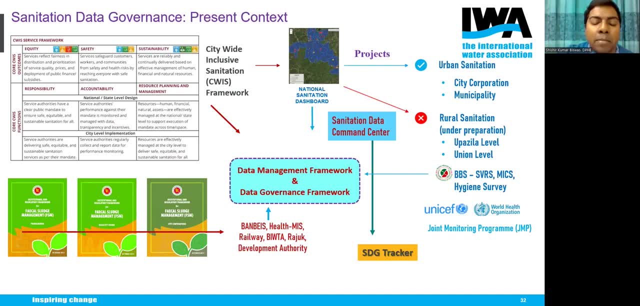 national sanitation dashboard. In the meantime, we have assigned some MOU with GWSC and our plan to establish a data management framework. data governance framework and basic concept of data commanding center we have established in DPHE and they have also started their work under. 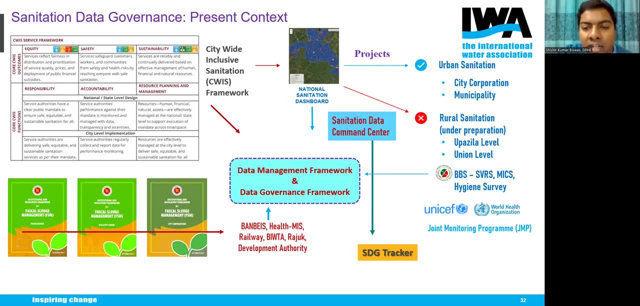 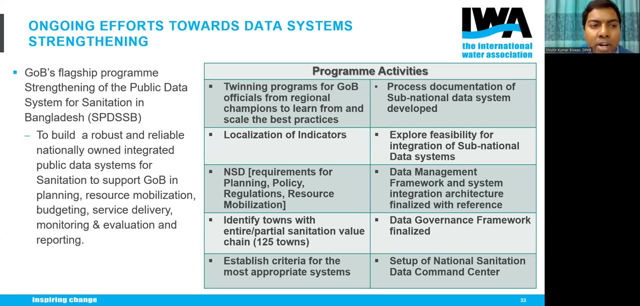 the support of Bangladesh government and the BNGF. So ongoing efforts towards our data system strengthening government flagship program, the strengthening of the public data system for sanitation in Bangladesh to build a robust and reliable national. If you can now wind up in a couple of minutes, please. 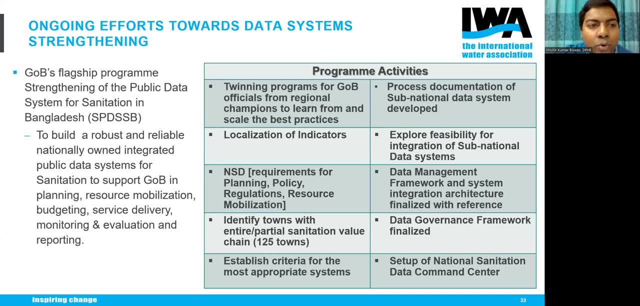 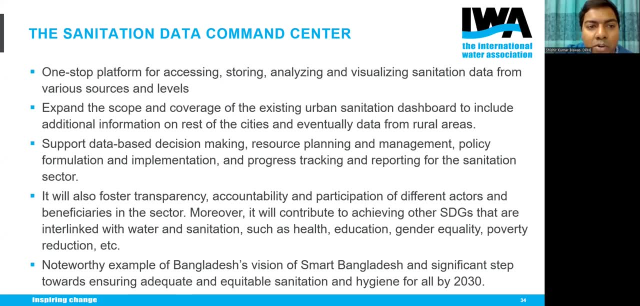 Okay, I'm going first. So after this, we have established this data command center. This is a one-stop platform for data management. So after this, we have established this data command center. This is a one-stop platform for accessing, sorting, analyzing and visualizing sanitation data from a various source. 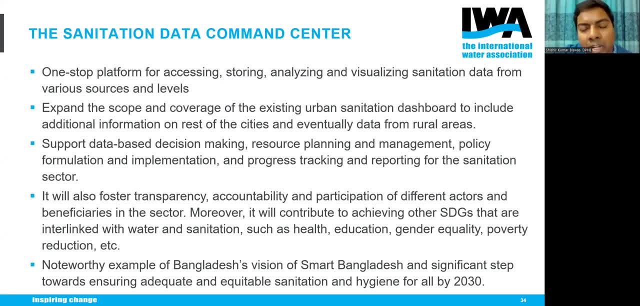 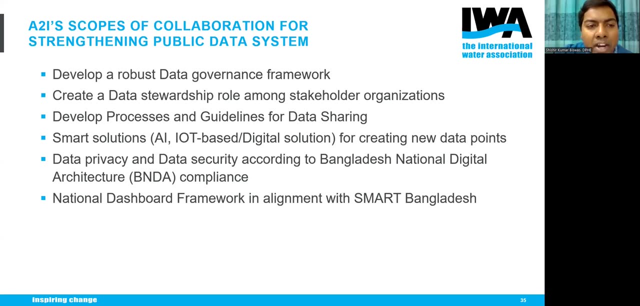 system of level. We have some time-bound assignment and hopefully this data, what we are actually collecting, will be standardized and validated. So access to information, also working hard and supporting us, since they under Prime Minister's office and related to this data, but also 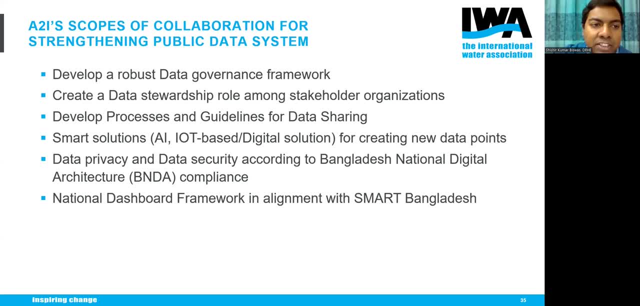 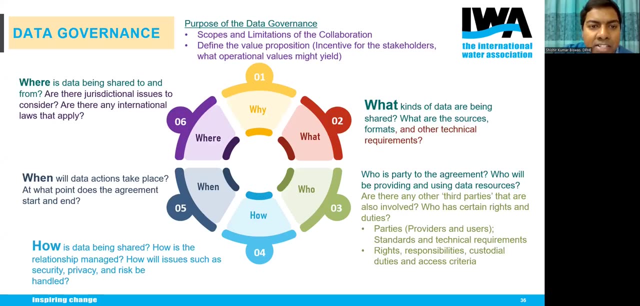 to provide the information to our SDG trackers so they develop a robust data governance framework and create a data stewardship role among stakeholder organizations. So here is the concept of the data governance. I'm not going in detail. So the other organizations? 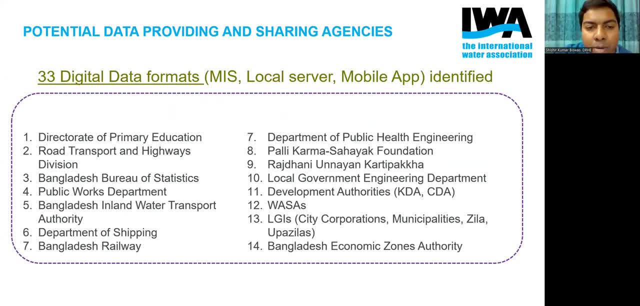 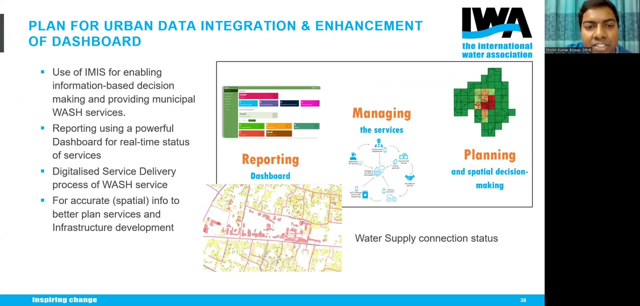 which I have mentioned, the Directorate of Primary Education. we are providing support to our primary education, All the primary schools. we are providing wash facilities, road transport, highway divisions. Bangladesh Bureau of Statistics, Public Sports Department, Department of Shipping- some other organizations are like this. 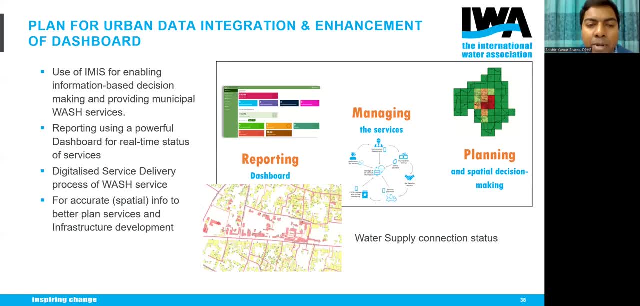 IMIS has already been introduced and in every urban project we are introducing this IMIS system, not only for the sanitation but also for water supply. So all the information, the holistic information, we are actually collecting and accumulating in our server and, chronologically and under a standardized system, We are preserving, and all the other. 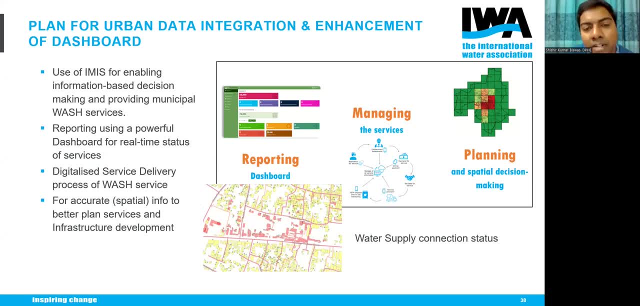 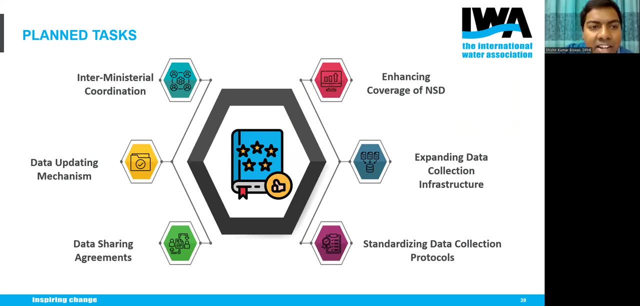 information, including our business model data collection system, and, you can say that, providing the service and tariff collection systems all are utilizing under this IMIS platform. So, apart from this, some plant tasks that are: inter-ministerial coordination, enhancing coverage of national sanitation dashboard, expanding the 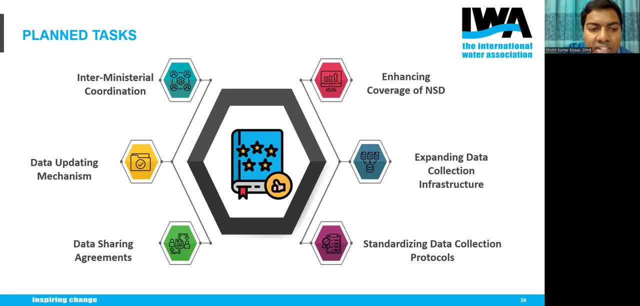 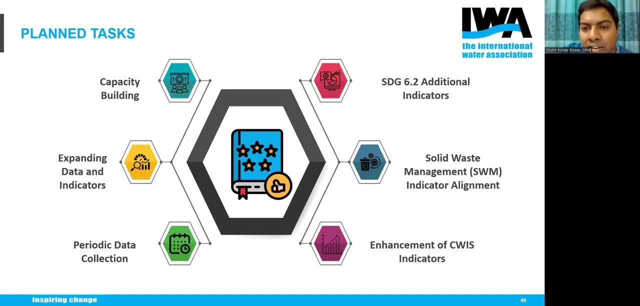 data collection infrastructure, standardizing the data collection protocols, data sharing agreements and data updating mechanism. SDG 6.2, some other sub-indicators. you know that I have already said that we have provided improved shared Latin, but it is not actually counted in. 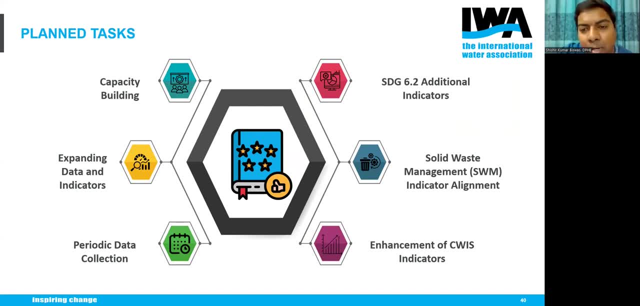 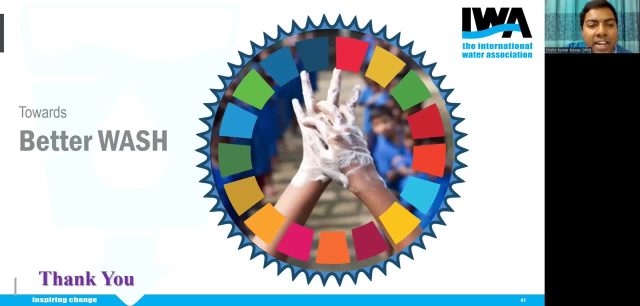 our SEPA sanitation system. so some other indicators. we are thinking about Solid waste management system and enhancing city inclusive sanitation system, some other. so thank you very much from my side. Thank you, Mr Bishwas, for a very engaging presentation and the kind of complexities. 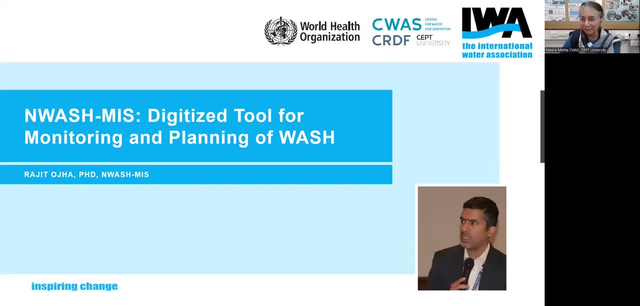 that are involved when you work at the national level and relating to the plans, the kind of different data systems that are there. So I think it was very good in terms of highlighting these issues. May I now invite Dr Roja from Nepal? 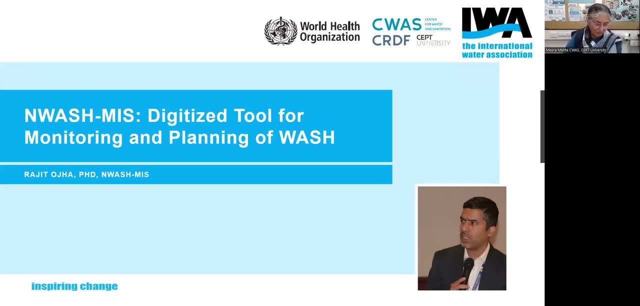 Dr Roja is the Chief of NWASH and Institutional Support and Service Advisory Support in the Department of Water Supply and Sewerage Department in Government of Nepal And I think from my earlier meeting with him, which were only online, that he is very conversant. 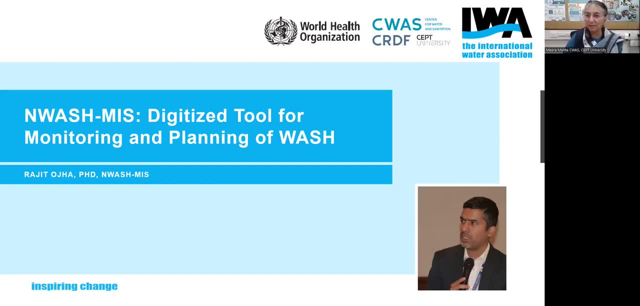 with the kind of activities that are going on in wash sector in Nepal and has been, I think, taking a leadership role in terms of setting up, monitoring and monitoring of water systems, which are extremely essential to improve over time. So that's something that we are really looking forward to. 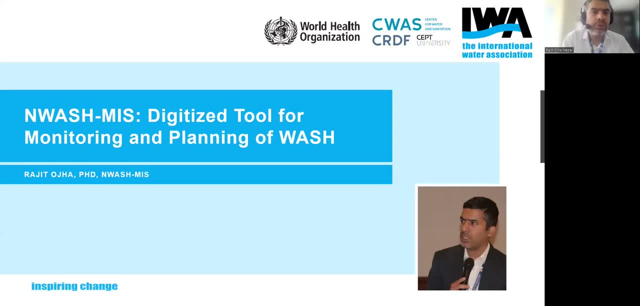 Over to Rajit. Hi Namaste and good afternoon everyone. I'm Rajit Roja from Nepal. Thank you for the opportunity for the presentation Today. I'm going to present about National WASH MIS, which not only covers sanitation. 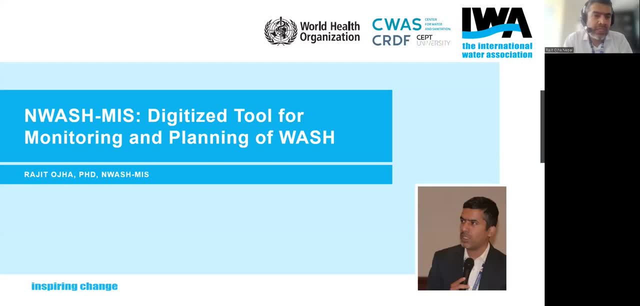 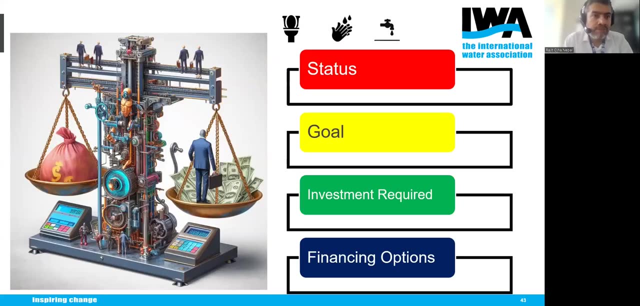 but also covers water supply and hygiene as well. It is a digitized tool for monitoring and planning also. So idea of NWASH, The idea of our development of MIS, was to support the local governments for the planning of SDGs 6.1 and 6.2.. 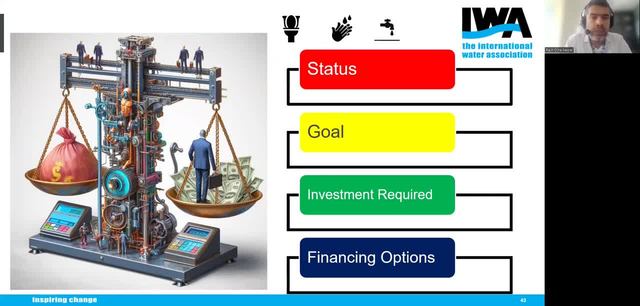 So, along with the monitoring of all those indicators which we can see in terms of status, we have let the local government know about what is their goal in terms of SDGs and what is the investment requirement. This is the back end calculation that we have supported them in doing and what can be the 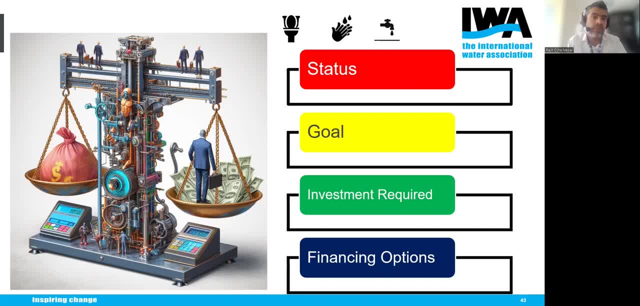 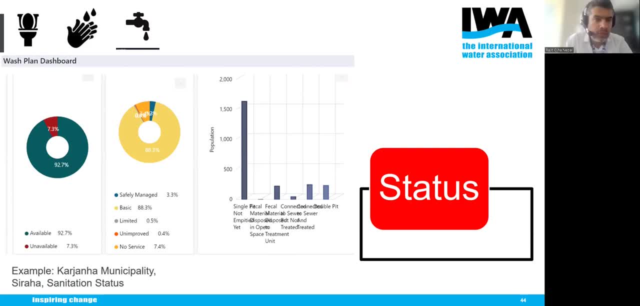 financial options. They can also discuss the financial option inside the overall management information system. So this is one of the examples of how we are collecting the status. This is one of the examples from Karzana, one of the municipalities of Nepal, where 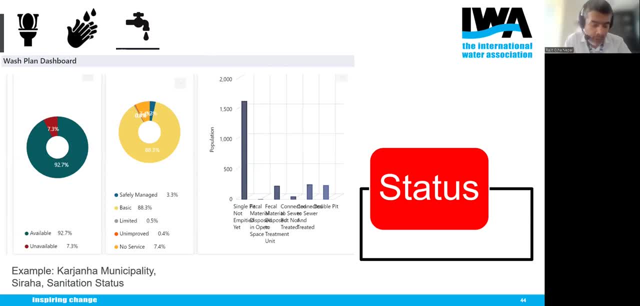 you can see the overall status in terms of JMP ladders. Mostly, we have adapted the JMP indicators. We are also fortunate to get the JMP support in terms of improvement of these indicators and we are also doing a few improvements, Thank you. And these indicators now and then and the discussion on improvement of those indicators. 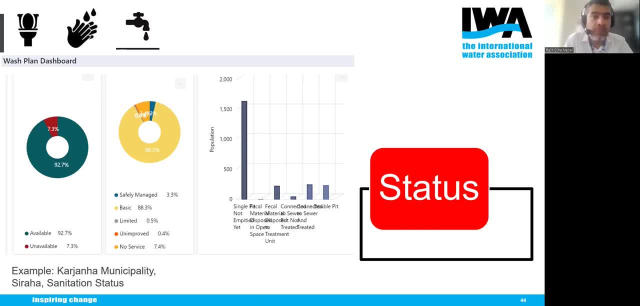 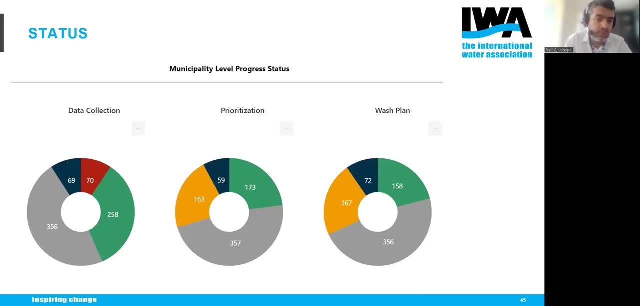 are going on, But mostly aligned with these are mostly aligned with JMP indicators, as pointed out before. So this is the status, that how much we have collected the data. More than among 753, more than 258 local governments have finished the data collection. 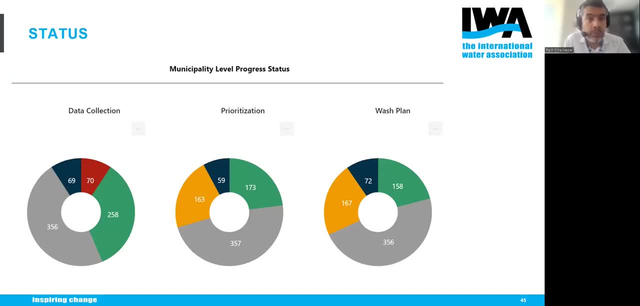 which will allow them to know their status. Then they will do the prioritization of the projects, which can be the project bank for the provincial governments And the federal governments as well, And then overall planning costs can be calculated and which we can see in terms of WASH plan. 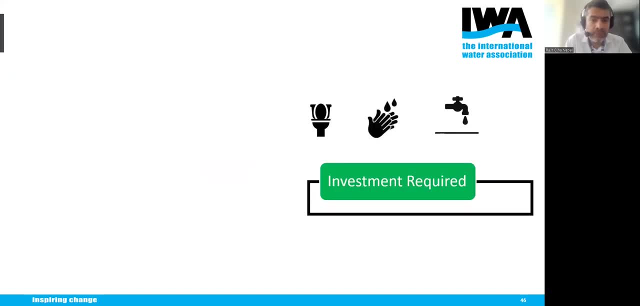 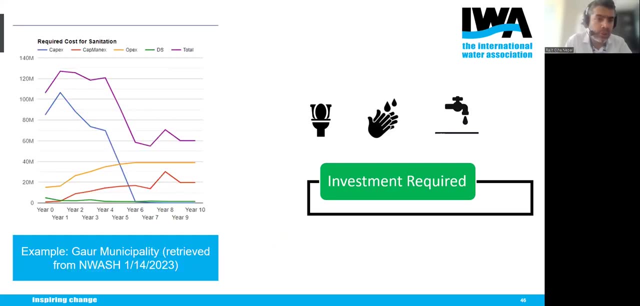 of 158 municipalities and rural municipalities, As I mentioned before, the calculation of investment requirements can also be calculated. This we have adapted based on the life cycle cost assessment. where we talk about the capital investment, We talk about the capital maintenance investments. 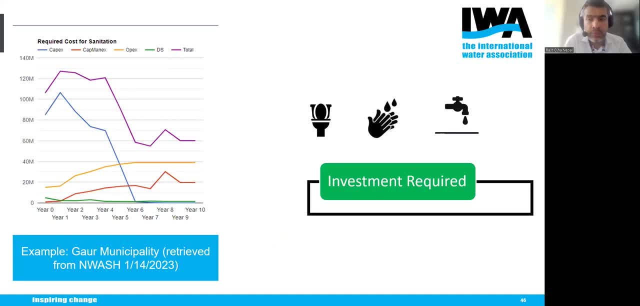 We talk about the operational expenditures, We talk about the direct support- capacity building support, Okay- And we talk about how much total investment will be required, And so, based on this one, we'll know how much investment will be required in one local government. 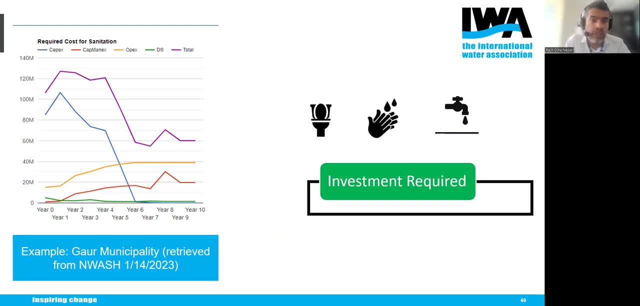 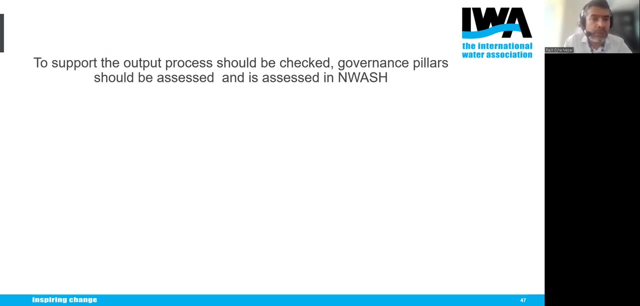 and how much investment will be required in the overall federal government. So this is allowing us to plan for the investment as well, And this is one of the example that shows how much investment will be required, based upon the local government's prioritization. So to support this, we identified there are a few governance pillars that should also. 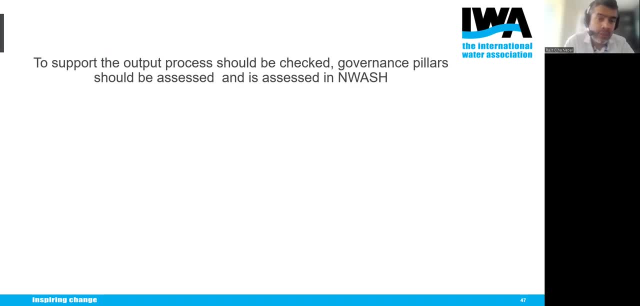 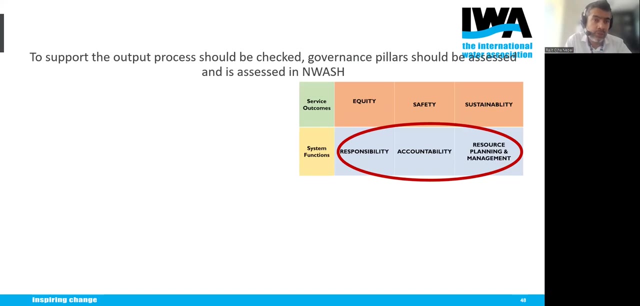 be assessed. We tried to link it with the citywide inclusive sanitation indicators as well. For example, how are the local governments updating the database and how they are using So it falls under the responsibility and accountability indicators of citywide inclusive sanitation. Similarly, we are also seeing what are the local legal frameworks are present so that 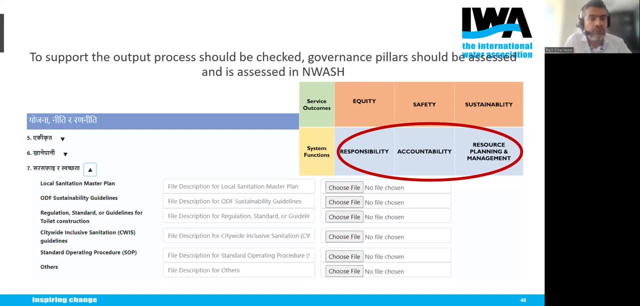 they could be able to regulate, they could be able to plan, they could be able to formulate the guidelines. Okay, So we are trying to identify the support, necessary support for the local government based on these data sets, So not only the output related data sets, we are also supporting them in terms of the 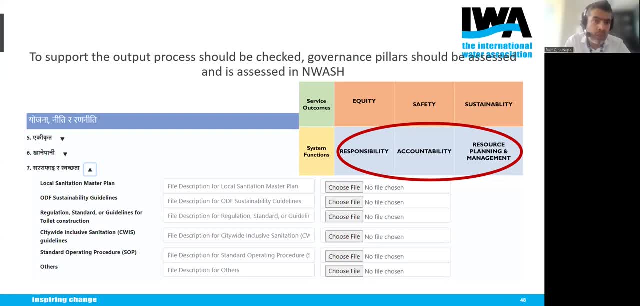 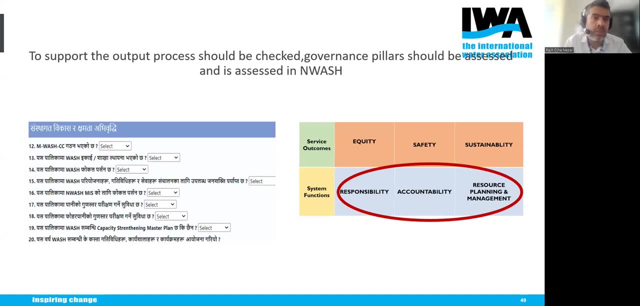 process data sets that will help them to strengthen the overall system. So this is like whether they have the human resource available or not, whether they have the TOR available or not. Okay, So we are trying to find those resources and where they are in terms of the organogram. 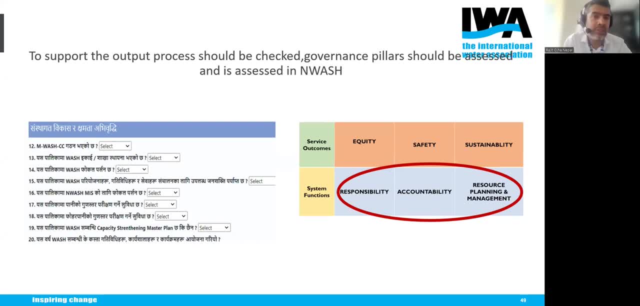 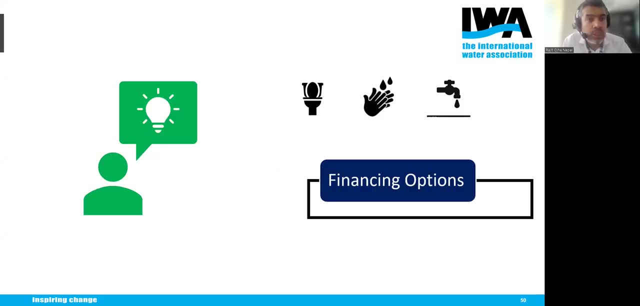 of local governments, whether they are getting the adequate training or not. So these kinds of areas also are under the discussion inside NWASH MIS. Then we talk about the financing option, where we talk about what can be the possible option for those local governments, how much tariff they can generate, how much tax they can use. 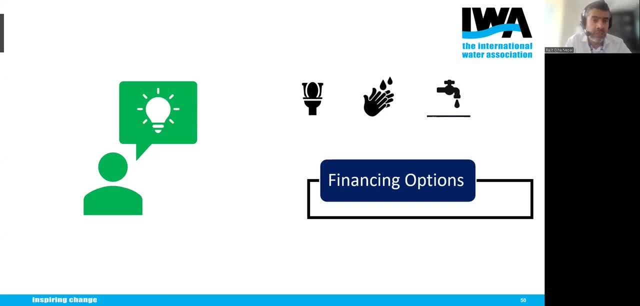 inside WASH how much transfer they are expecting from federal and federal government, provincial government and other development partners? also, is there a possibility of like bringing the private sector in terms of trade? how much self supply uh is happening there so that so that overall financing landscapes could be seen these? 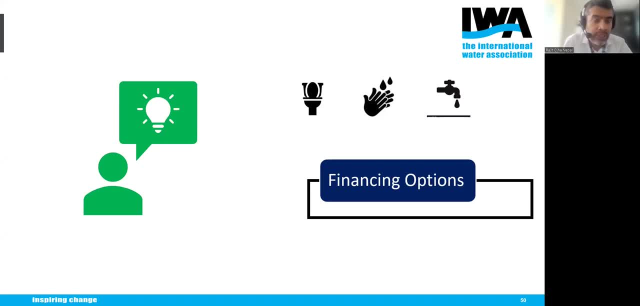 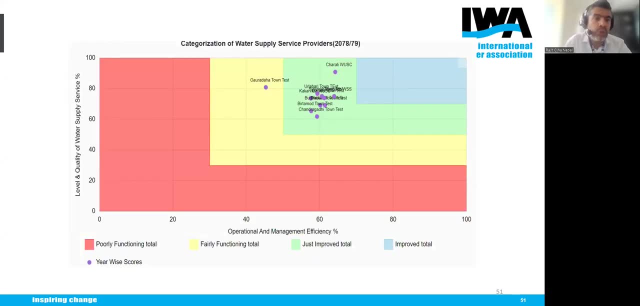 all indicators has been taken from the track fin initiative that we are doing now, um, with the support of who? uh. so this is one of the examples that we did for the water supply service providers which we are thinking of. uh, doing it in sanitation service provider as well, um, where we would be able. 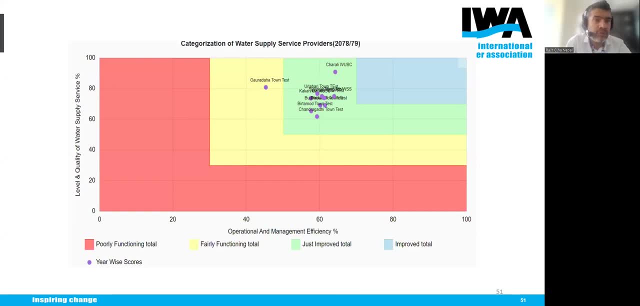 to track where they are in terms of level and quality of services. i am showing this now for the water supply services, but the similar kind of arrangements can be made for the sanitation service as well, where we can see the key performance indicators, such as like regularity of service. 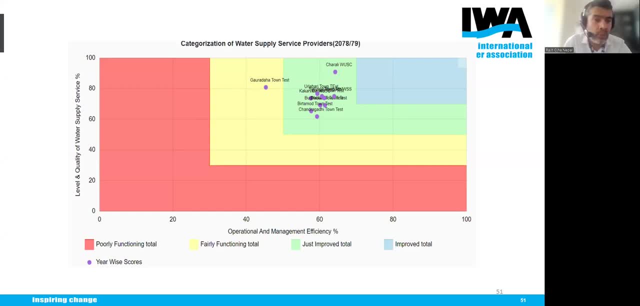 the coverage and this kind of service can be seen in terms of level and quality of water supply service. and then we can see the process indicators of those uh service provider in terms of operation and management efficiency, for example, like how they are doing the asset management, how they are. 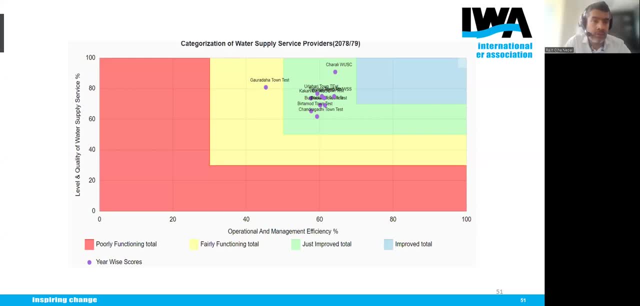 doing the accounting systems? uh, what is the billing efficiency? what is the metering efficiency? so these kind of indicators comes under the operation and management efficiency and based on this one, the operators, we can try to find out where the operators are lagging in terms of key performance. 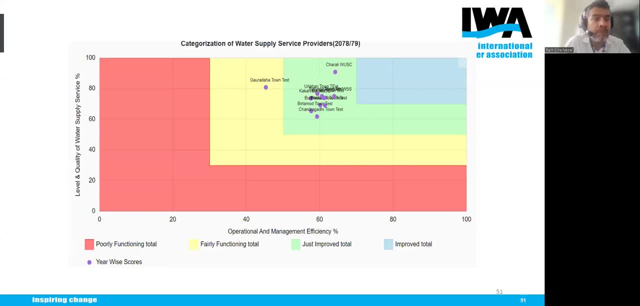 indicator. so this will fall under the federal regulation and we'll know which kind of support will be needed for the service provider. and we are hoping we could make the similar system for the sanitation service providers as well, which will allow us to formulate their business plan and which will allow us to build their capacity as well in terms of, let's say, for example, like 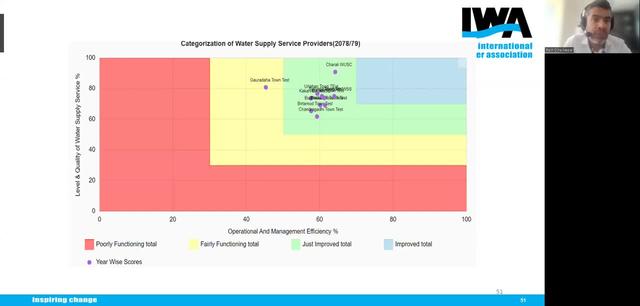 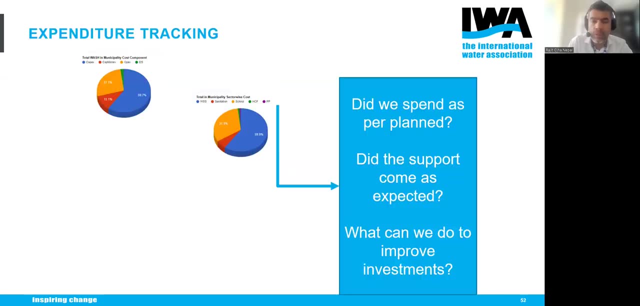 occupational health and safety, containment improvement, the transportation improvement and influence standards and everything. so, then, we are helping the local government track their expenditures, where we will know whether they are spending in terms of planning or not, whether the support came as expected or not, and what we can we do to improve the investment inside. 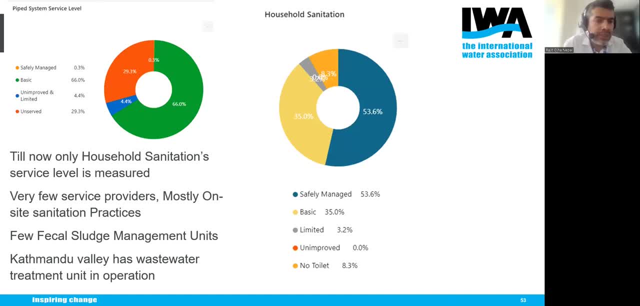 the local governments. uh, so till now the household sanitation only has been measured in terms of sanitation services. there are very few service providers in sanitation landscape, mostly on-site, on-site sanitation practices. so once the regulation is formulated, that is, in draft states, once the regulation is formulated, it will be our responsibility to build the sanitation. 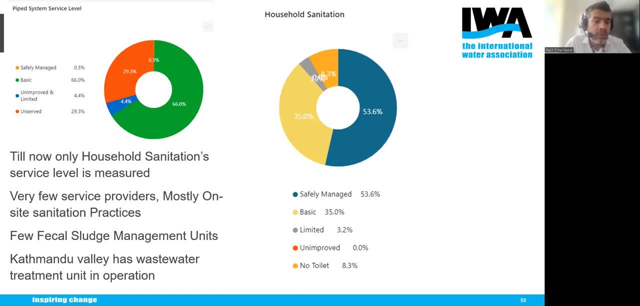 service providers through the licensing and everything. and, uh, only few vehicles loss management improvement management units. so, uh, once the capital investment goes there, we'll try to track the institutional data as well. uh, and only Kathmandu Valley has the wastewater treatment unit on operation. so because of that one, the service providers related data that I showed in. 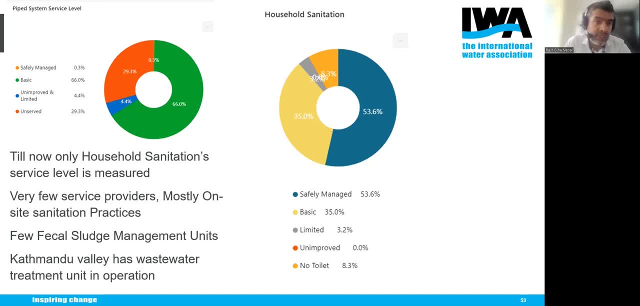 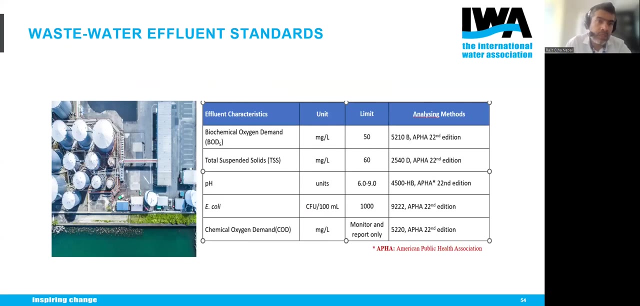 the water supply facilities are not available to us in sanitation facilities. but as soon as the regulation will be in the field, uh, this kind of data will come inside the unwashed MIS. so this is the wastewater influence standard that uh uh federal government has. uh, federal government. 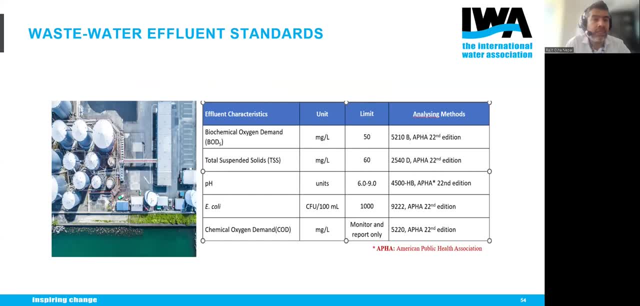 has approved so far and from this we can see there is a need for the utility, there is a need for the influence standard monitoring, there is a need for the containment monitoring, there is a need for the transportation monitoring, there is a need for the monitoring for the like whole sanitation value. 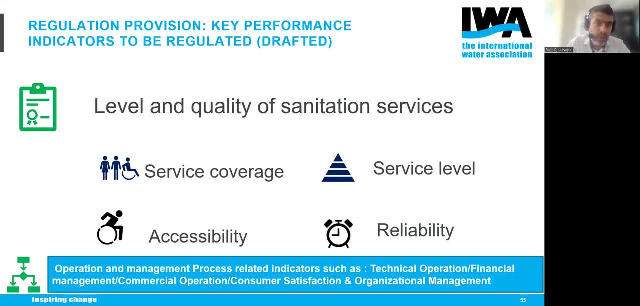 chain, as I mentioned before. uh, we can customize the KPIs for the service providers. for example, we can talk about the service coverage. nowadays, we can topic talk about service level, accessibility, reliability and operation and management process related indicators, such as like how they handle the asset management. this 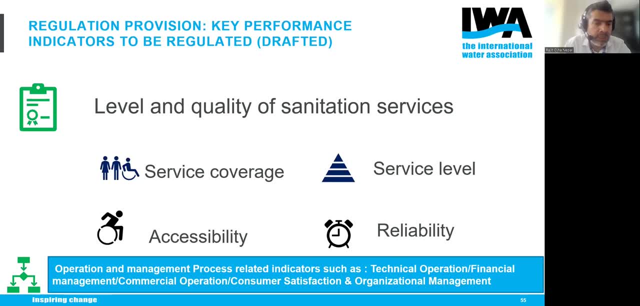 can fall under the technical operation how they are doing the financial management, inspection and organizational management inside that operator. so the this, this, this is under the draft regulation, which is allowing us to build the management information system which is allowing us to help them develop their own business plan based on those KPIs. so a few. 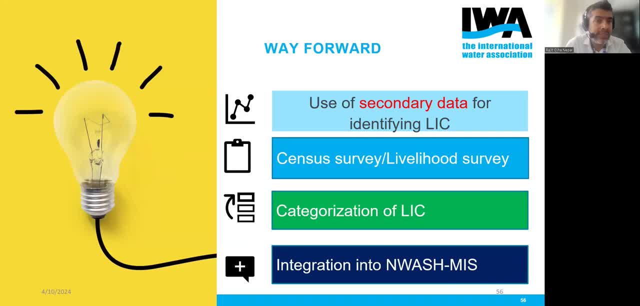 other words that I'm putting on is uh. we can use secondary data sets also, not only the uh, not only the primary data set, and this can come uh from the beginning. for example, low income community can be one of the data. those data sources are already uh in other data platforms and if we can make the 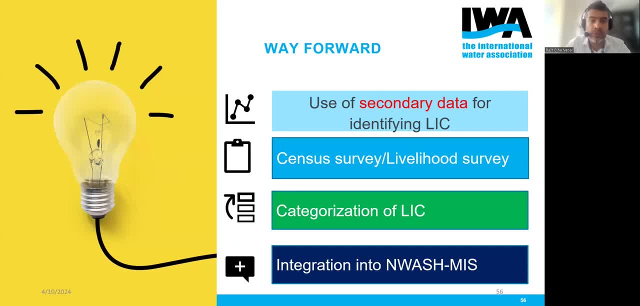 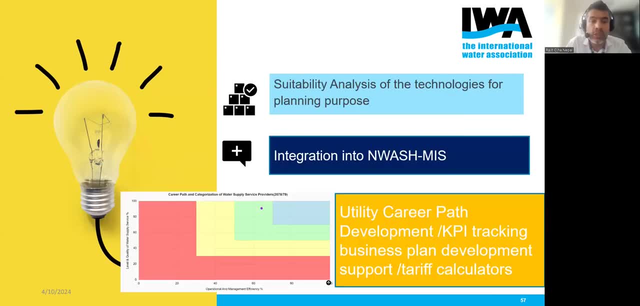 overall data platform interoperable. those kind of data sets can come inside our system um the categorization of LIC can be made based on that one, and we can easily integrate it into the National Wash MIS. the one thing that, uh, that is creating the hindrance in overall planning is: 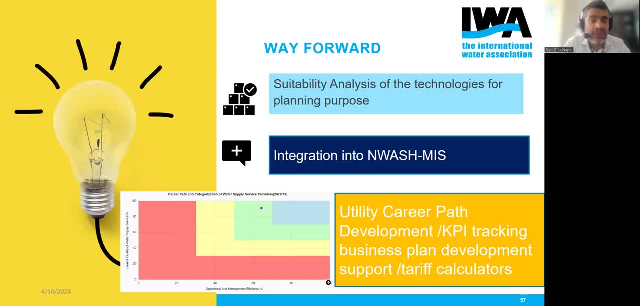 the suitability analysis of the technologies, because this can be double paid, this can be because loss management or this can be wastewater. so, and based on that one, the planning cost can vary on capital investment, on operation investment. so the suitability analysis is going to be very much important for us to plan the sanitation service and integration inside and wash MIS. 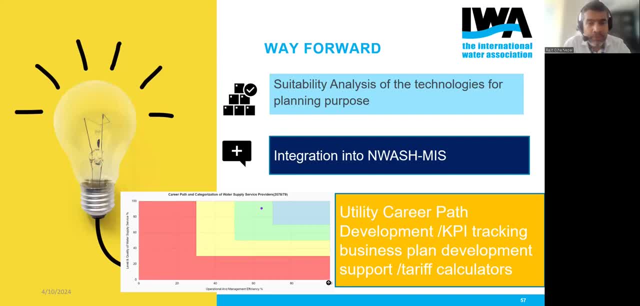 will be also important and based on our water supply. example, where we are trying to develop the utilities career path, we are trying to help them develop the business plan, we are trying to help the KPIs and also we are trying to develop the tariff calculator so that the local government would be able to fix the tariff for the 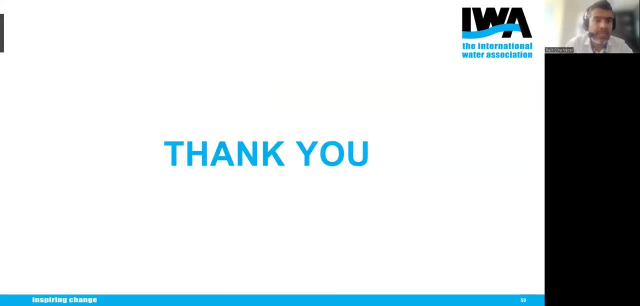 operators as well. so this is uh from my side. uh, any questions will be welcome later on. thank you very much. thank you, Rajitji. this was excellent in terms of capturing both the links to GMP, which I think earlier Rick talked about, but also very much to your own plans and investment. and how does monitoring system link to all this? I 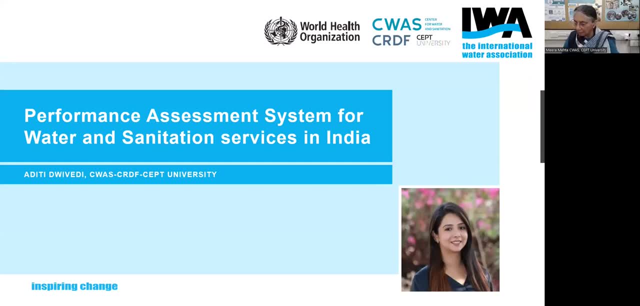 think it was excellent presentation. uh, let me now invite Aditi. Aditi actually works with our center in India and she's been associated with us for the last 10 years, and she leads our activities in both communications as well as in terms of improving monitoring systems, and we work both at as state. 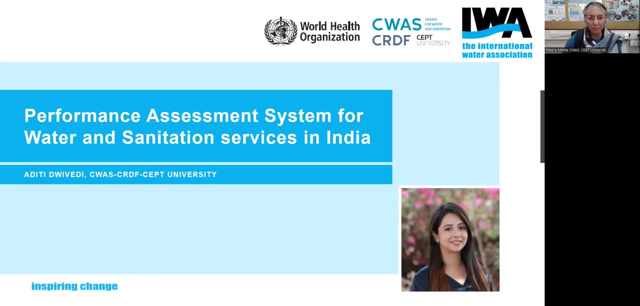 level, national level as well at local level. over to you, Aditi. thank you, Professor Meera. I am going to talk about the performance assessment system for water and sanitation services in India, and previous speakers talked about how there is often no data on nationalized data on on-site. 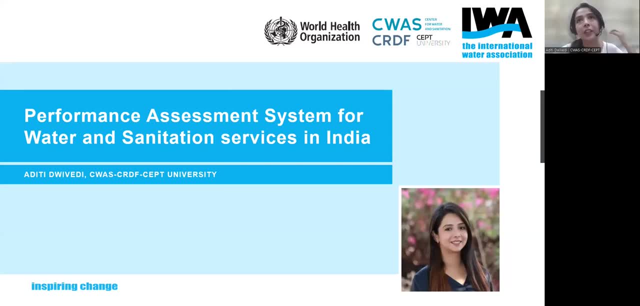 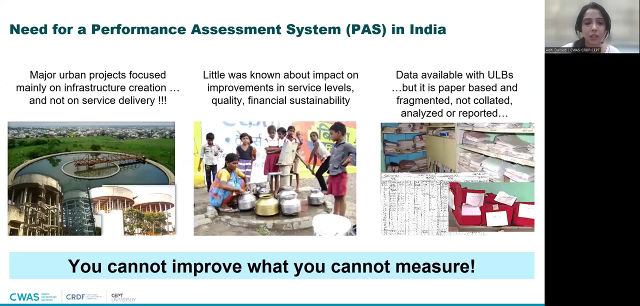 sanitation systems, which are more prevalent, or, uh, the need to track- uh- uh you know- the impact of investments and plan for investments in uh infrastructure. and pass also touches upon some of uh those uh issues, some of those uh solutions. uh for india. uh, when uh pass was yeah. so pass was initiated in 2009 and was housed at uh you know. 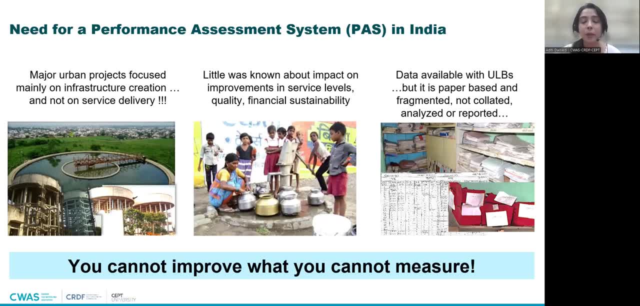 sept university and at the time it was conceptualized. that was a period of major investments in infrastructure in water and sanitation in india, but at that time very little was known about the impacts that this infrastructure was doing on the improvement in service levels. and of course you cannot try and improve what 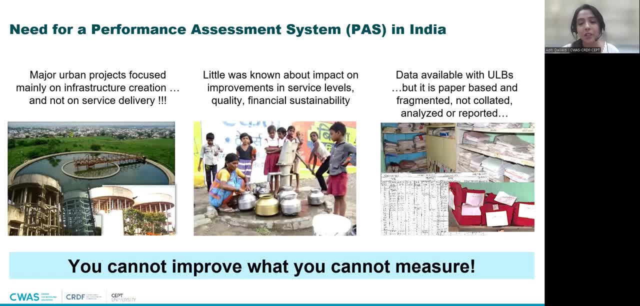 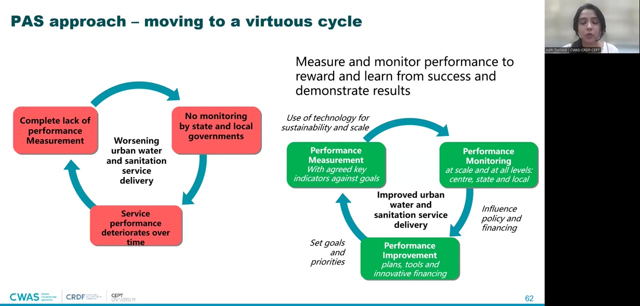 you cannot even measure. so the experience of our team was that data was available, a lot of data was available with the cities who were mandated to provide these services, but it was very disaggregated and not in a usable format. it was paper based and, you know, never analyzed. and that is what uh pass tried to. uh, that is what pass tried to work on it. uh. 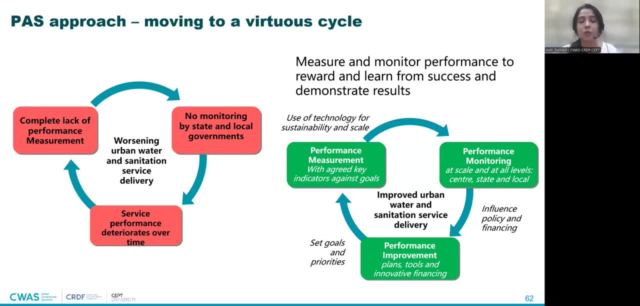 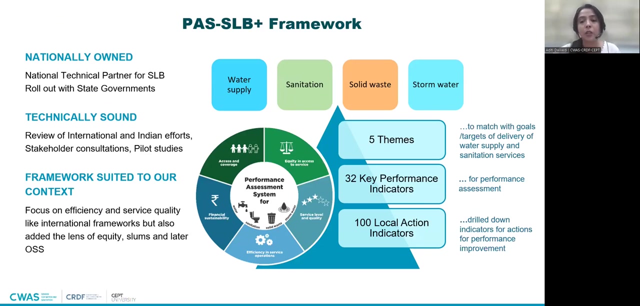 conceptualized, moving from a vicious cycle of, you know, no measurement, no monitoring and deteriorating services to a constant measurement and monitoring of performance, uh, with some uh in agreed upon indicators and, you know, setting the goals and priorities which will lead to continuous improvement. uh, and with that, uh cos developed this uh pass slb plus framework, which touched upon uh. 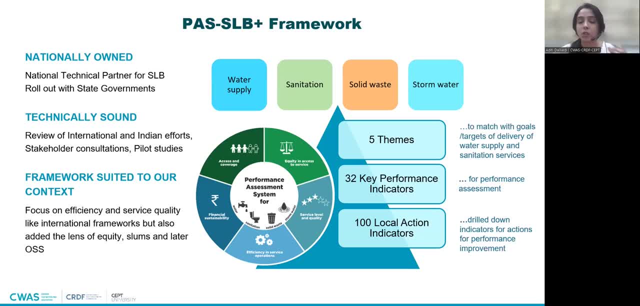 these four uh sectors- water supply, sanitation, solid waste, storm water- and uh had uh indicated on uh around five uh thematic areas uh and there were 32 key performance indicators and many other uh you know local drill down indicators uh for uh measuring and monitoring uh service delivery. 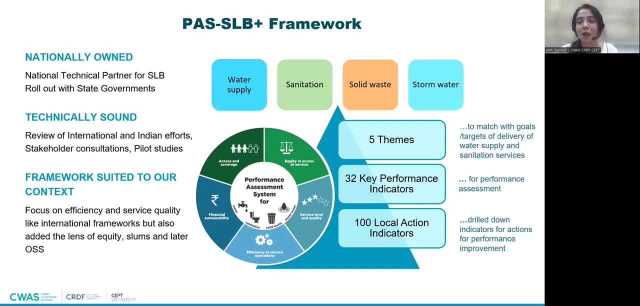 uh pass was not just an exercise by the university. it was also aligned with the national service level benchmarking initiative by government of india and was uh developed with a lot of review of international and indian efforts, uh stakeholder consultations, etc. and we also attempted to uh localize uh. 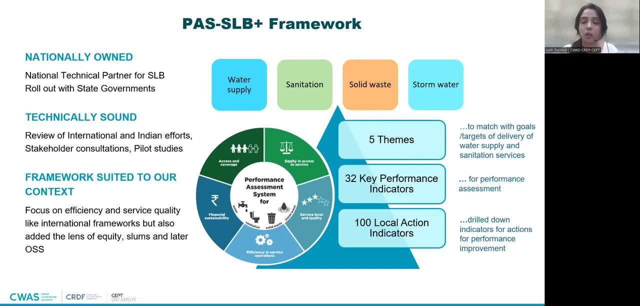 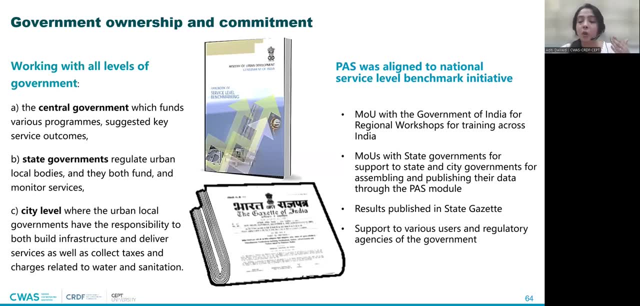 the indicators and suit them, suit the framework to local context. uh, and like i said, uh, it was not a university driven exercise. it was, uh, it was owned by the government and we made a lot of efforts to work with the central, state and city level governments. it was aligned to the national service level, benchmarking initiatives and 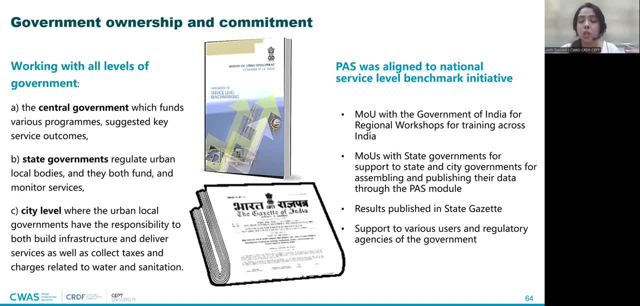 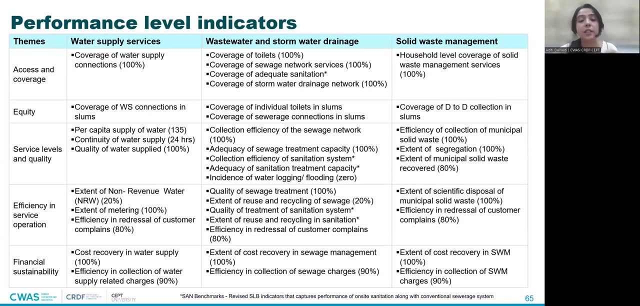 uh, various different uh uh institutionalized through among all big states as well as different countries, but also to the hmm. instructionalized through mous, and we worked with the government to provide support on various government users and regulatory agencies and in using the data. as you can see, these are the indicators across each of the service chains of the. 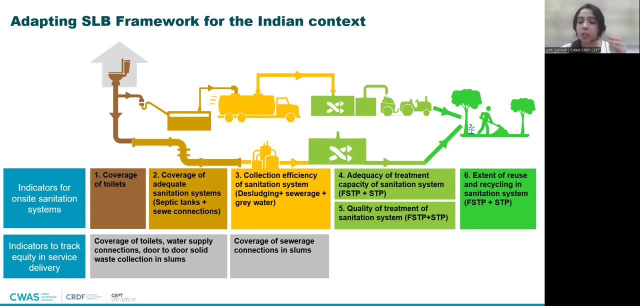 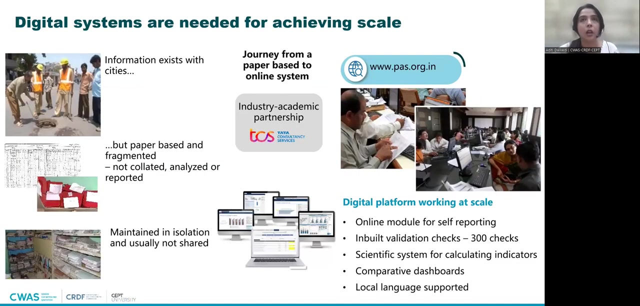 this to Indian context, where we realize a lot of cities did not have sewer networks and on-site systems were very prevalent. so this set of sand benchmarks were introduced, which you know also showed service levels on on-site systems, and there was an attempt to include indicators on equity and the coverage in, especially in slums, and this was not a one-off exercise and the idea 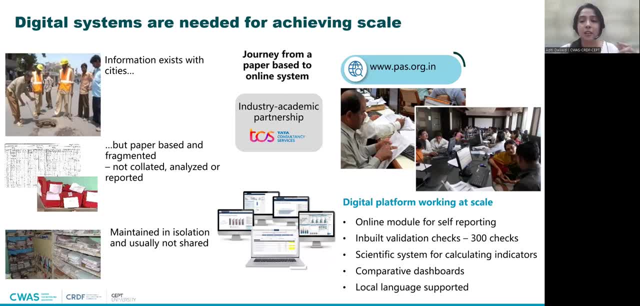 was to do this at scale and we realized that we required some digital systems to reduce the human effort and the geographical effort that is required to move at scale, and for that we developed this industry academic partnership with the Tata consultancy services and developed an online portal, passorgin, which consisted of a online module which cities could use to self-report. 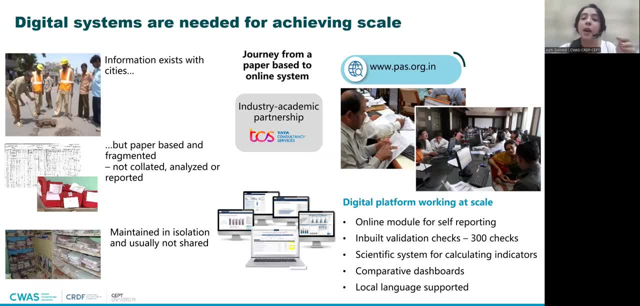 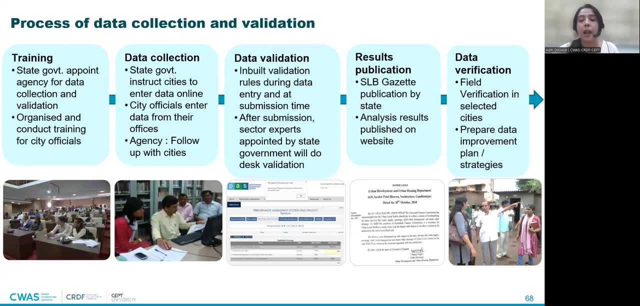 you know, sit in their cities and just report themselves, but also had a validation checks to keep, you know, the quality of data in check and with this online module we try to provide training to all these participating cities and roll out in many states and collect this data annually and also try, and you know, verify some part of it on ground. 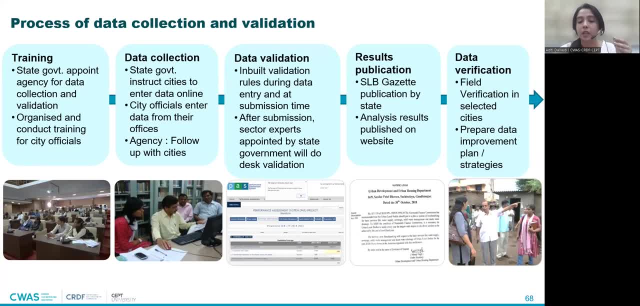 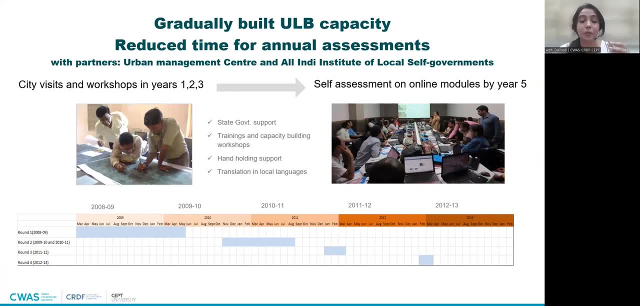 the results of these are published by the cities, by the states as part of, as part of Gazette, and over the years. the result is that the first exercise took one one and a half years to collect the first round of data and now we see that, after many years, this in two months, we are able. 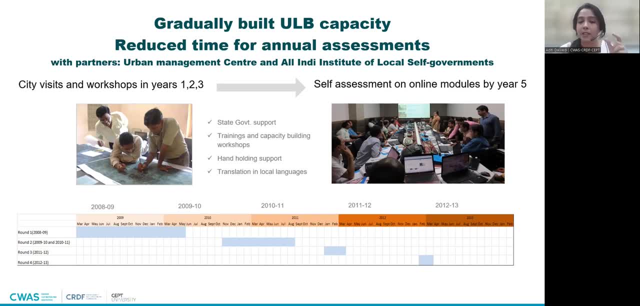 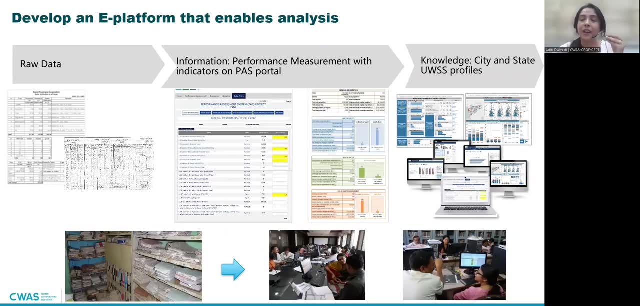 to you know, finish this annual exercise for all cities, and we are not just collecting the data, collecting and accumulating data. the data we've made it digital, so we've made it into digital information, but then, in order to use it, there is a need to have it in a 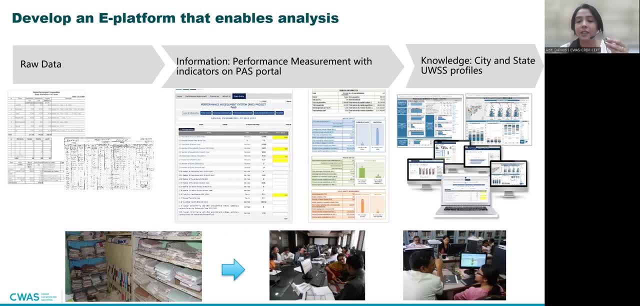 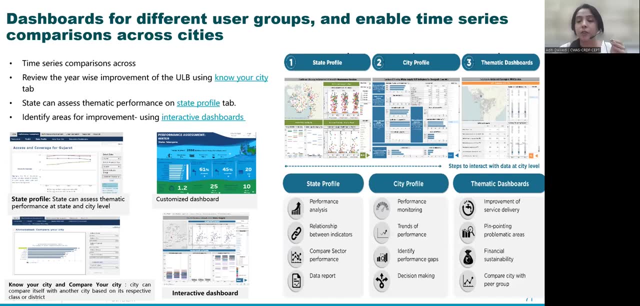 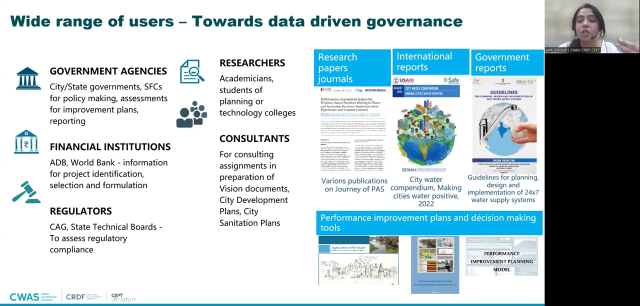 format that is. you know that could provide some insights, and so we have developed all these dashboards, which are focused on different stakeholders and different purposes, that use this big repository of data to provide some insights into how, in how, services can be improved, and this information has found a wide range of users. 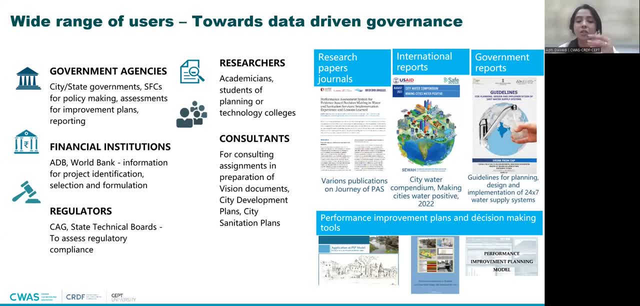 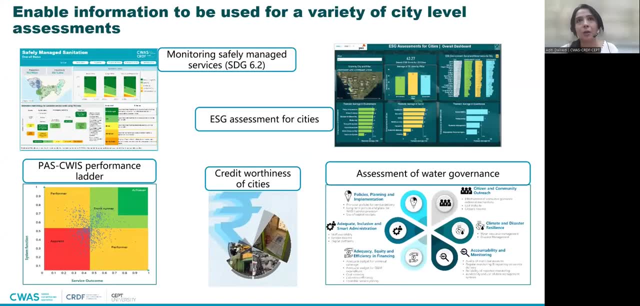 for data driven governments, from government agencies to researchers, to financial institutions, and also regulators and consultants. and it's not just reporting and improving on the services we have. there have been over the years there have been efforts to move this from just service, you know, looking at service delivery to the public sector, to the public sector to the 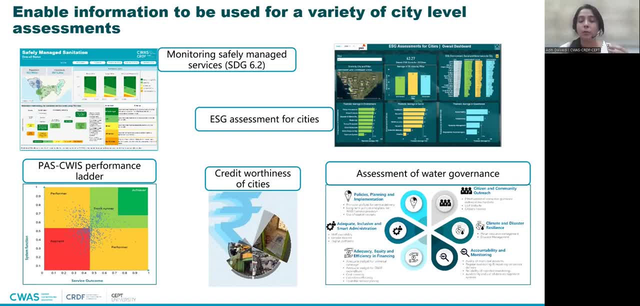 government industry or to the majority of underserved globalика, um, and to looking beyond this, to the government, sometimes, to when we do these outsourcing uh. so you know we do a lot of that, but you know we have also gone from the resource delivery to uh looking. 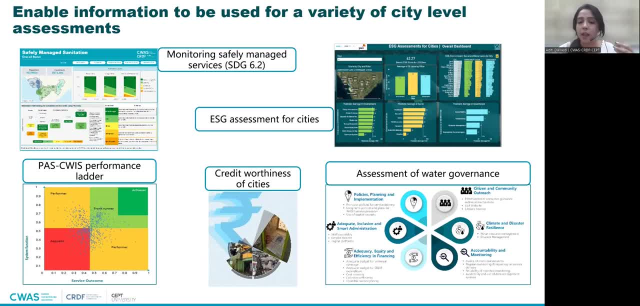 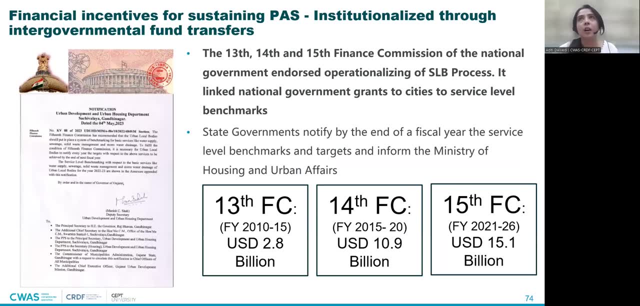 beyond, into, you know, the, using this data to look at the sdg performance or to move into assessing civis, citywide inclusive sanitation or esg assessment or creditworthiness of cities using some of the, you know, local action indicators, and also to look at water governance. 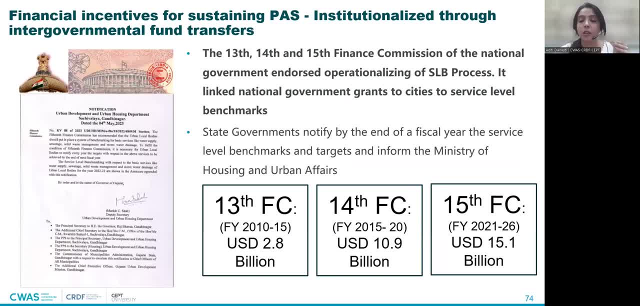 in a context of uh climate change. uh, the reason, uh one of the reasons this has uh sustained so far is because of the government support and the government tacit 1400, where the bill was made, and corresponding problem, the step swordagwick their system in science and operations. 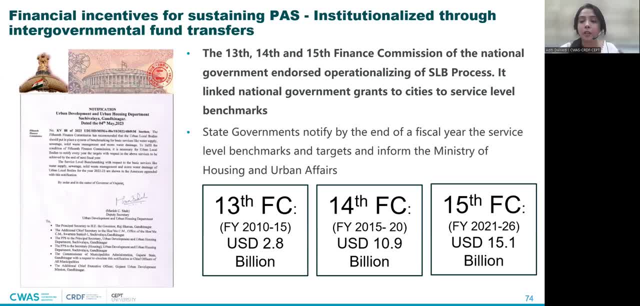 described the contribution of climate change which has to peecer, which kind of higher stability, a very positive pivot in the way climate change, apparently an approach to council administration, institutionalization, and this has also been institutionalized through intergovernmental fund transfers and the publication of this information every. 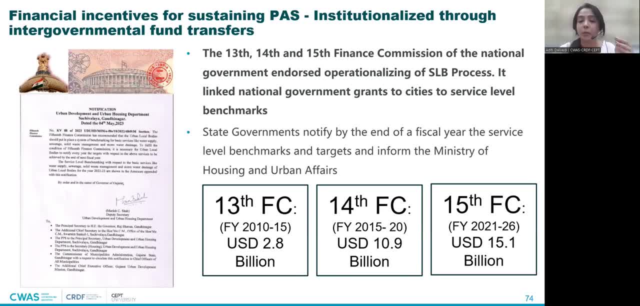 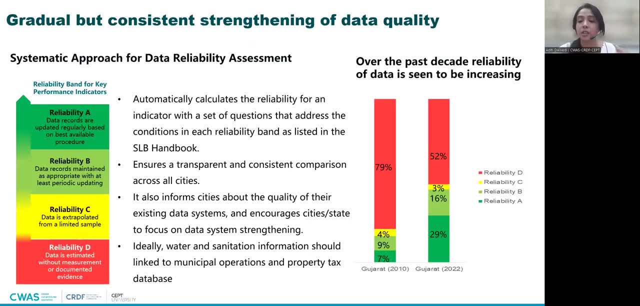 year by the cities is mandated by the, the, the Finance Commission, which dictates these intergovernmental fund transfers, and that has resulted in sustaining this program for so long, not so now that we have a system in place for measuring and regular monitoring of data. efforts have also been made over 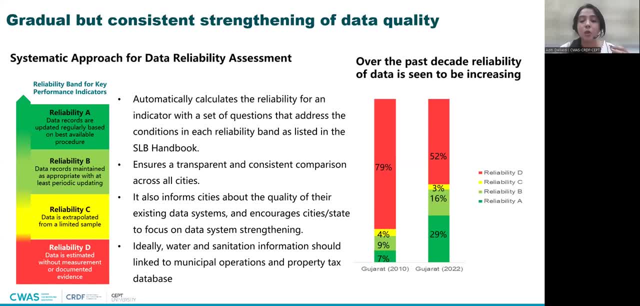 the years to look at data quality and, as I mentioned, the system looks, has a system has built-in validation checks to look at quality of data. but also there there are modules to look at the reliability of data, for example, in terms of whether the information that you are 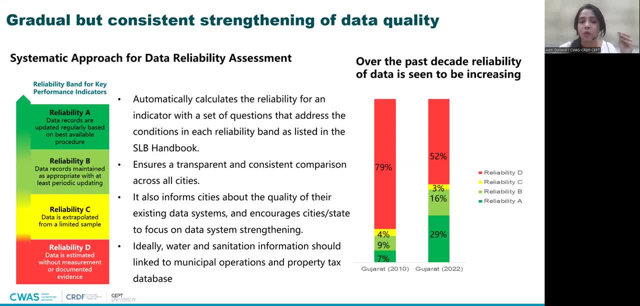 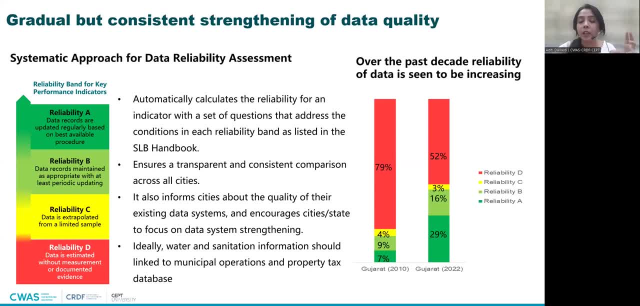 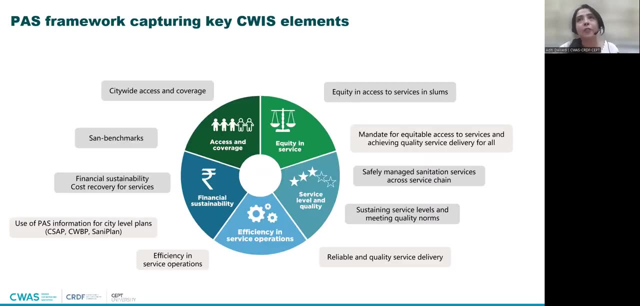 Gujarat. we have seen that from reliability D, there has been a lot of improvement towards reliability A, which is, you know, data records that are updated regularly based on very best available procedures. and if we talk about uh, inclusive uh, if we talk about a data strengthening or data governance for urban sanitation, the the latest. 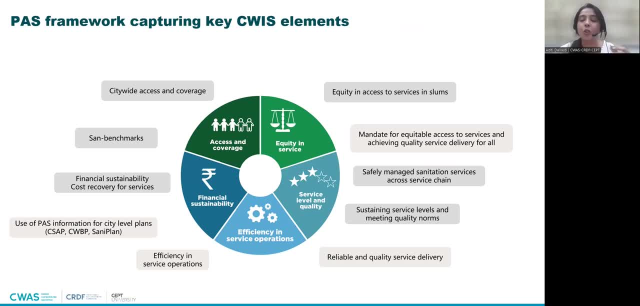 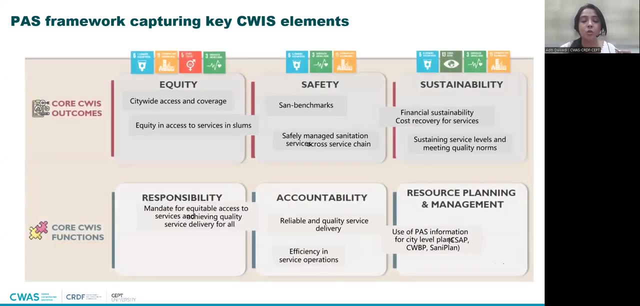 prevailing theory of change is citywide inclusive sanitation and even though pass is uh in its 15th year now and service is relatively uh new, we can see that many aspects, most of the aspects of service, are reflected uh in our past and can be used to uh uh. 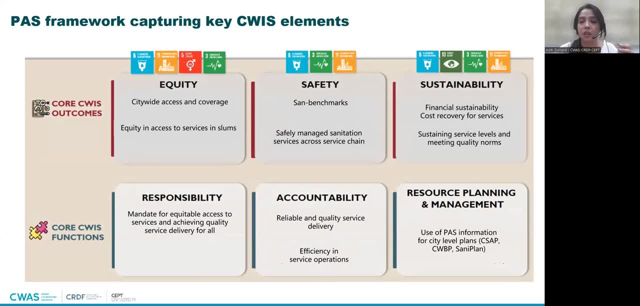 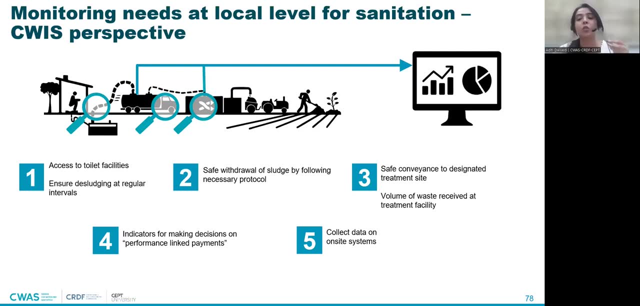 measure uh- the service, uh elements and uh to look at uh monitoring beyond. you know, city level pass provides this uh system to look at monitoring at city level and uh it has triggered many more uh monitoring systems that go beyond city level and look at sanitation monitoring across the service chain. to 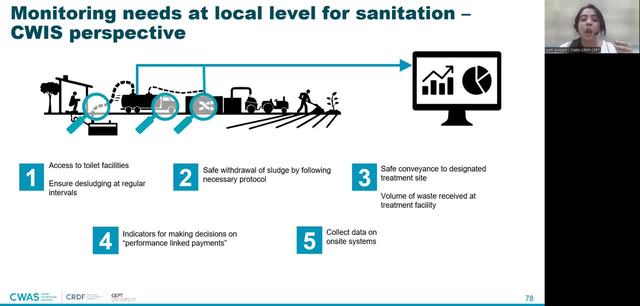 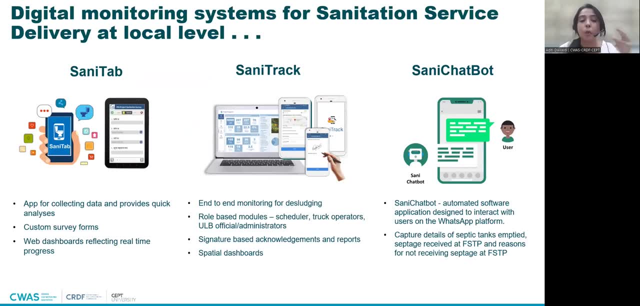 look at how service is provided for on-site systems, how data is collected, how private uh operators are involved, and we have looked and we have tried to develop more monitoring systems such as uh- these three are mentioned here- which look at uh, uh. you know how we can uh look at what type of uh septic tanks are available in the city and we have sanitap. 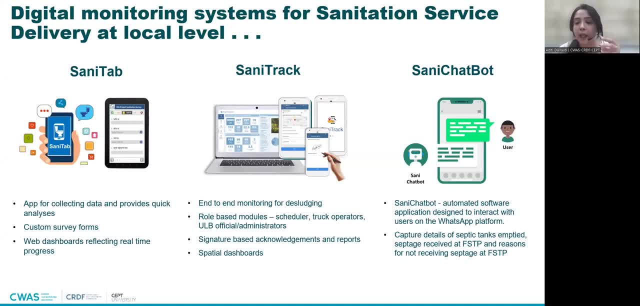 which can do custom questionnaires. to do that, we have Sani track, uh, which can look at end-to-end monitoring of uh dislodging of septic tanks, uh and uh. we have Sani chart board, which is a- you know, WhatsApp based text-based uh monitoring system for uh looking at the functioning of fstps. 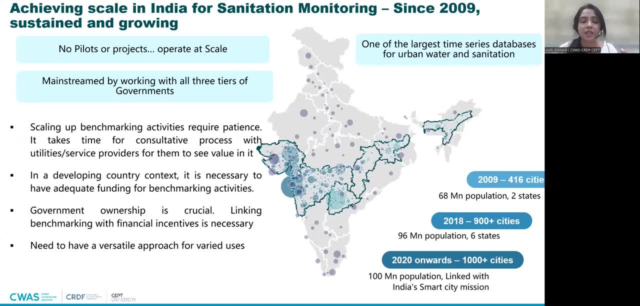 and uh. to conclude, over the years pass has sustained uh. it was not a pilot, it operated at scale and you can see here how it has scaled up from, you know, beginning uh with 400 cities to over thousand cities now and has sustained for many years. uh and uh. yeah, that that I will conclude. 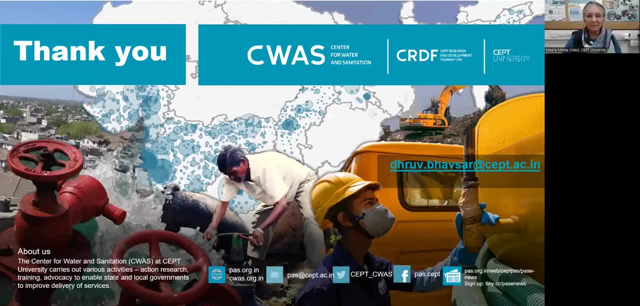 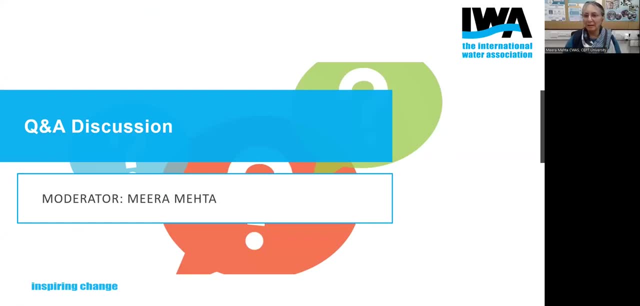 here uh over to you uh, Professor Neera. thanks, Aditi. uh, this is, of course, an activity that we have been involved in from the center and we worked with, as Aditi said, uh worked with uh state governments as well as national government in taking forward this whole idea and sustaining. 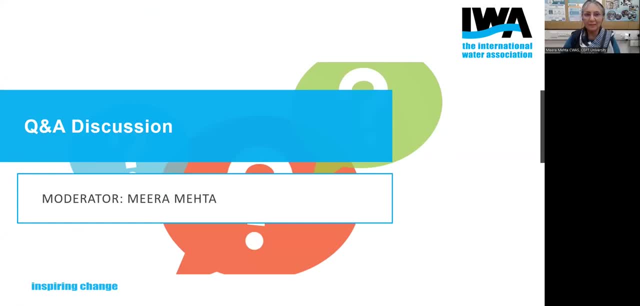 it over the years. so thanks very much, Aditi. let me open. let me, before I open up for any questions and answers. uh, I just wanted to highlight that a lot of people- participants- have put in links to various documents that they have worked on which relate to the kind. 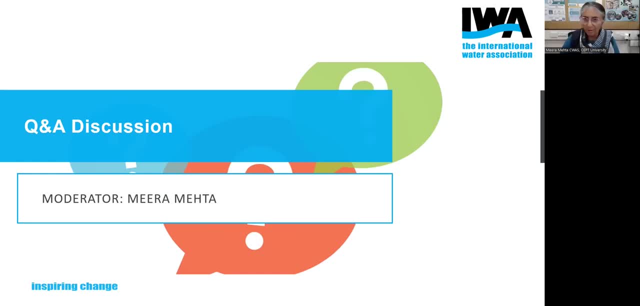 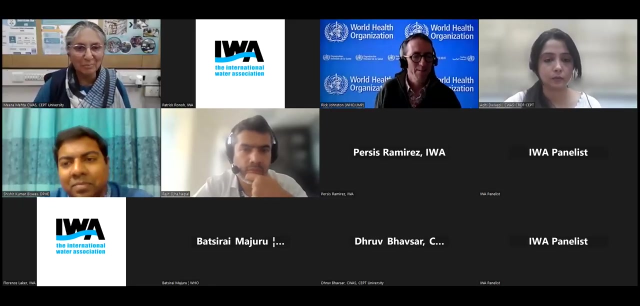 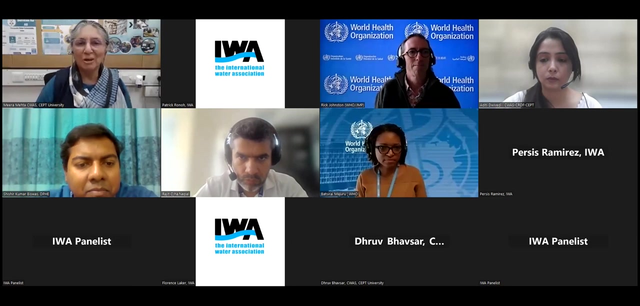 of discussions that we had, so it would be good to take a look and download whatever you think are likely to be useful for you. uh, may I have everybody's? uh. let me start with a question that has been put on the question chat. uh, and it's put to you, Rick, in terms of that you highlighted. 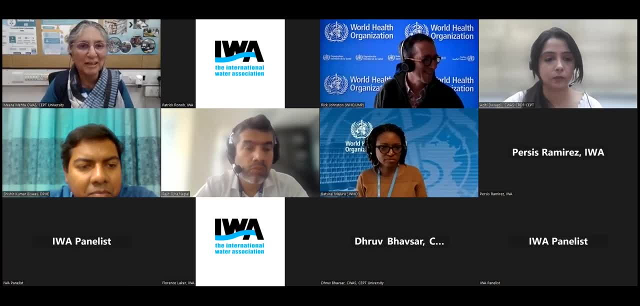 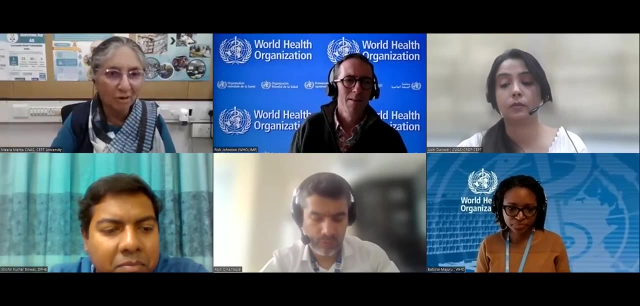 some data in red in your presentations in terms of the data that is missing, but what are the other key challenges that you think are needed in terms of- and let me embellish this question a bit- that the kind of uh examples that you saw from the three countries in terms of kind of data? 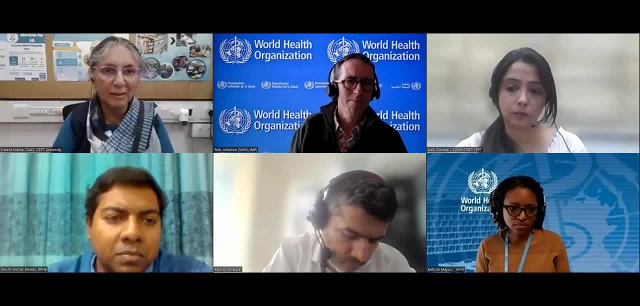 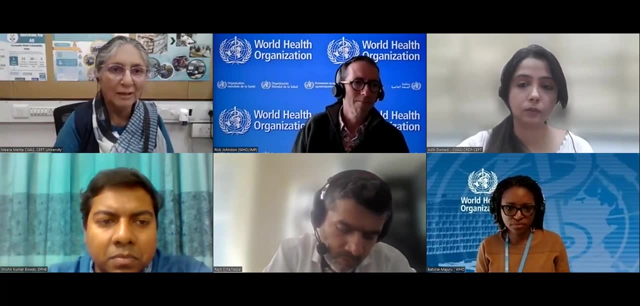 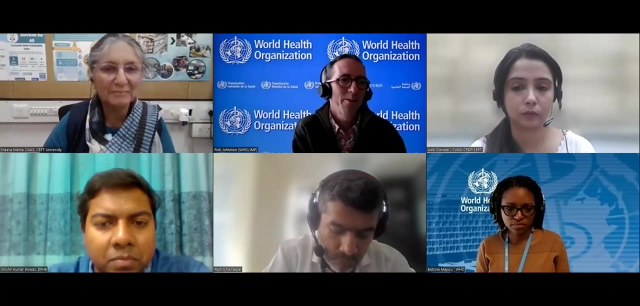 systems, kind of effort that different governments are making, both in terms of developing their plan but also introducing uh monitoring systems and so on. so what do you see as a good linkage between the two? thank you, Mira and um, I'm happy to start, but I think really the the national partners here. 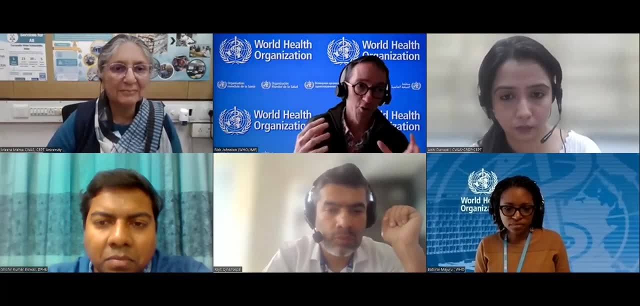 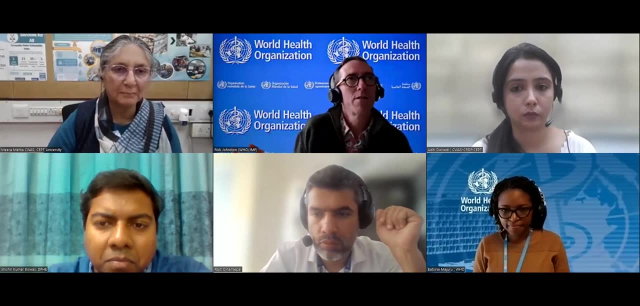 are in a better position to talk about the key challenges for strengthening data systems, because that's what they're doing and I think that's what they're doing, and I think that's what they're doing. but I can reiterate that, um, at least one of the challenges for SDG- monitoring at least- is that a. 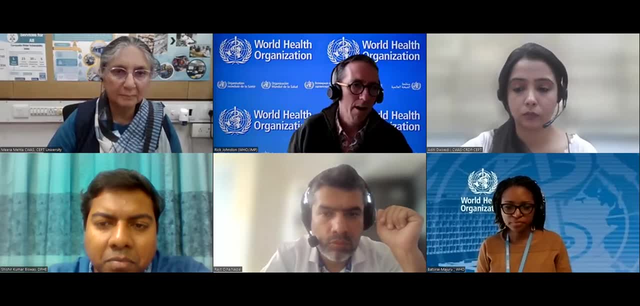 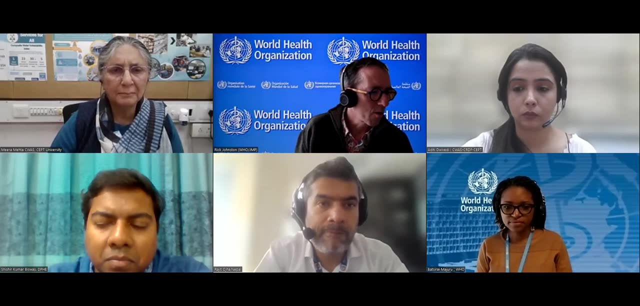 lot of the information that are collected at the local scale are not aggregated to the national scale. maybe they're not covering the entire population, and I think there's a real question about who has access to the data and and the ability to use it. so I'm very happy to see the 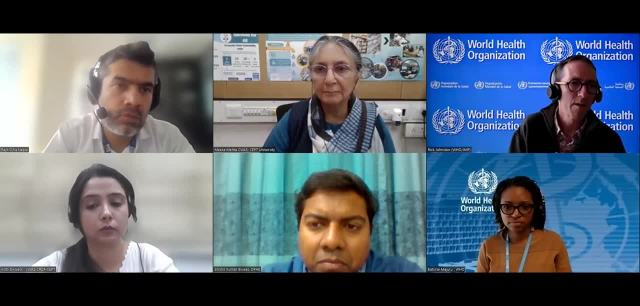 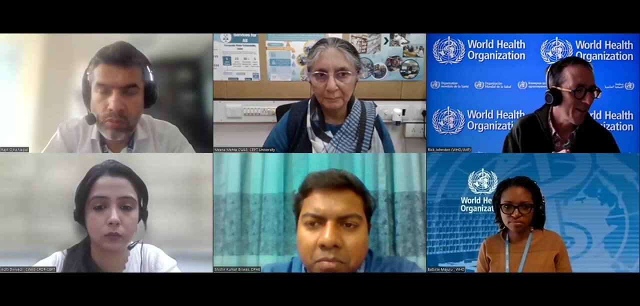 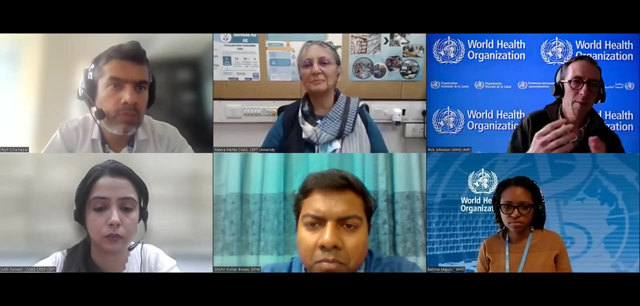 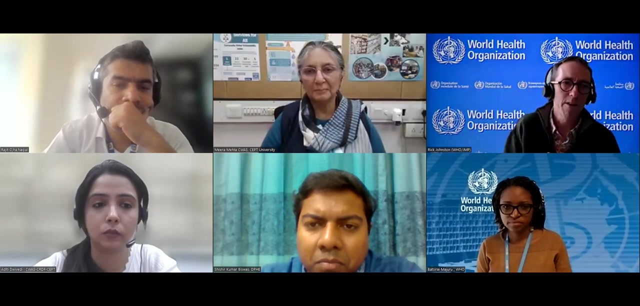 open data portals um in, in, in in the three countries that have been participating today. I I do want to reiterate that um regulators are an excellent um way for data on services to be collected and made publicly available. and, Mira, I take your point that maybe in these countries there aren't independent regulators. uh, in the 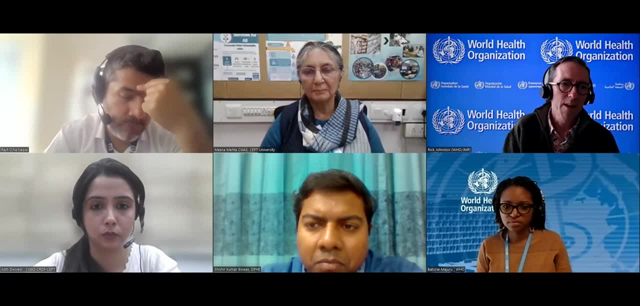 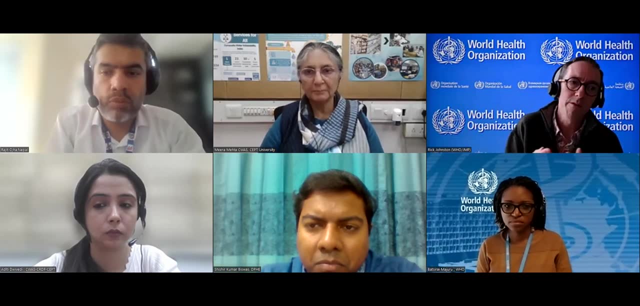 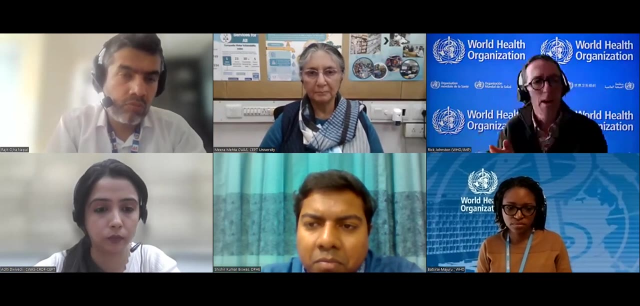 way that there are in some of the African countries. but still, even without a formal independent regulatory body, there can be institutions that form uh, perform the, the roles of regulation, and that can still help in both making data publicly available and improving service delivery. so the specific types of data I mean- I mentioned that- for 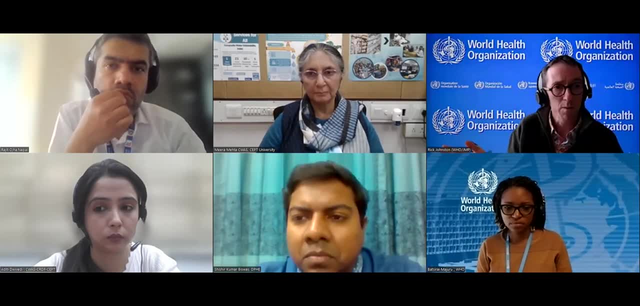 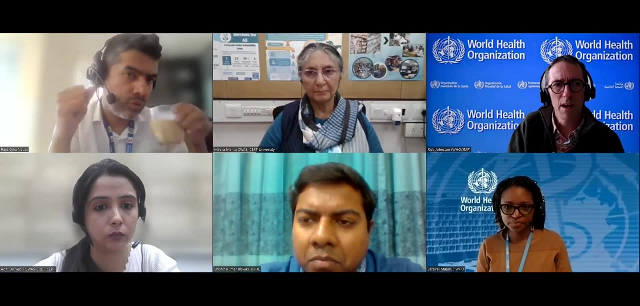 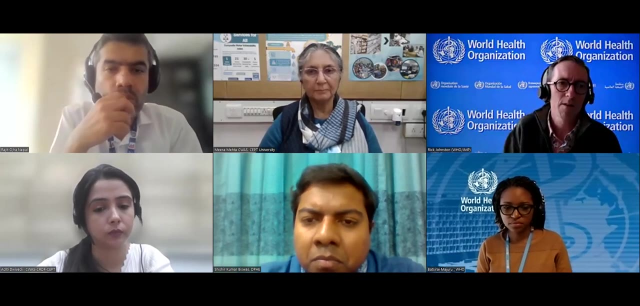 these countries. apart from India, we didn't have national data on centralized wastewater treatment. but more generally, I think data on the on-site sanitation is what's really lacking, and especially just on that, you know, on the facility itself: um, how well is it constructed and how well is it containing wastes? I see I see more focus on fsm and 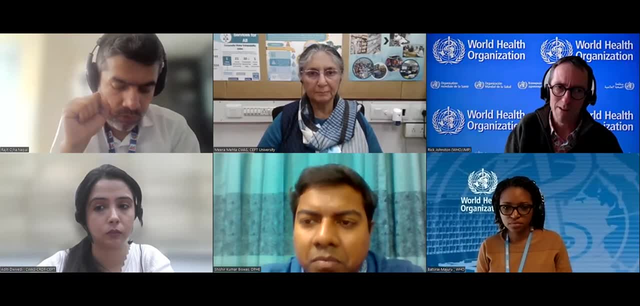 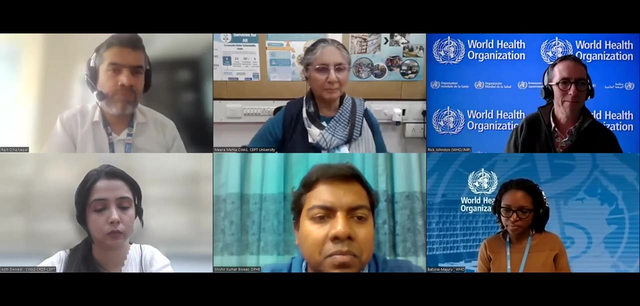 trucking and fstps than on, just you know, is that thing really a septic tank and is it really containing the wastes? but I'd like to hear from others, and also Batsy- uh, I think you had some some reflections on this topic to share as well. go ahead, I think you're put up. yeah, so, um, I think one. 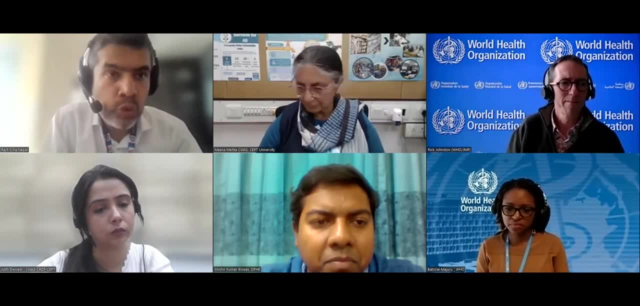 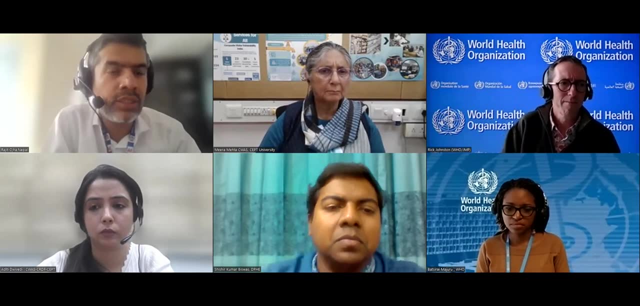 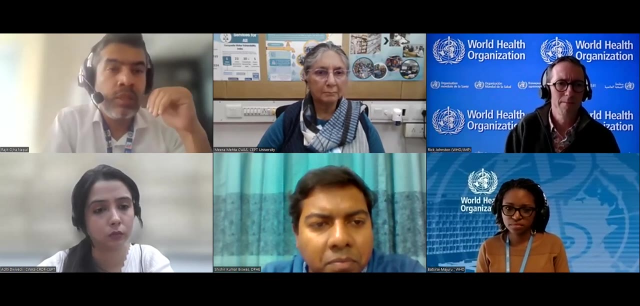 of the biggest challenges, like um to two kind of infancy periods that we need to look upon and start handling the challenge. the first one is the governance- in fancy because we are talking mostly service riders from the local government's angle- but I think the major capacity and major knowledge development and everything, 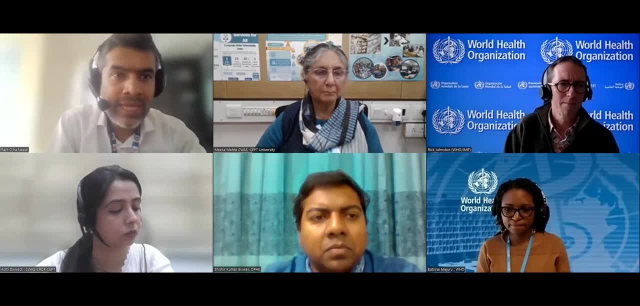 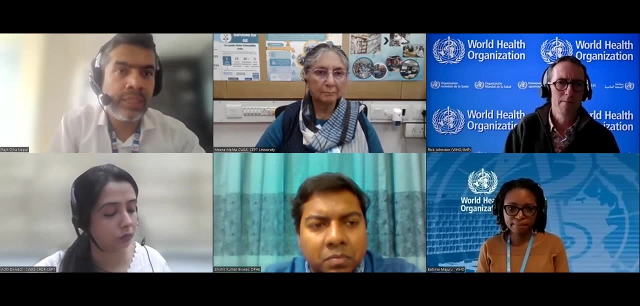 falls under the federal government's responsibility. so it's like how you trickle down those capacity building initiative to local governments becomes very much important and also- uh, it should be- the realization of local governments that the vast systems data is going to impact them is going to be like a biggest challenge and maybe that is also the biggest. 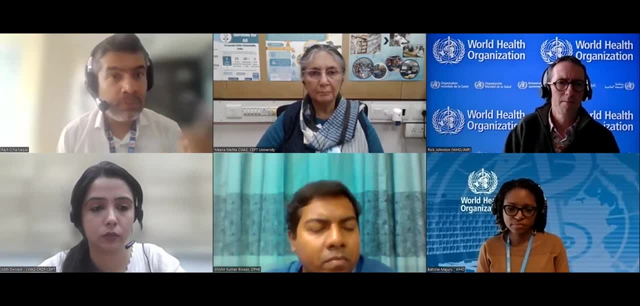 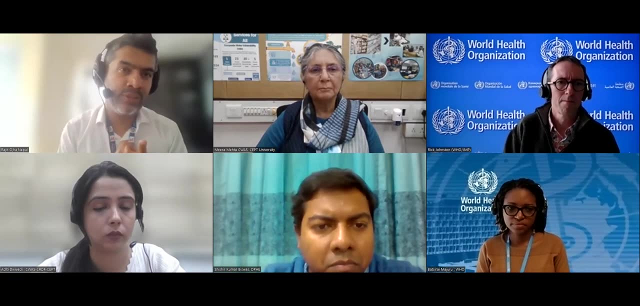 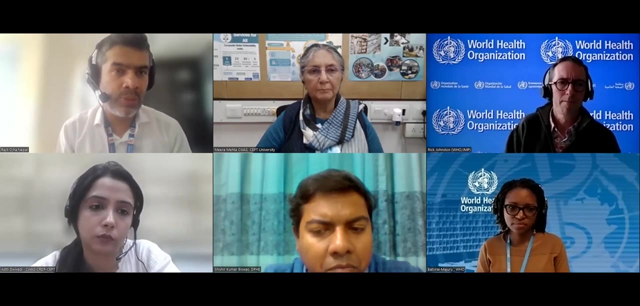 opportunity that we can, that we can use. similarly, the service providers in fancy also plays role. for example, I was talking about the right now. the sanitation services are not even licensed in the absence of regulation. so how do we manage to bring them inside the regulatory landscape and how we can use those operational data? 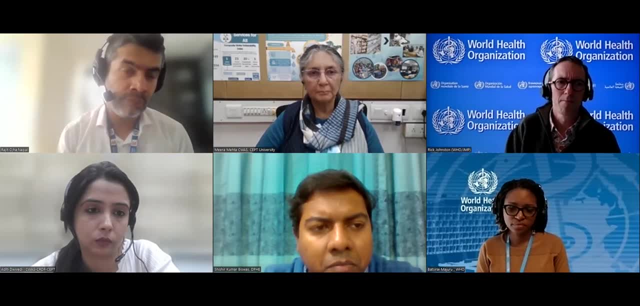 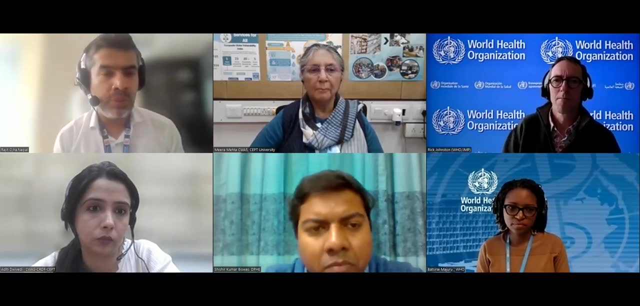 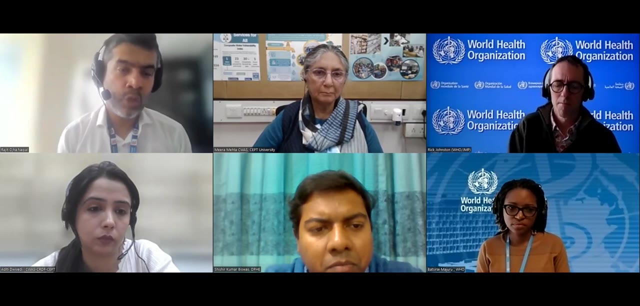 in order to make ourselves better is going to be very much important. so, once the service providers are aligned, the regulators are not the one which are which will going to be enforcing them to operate, but will be the one who will be facilitating them to operate according to. 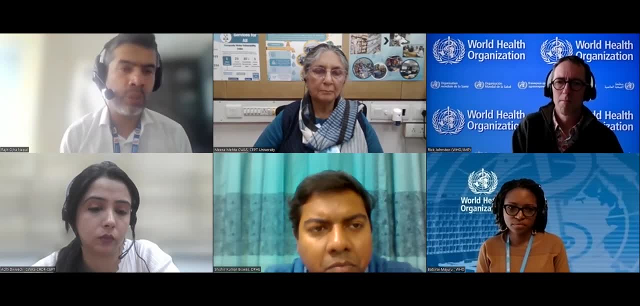 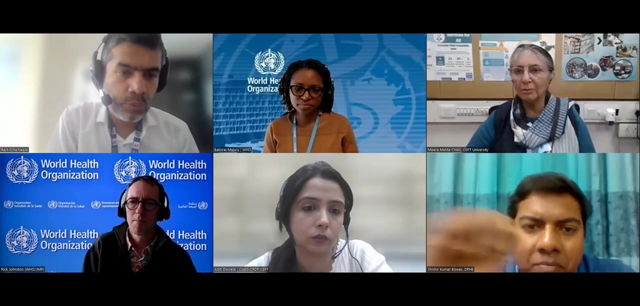 business plan. so, rather than being enforceable, how the government, government system becomes facilitative towards the service provider to bring the data forward is going to be very much way forward, i think, to cope with that challenge. i think, thank you. thank you, i think she did. you want to come in. you put up. well, thank you very much, actually, uh. 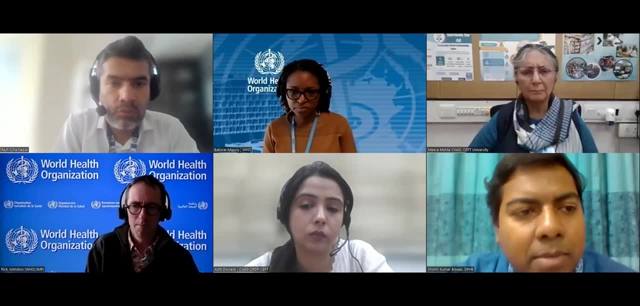 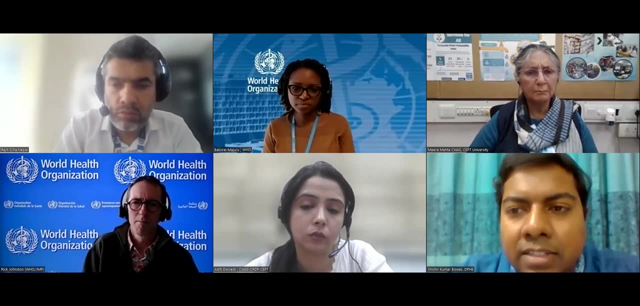 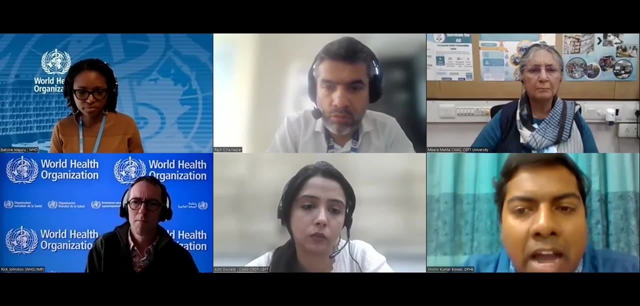 regarding the data collection, that is the another part. and but establishing a sustainable value chain of the waste management, that is another part. what rajit actually uh said, it is uh really correct. in south asian region, in bangladesh, you know that the from the higher end- i mean from government and service provider- as level uh for. 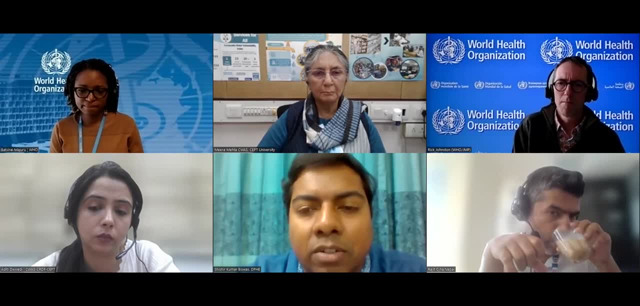 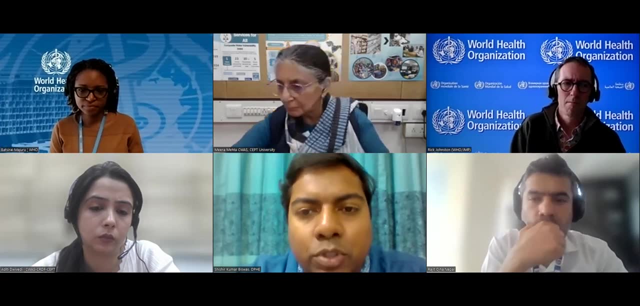 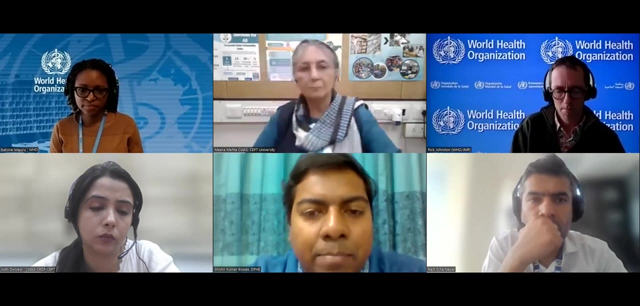 the rural and also for the city corporations or the municipalities. it's quite so okay. under project-based activities, the development wars are going on, but after completion of this project, uh, you know that the acceptance and sustaining the development activities and providing their uh every components data to. 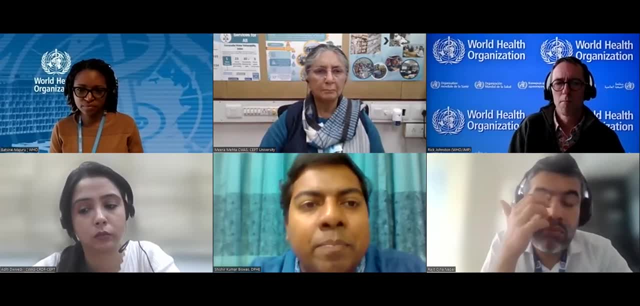 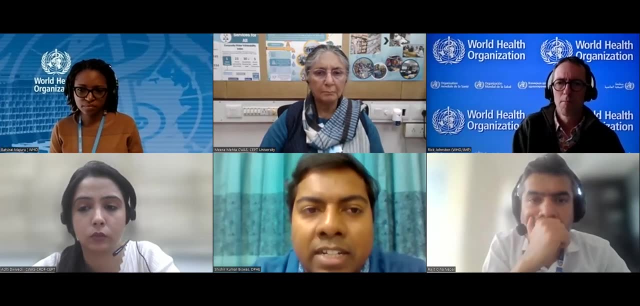 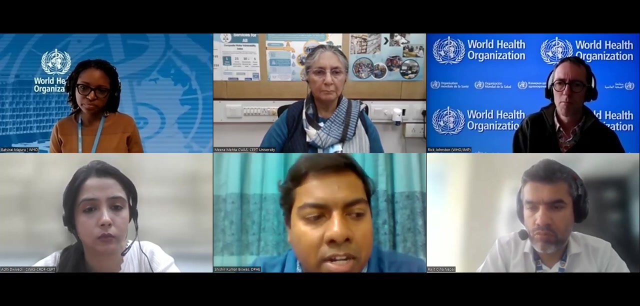 the data preserving center. that is not we are finding in a good shape. yes, uh, establishing a regulatory body. it's a huge challenge still now, but before that, for bangladesh context development of sustainable service is also very, very much important. yes, we are doing a lot. our different organizations, all the sector partners are really coming forward. for 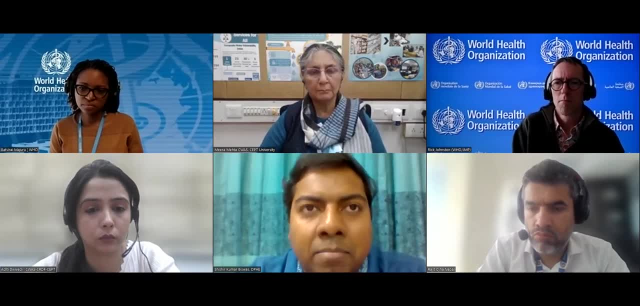 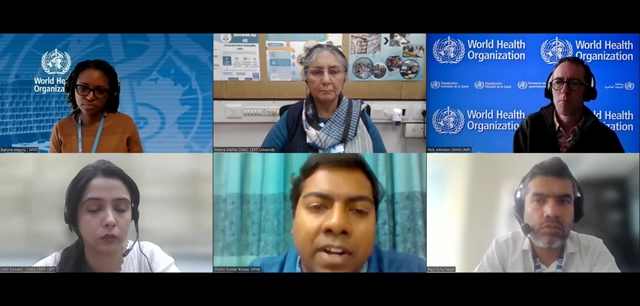 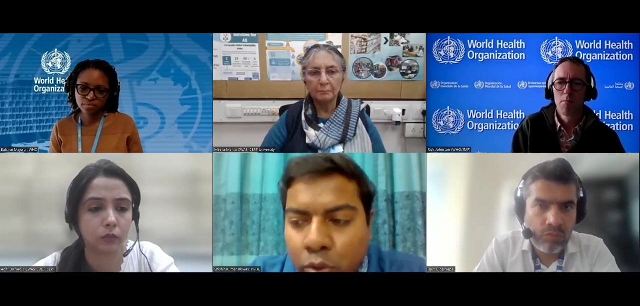 providing these facilities. from my previous experience, without giving a certain services, whatever activities for this improvement of the value chain, this will not be actually sustainable. so, after strengthening the local government institutions, the root level, the villages, the rural, urbans, all of those, so the accountability, the responsibility need to be grown for us from. 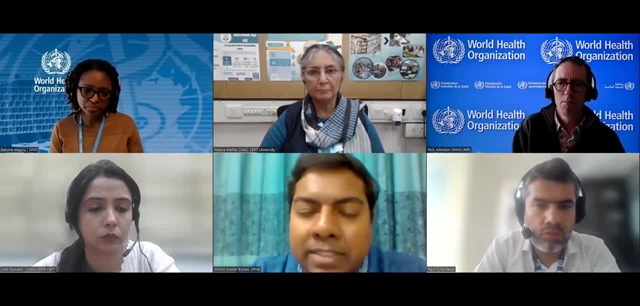 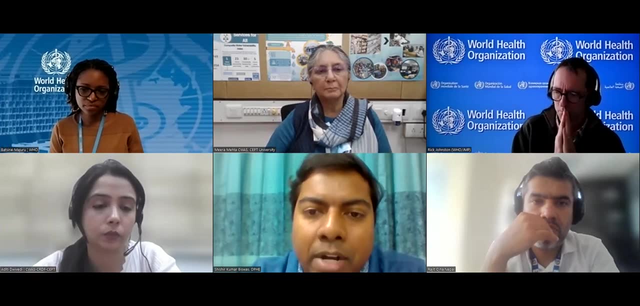 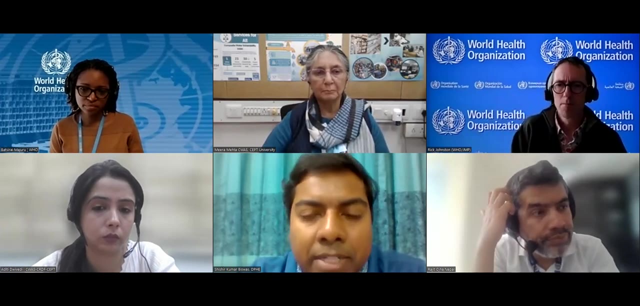 their site. yes, capacity building and awareness campaign program is a huge from our country, uh our. we have uh different mou with different development partners. bmgs comes forward and we have established a thub and cb hub. cb hub means capacity building hub. the other institutions, sector partners, like s nv hub, which is trying to 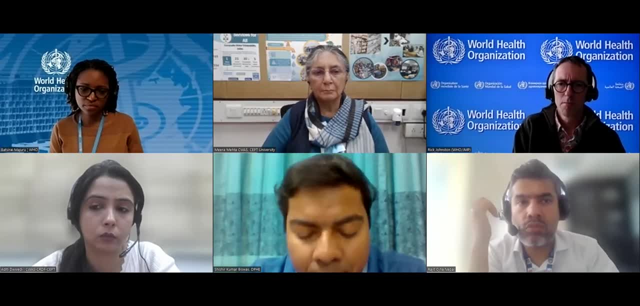 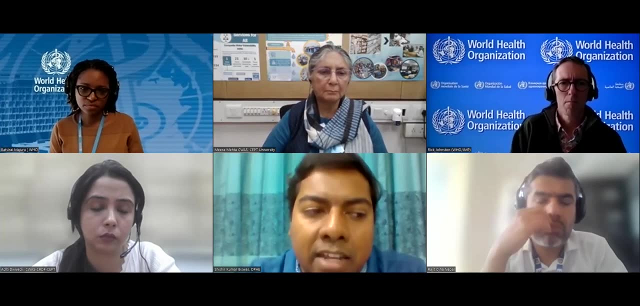 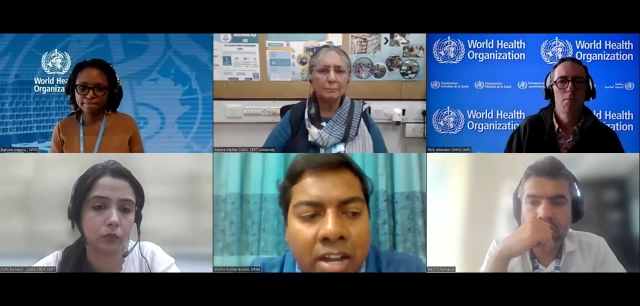 like S&V, WaterAid. all of those are really providing a good job, good service and our local government institutions members, the technical members and the political members coming there and getting knowledge of every component of this value chain. But at the end, what can I say? 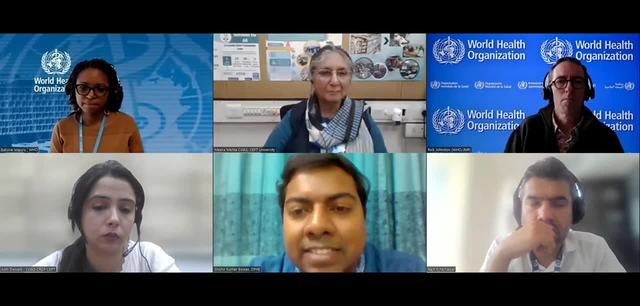 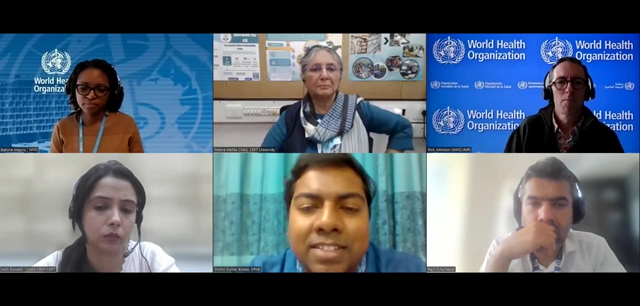 That the service, sustaining the service, goes to those institutions and providing this information to our central level. that is also be strengthened from their side And we, the central government, just could help them with different phenomena, something like this: Thanks, Shishi. 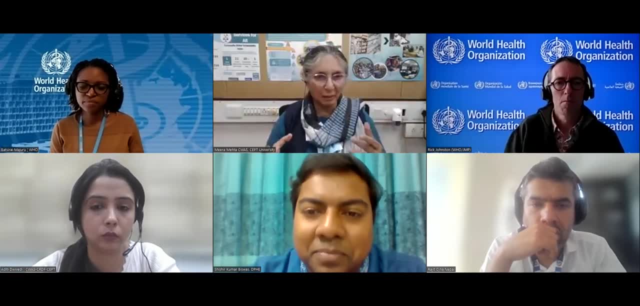 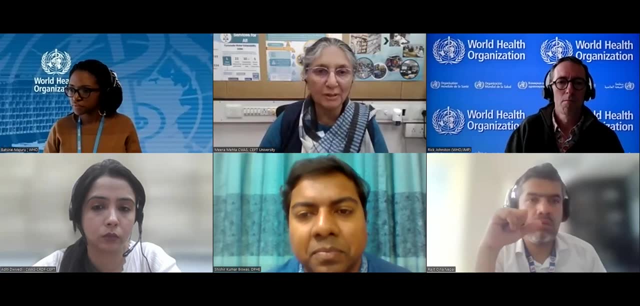 I know it's a balancing between national government and local government and how do you connect? How do you connect the two through better monitoring systems and what is role of each level is very important. I think we have Batsirai. I hope I'm pronouncing it correct. 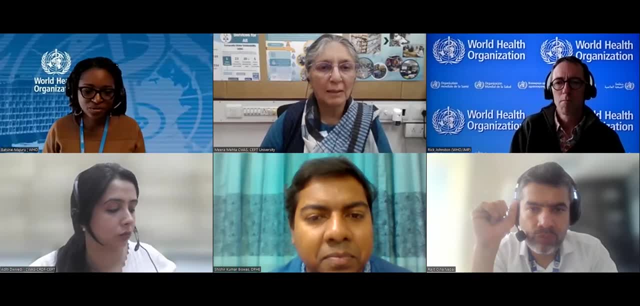 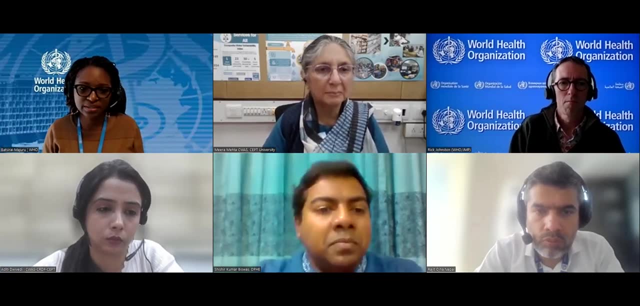 Would you like to come in with your question? Thank you, Meera, and thank you to all the speakers. So just to quickly introduce myself: I work with WHO's International Network of Drinking Water and Sanitation Regulators And I really just want to reinforce some of the points. 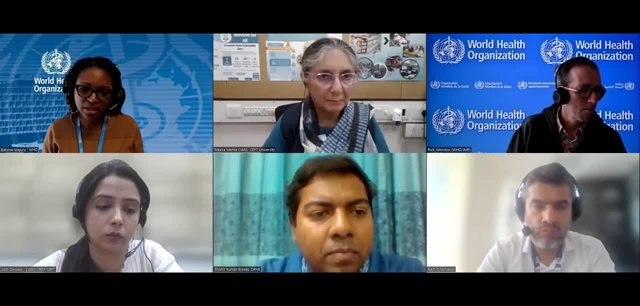 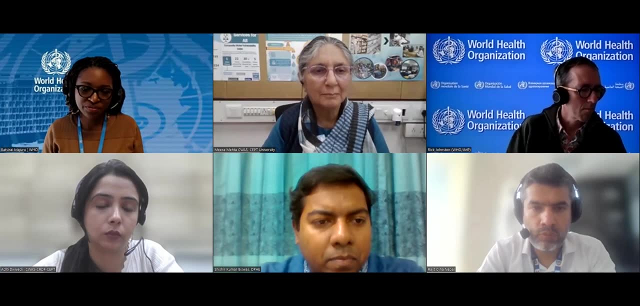 that have been made around governance, accountability and really the point that Rick, who was mentioning about who this data goes to, And maybe just to preface my statement by saying that when we talk about regulation, I think we're not necessarily referring to an independent regulatory institution. 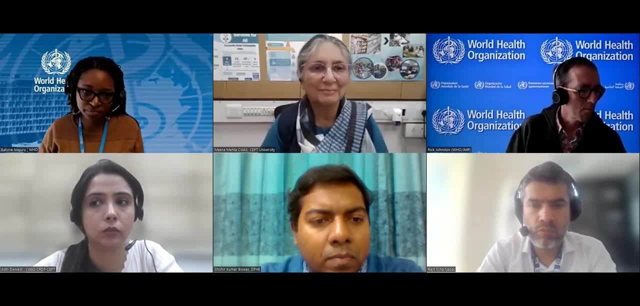 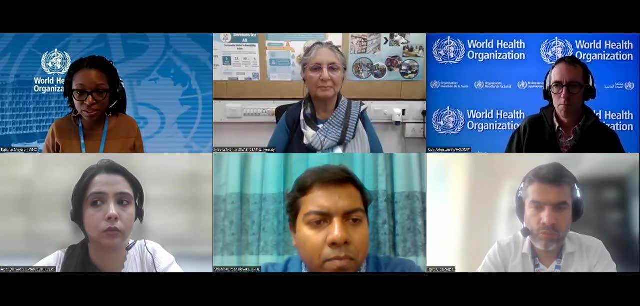 because sometimes that comes further down the path. But what we are talking about is oversight. Ultimately, who has the responsibility of making sure that these services are being delivered, that they are inclusive for everyone, that they're affordable and that they are being delivered? 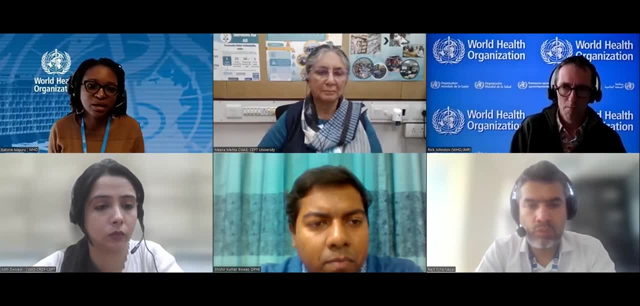 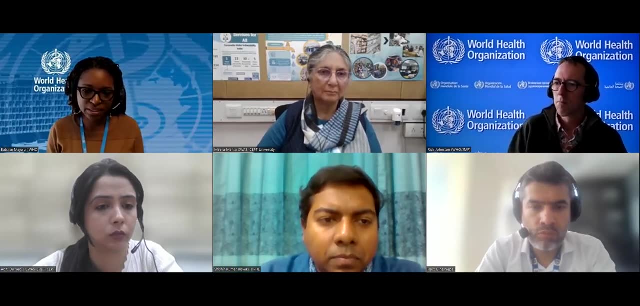 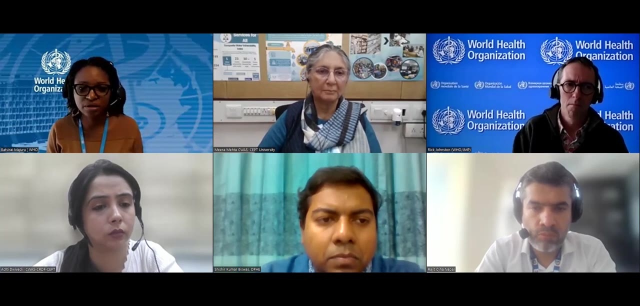 Thank you, Thank you. So I think there are a lot of countries that we can learn from in this space, in that they might not have established independent regulatory institutions, but they are conducting this oversight, and that's a good starting point. But, specifically when it comes to data, 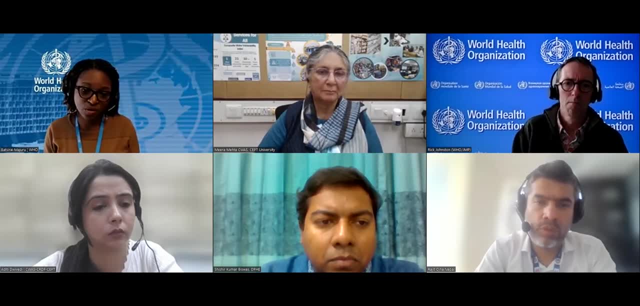 I think the key point to emphasize is that, ultimately, the buck has to stop with someone, and someone has to make sure that I've gathered all this data, we're able to understand what is happening in the sector relative to our own policy goals. 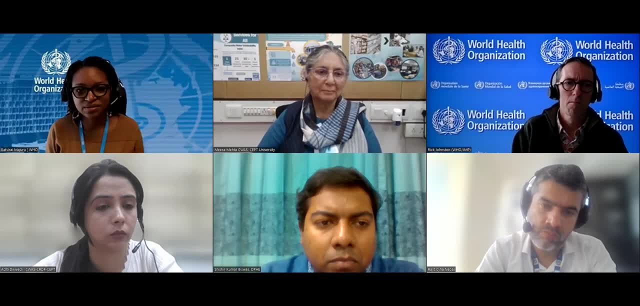 and where do we need to adjust And, like Rick said, regulators or persons with a responsibility of oversight are really well placed to do that. I'm aware that there are some efforts that have been made to establish these entities of oversight in Bangladesh, in Nepal and in Odisha state in India. 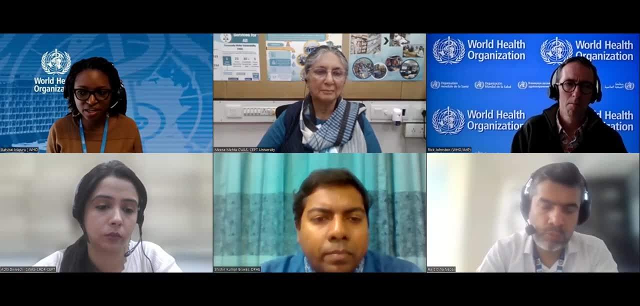 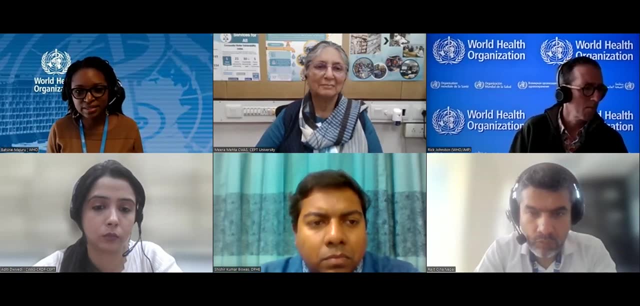 But, more importantly, also thinking about how that can be done at a regional level, so that there are more regional approaches to this oversight. How do we harmonize indicators that are being used for regulating, overseeing sanitation and drinking water services, making sure that, as a region, we're all moving towards the same goal? 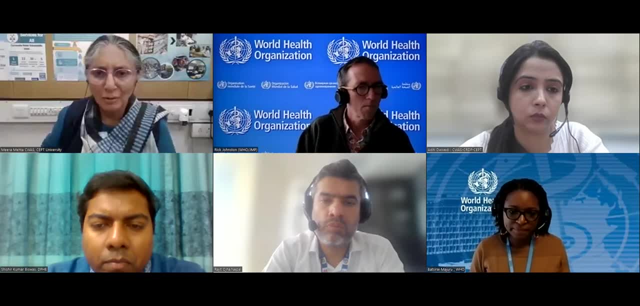 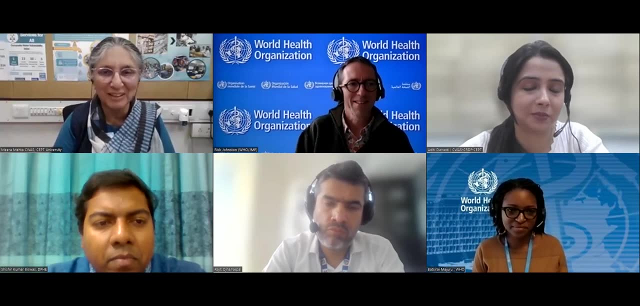 Thank you. Thanks, Bathira, I don't think there are any specific questions. if you want to come in, I have my personal opinions in terms of this whole regulation. I think it's a very interesting perspective, But maybe I don't should not really go into that here. 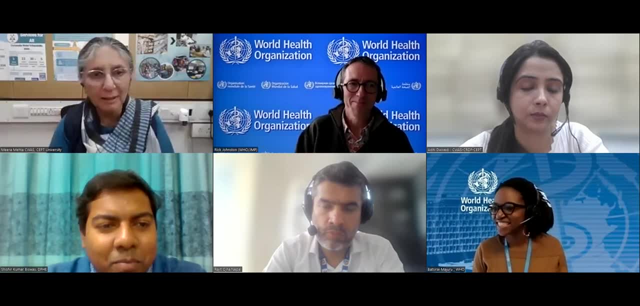 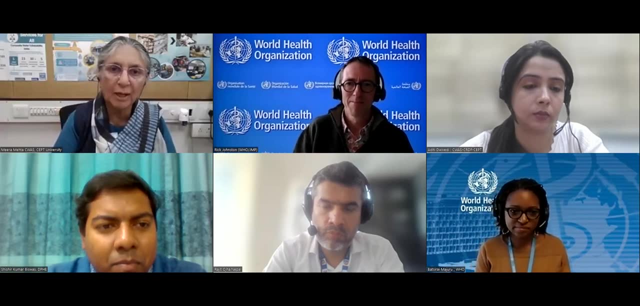 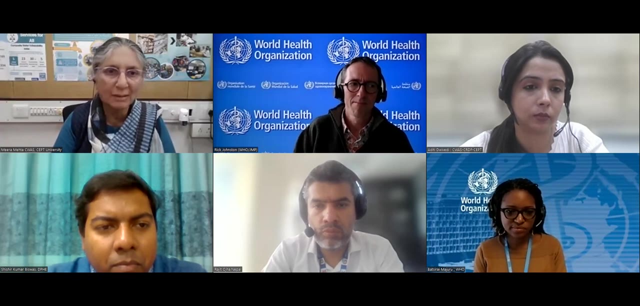 But I think what is coming out very clearly- and maybe Rajit and others can, and Shishir Aditi can, come in as to that: it is true that to have effective monitoring and effective data systems there has to be oversight by some agency. 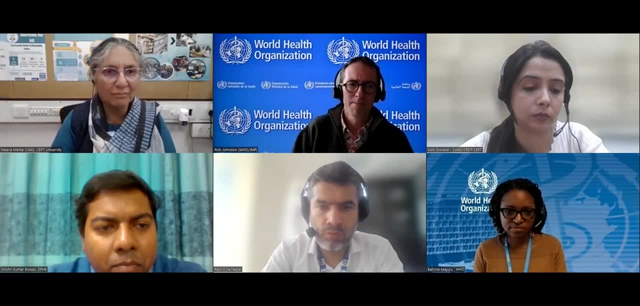 Now, whether that agency can be part of the existing government system or not, the government structures itself, and which is what I thought I heard from both to some extent, from India and, in Nepal, Bangladesh, one seems more complex than the other two countries. 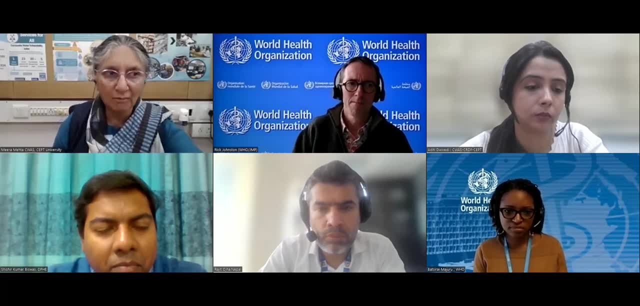 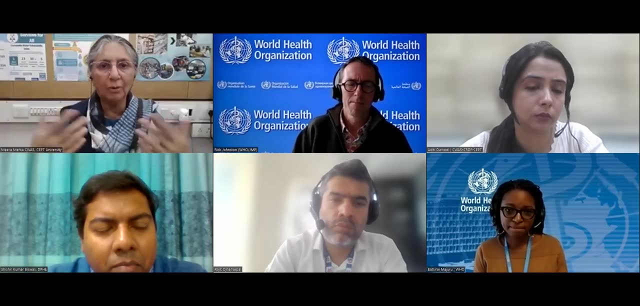 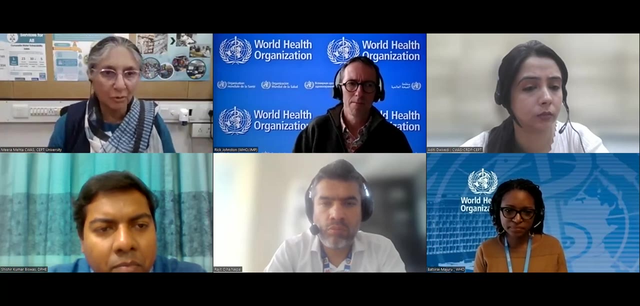 But so there is oversight. It's a question of isolating or identifying clearly who these agencies are, what their roles could be and how does the monitoring system support performing these functions better. So that is something that we really need to identify and highlight. 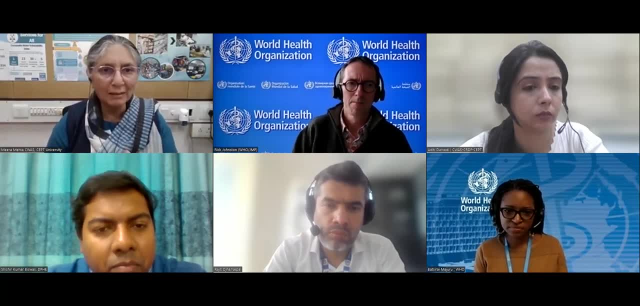 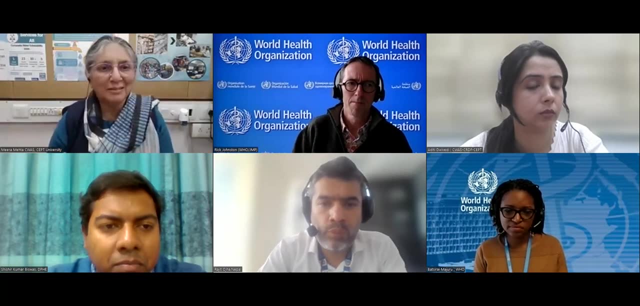 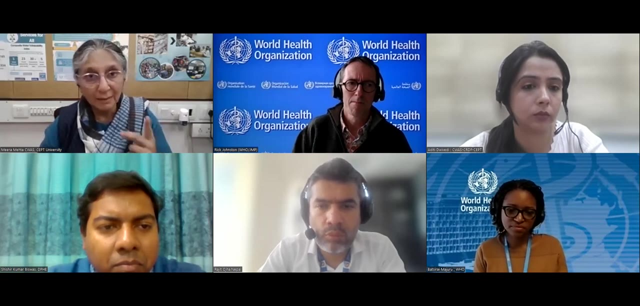 and understand better, also Because I think the whole regulatory perspective is very much linked to independent service providers, And that is not something that is likely to be the case in South Asia. to a great extent, It's not that there are. The other major issue seems to be that there are multiple service providers. 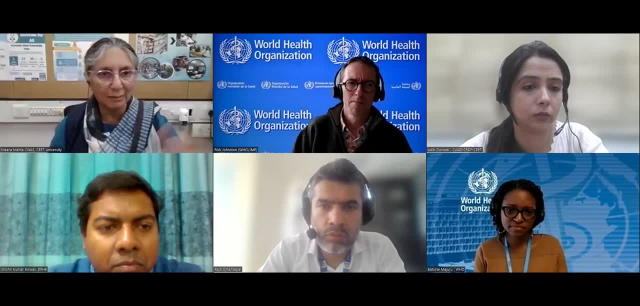 The other major issue seems to be that there are multiple service providers. The other major issue seems to be that there are multiple service providers at the local level, And I think what Rajit was also highlighting, that the clarity in terms of who is providing the services. 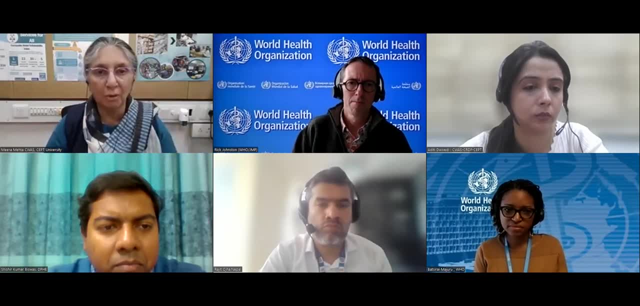 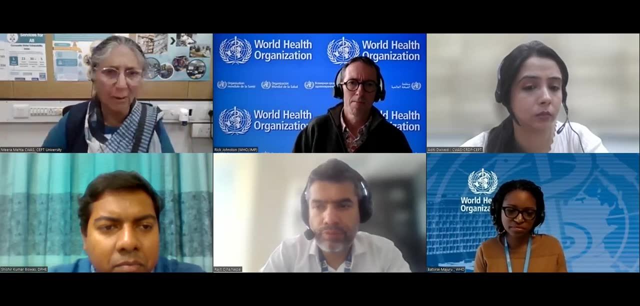 local government or private service providers and what is their relationship. these are issues that need to become part of the monitoring system itself And part of, in a way, indirectly, whatever we call it regulation or supervision or whatever term that we give to certainly. 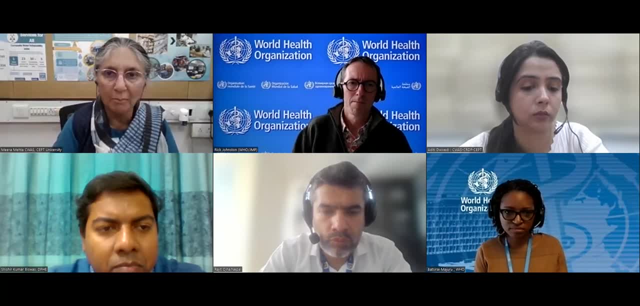 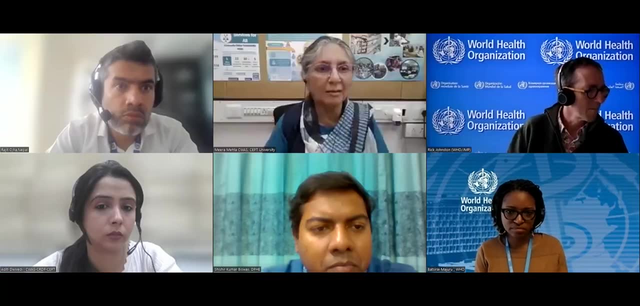 I think there were a lot of questions in terms of data. I think there were a lot of questions in terms of data quality improvements, And that's something that I don't know. what efforts have been made in these three countries, as well as from Rick and Batsirai? 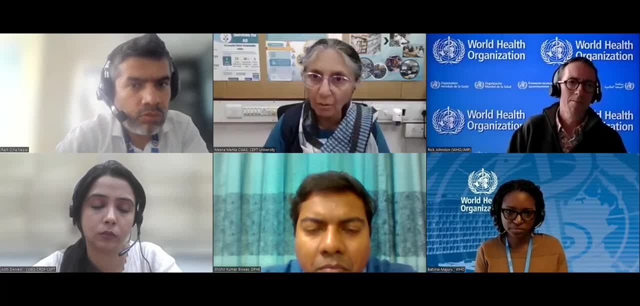 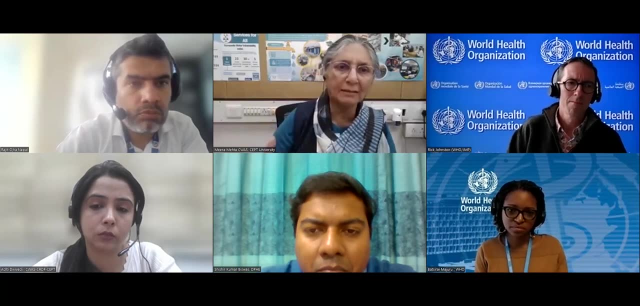 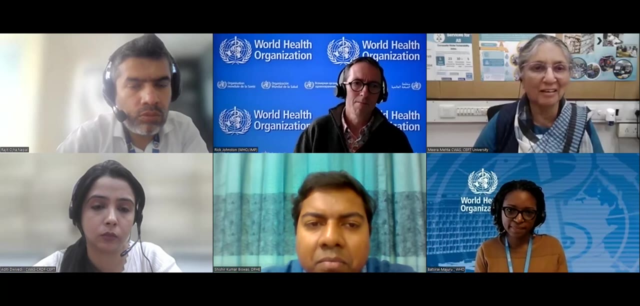 from your experience from Africa also, That how can data systems be improved and the quality of monitoring actually can contribute, Because that is by to some extent, critical to really to have belief in the kind of data that is generated. also, I have two hands up, Rajit and then Rick. 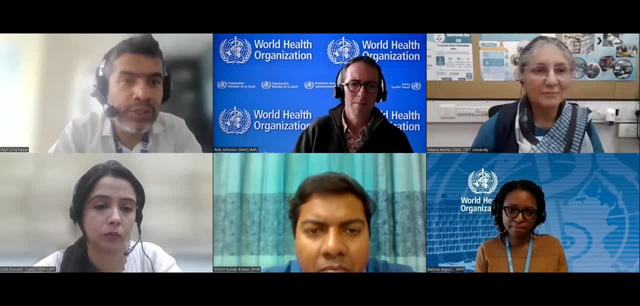 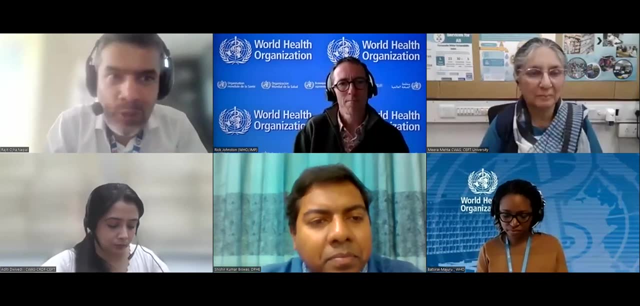 Rajit go ahead. Rick, you want to go first, or you let me Go ahead, Rajit? Okay, So just wanted to highlight one of the things we are planning to do. It is in research phase, but I think it will come good. 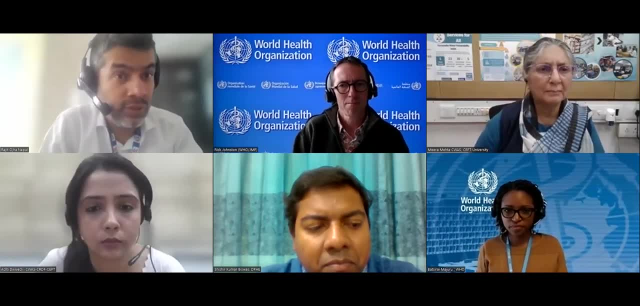 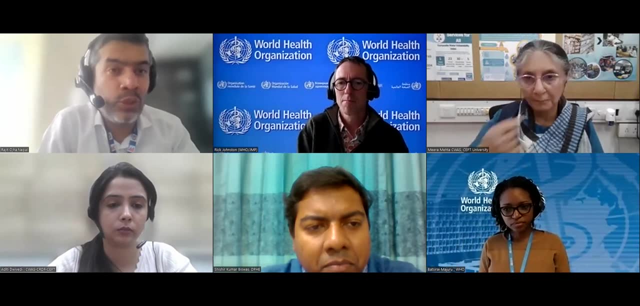 So what we did was like we're capturing the georeference data, and there were a lot of images which were used in order to achieve the georeferencing right, But when we started collecting the data, we knew that these image sources also can be one form of data sources. 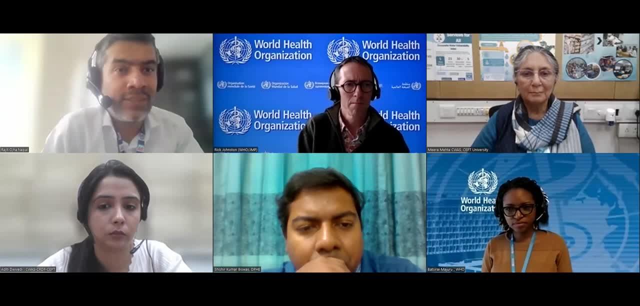 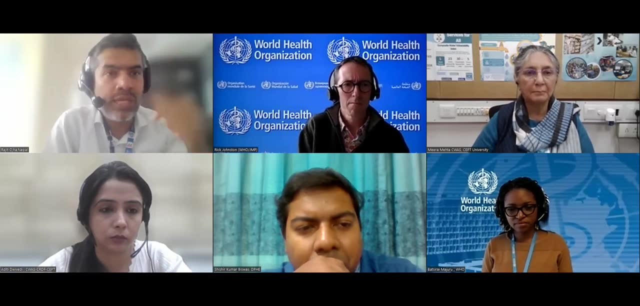 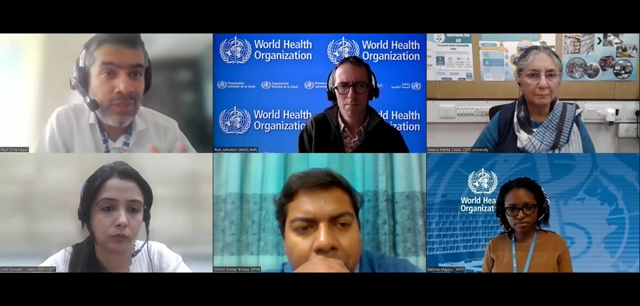 If we properly do the image processing we can see where are the data risks. So, for example, like if one tap, if one tap of, if one water tap is broken in image and someone has put this is in good condition, then these data. 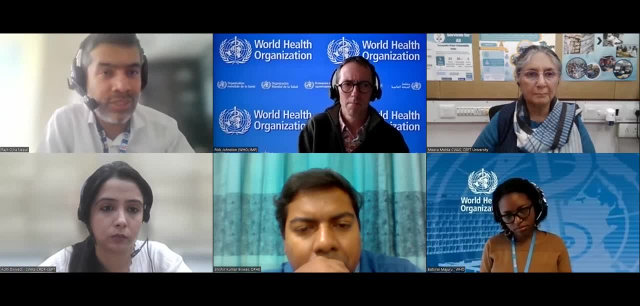 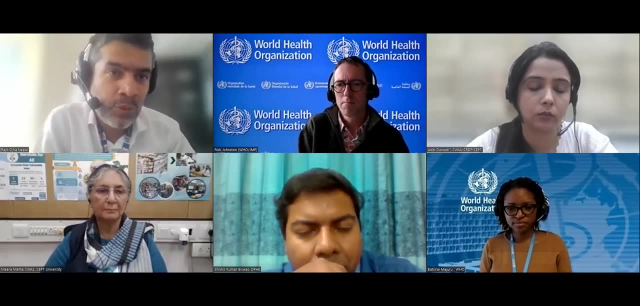 these two data are violating And image processing can easily say this data is violating. This has the like risk of violation of the. this has the risk in terms of quality of data. So this way we can create the data patches which are like: 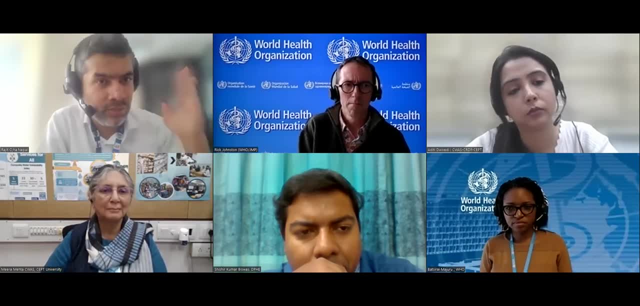 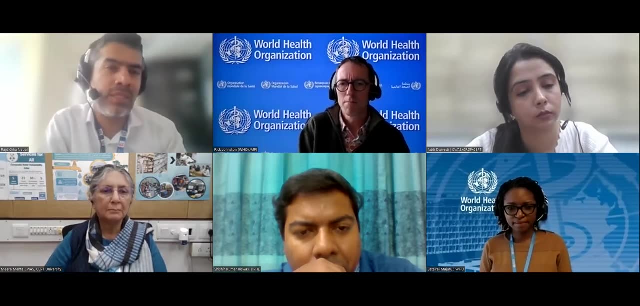 which are more risky data sets, And there we can focus more on validation. So in sanitation for example, like in the public toilets, the toilet pan is not clean as it should be, But if the data is coming like it is clean. 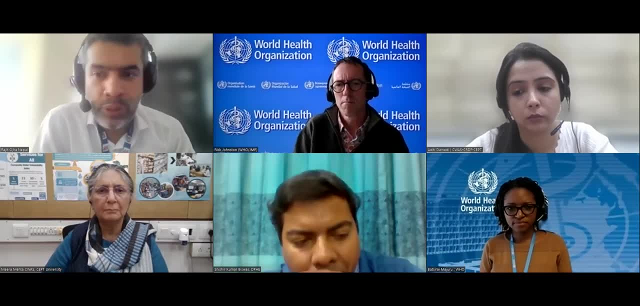 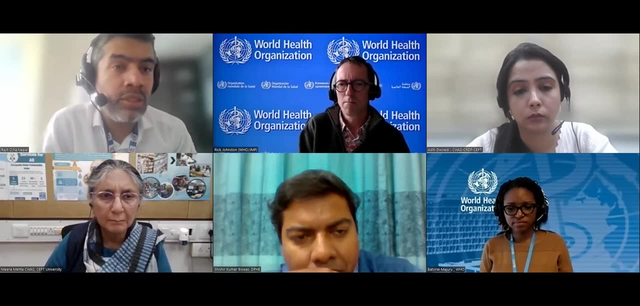 and if the image is there, so the validation of the data. it would be a lot more easier. So I think we need to. we can use some innovative solutions in validating the data, And machine learning and image processing can also be one of the examples. 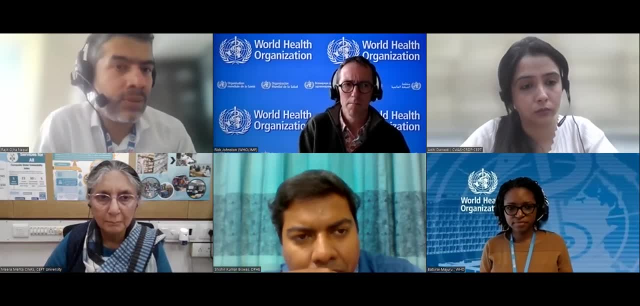 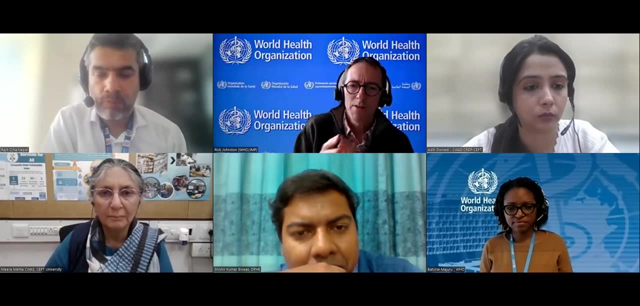 that we can push forward. That is Nepal's case, So just wanted to highlight that. Maybe there can be other examples also, but this is one of the case from Nepal. Thank you, Yeah, On the question of data quality. So one of the questions was: 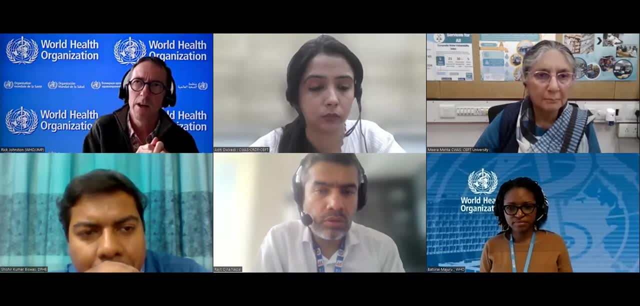 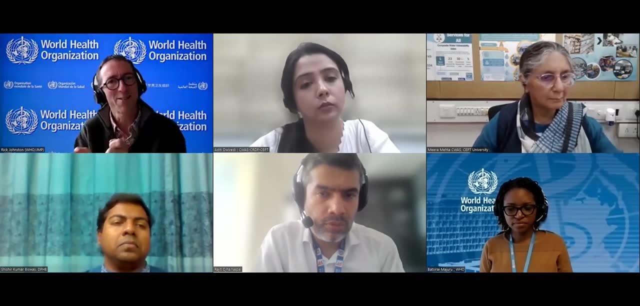 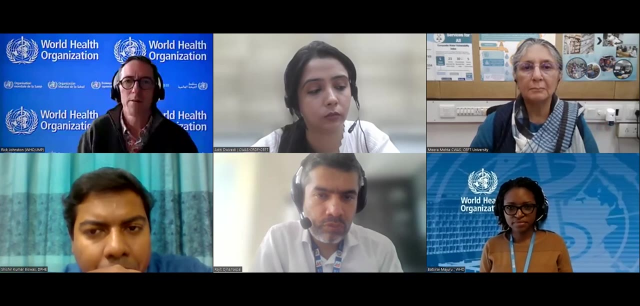 is digitization the way to ensure data quality And I think digitization is really important and it certainly increases data accessibility but not necessarily quality, And it relates to this tension I see between the types of information you can get from routine household surveys. 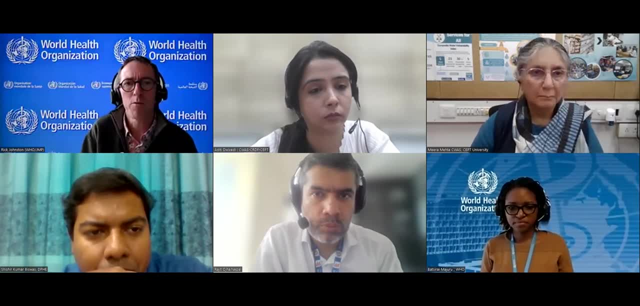 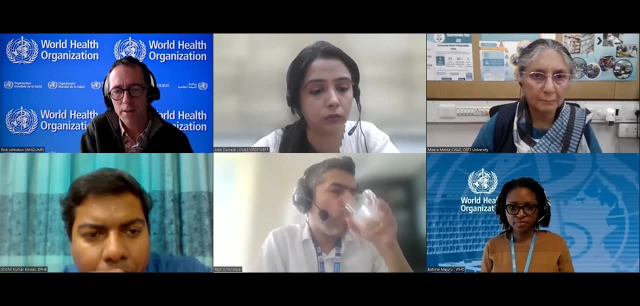 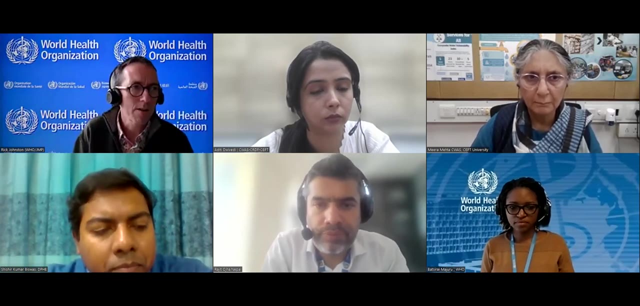 and the types of information you can get from routine administrative data systems And there's a transition And I think the three countries here are at stages of that transition. If we look at, you know the high-income countries, they don't collect data on WASH in household surveys. 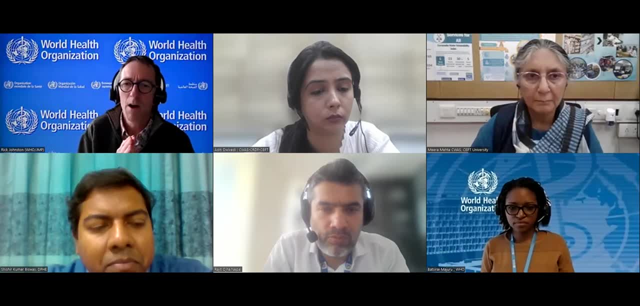 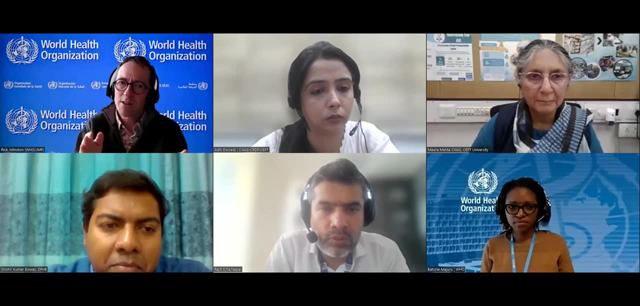 They have comprehensive administrative systems And the very low-income countries they don't have any administrative systems, so it's only household surveys. But these countries, they're in transition. So I think there are challenges when you try to build up an administrative data source. 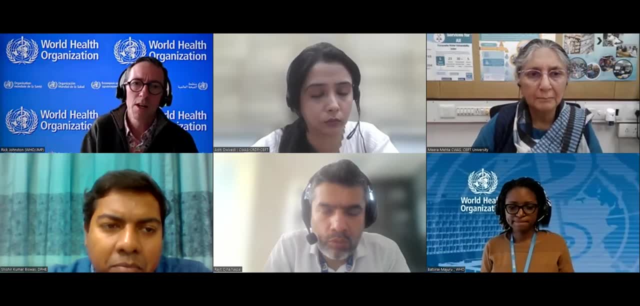 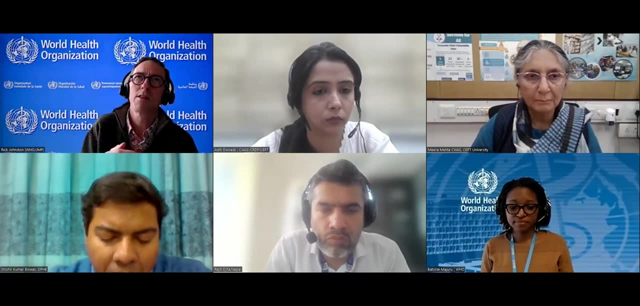 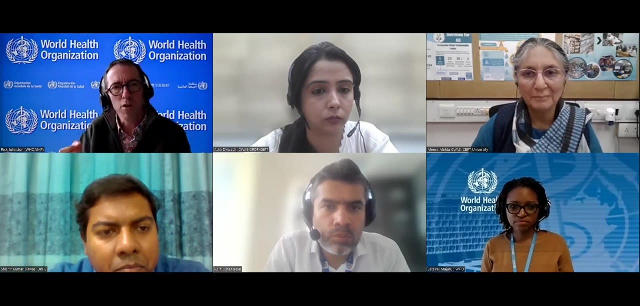 around data quality. One challenge is around just geographic scope, and are you really capturing data and monitoring everyone? And especially as administrative data sets are in their early days, there are data quality problems. You know it's the stronger-performing local government institutes that give data. 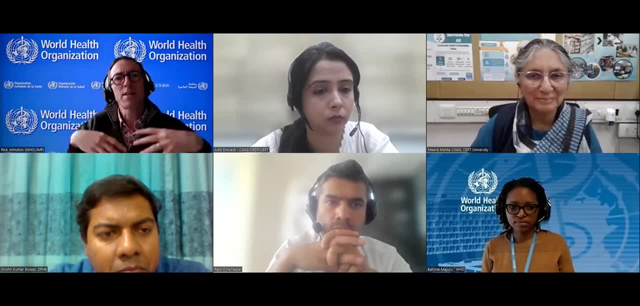 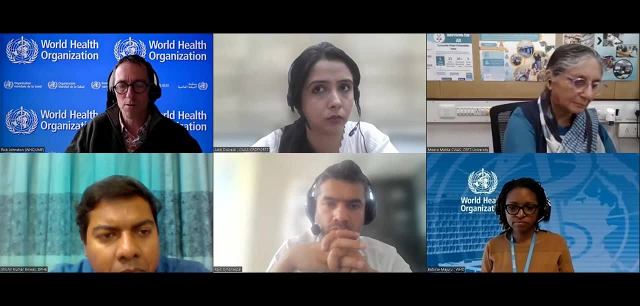 and then the weaker ones don't give data, so then the data aren't representative. It takes time to get to a place where you have reliable administrative data, And I think in all three of these countries you're making steps towards that and advancing it. 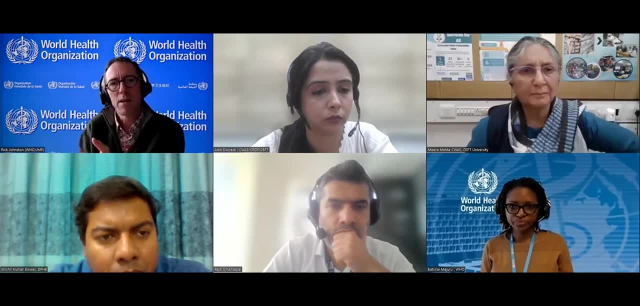 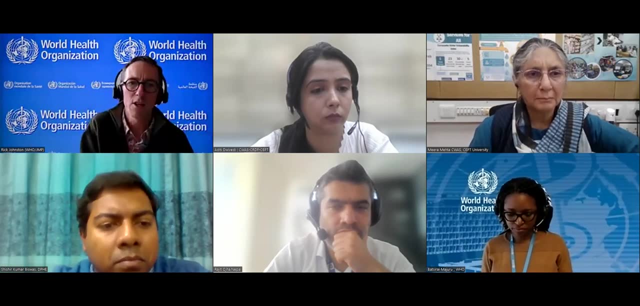 I think ideally there's a primary reliance on routine administrative data, but with some kind of ground truthing or Rajit. you mentioned validation. You know spot checks Just go to the field, whether that's households or service providers. 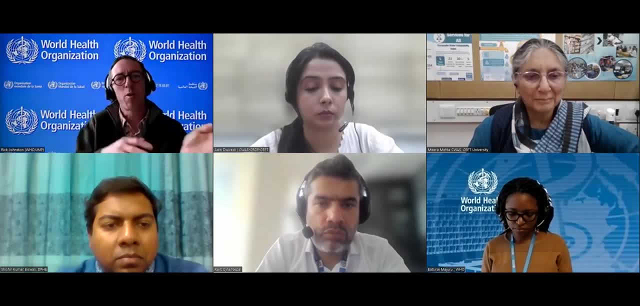 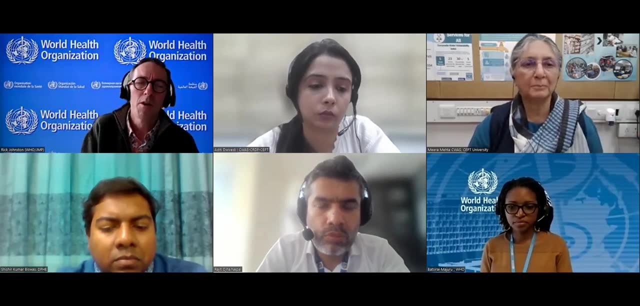 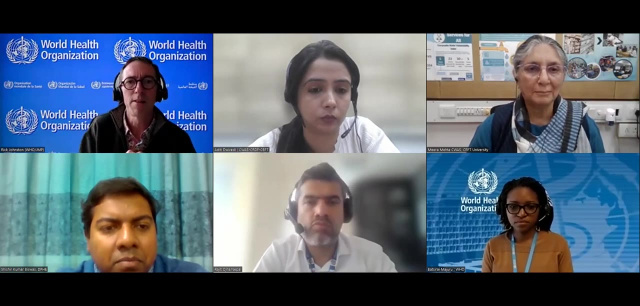 and you know, check that what you're getting from your main source of data is really reliable. because, again, especially when these systems are new, you know there are incentives to take shortcuts or to say things are better than they are. So there are challenges with data validity. 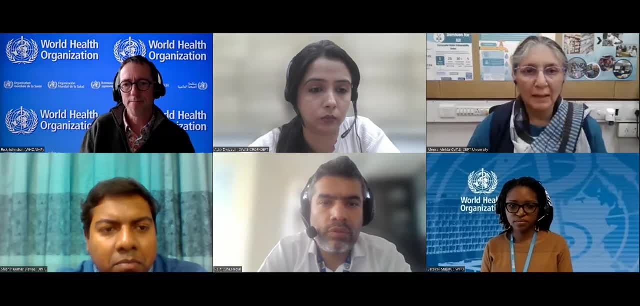 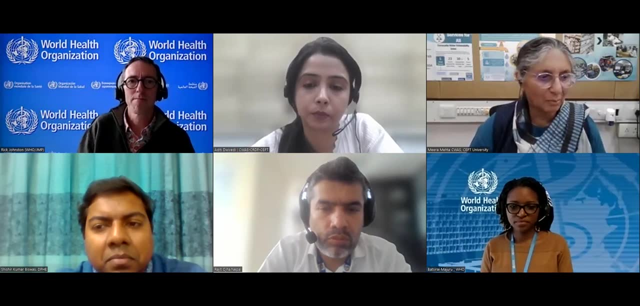 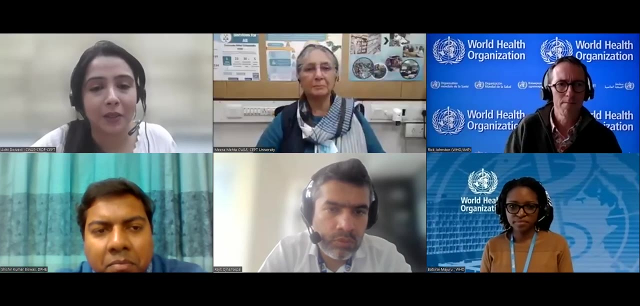 in the early days of administrative data systems. Thanks, Aditi, you want to come in And also if you want to highlight more the links related to possibilities of climate and sanitation, and how would you contribute to that I also? First, I wanted to again touch on the digitization. 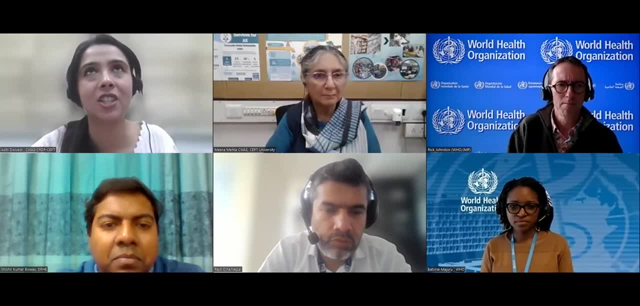 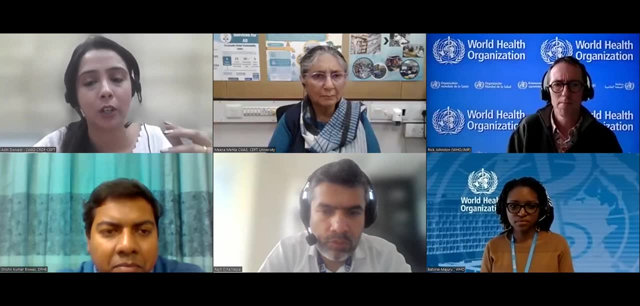 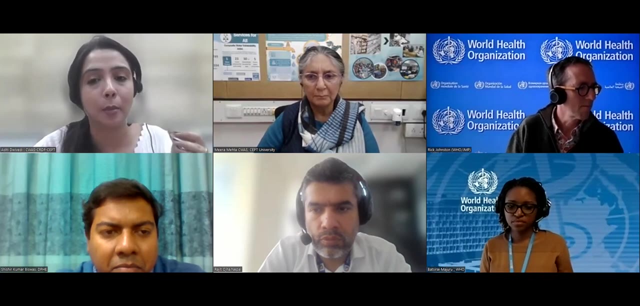 and the technology aspects. While technology and digitization does not necessarily, you know, mean better quality data, but it provides pathways to improve the quality of data And I mentioned the system of you know data, Mentioning the data reliability in the past module. 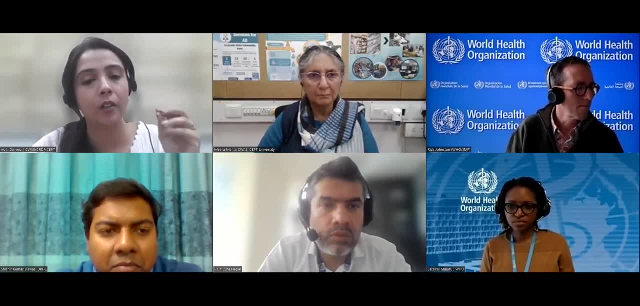 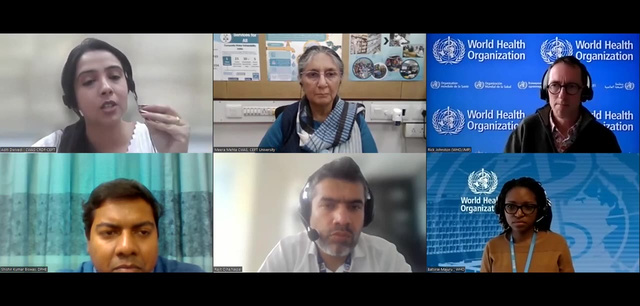 While that means manually, you know, putting in reliability A, B, C, there are also a parallel system of automatic data validation checks- So there are around 300, you know formulas or data checks that check the quality of data. So, if you've mentioned X number of households in this, 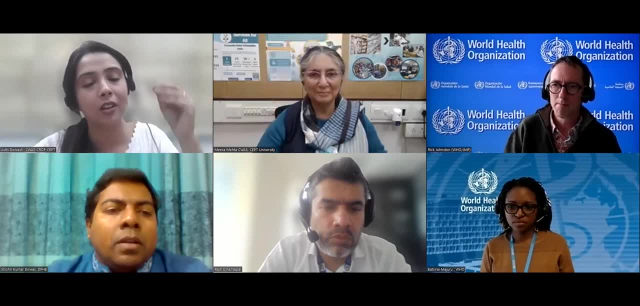 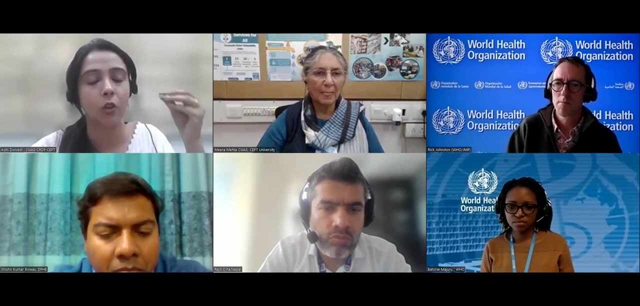 You've reported X number of households last year. you cannot, you know. it just shows a warning that you cannot show a lower number of households or connections this year. So those kind of checks. the amount of groundwater you've extracted cannot be more than the total amount of water. 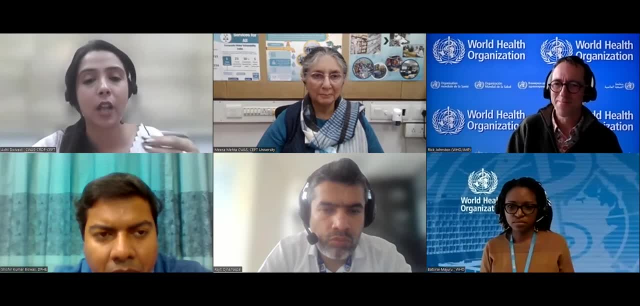 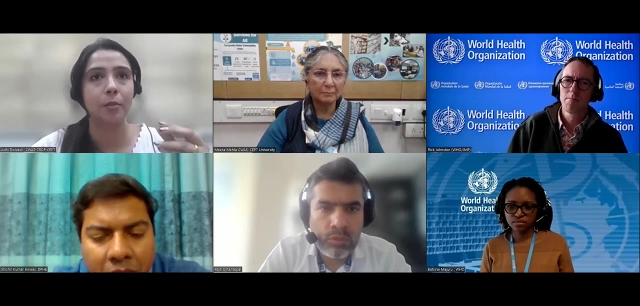 you know production you have reported this year. It enables those kind of pathways. The other thing is it also enables you know the human, The human mistakes, So the human oversight. it eliminates that that could happen. So, for example, when we worked in sanitation, 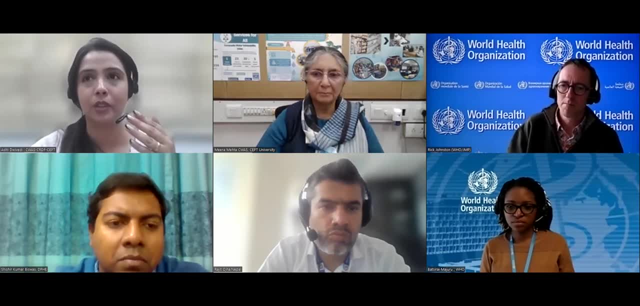 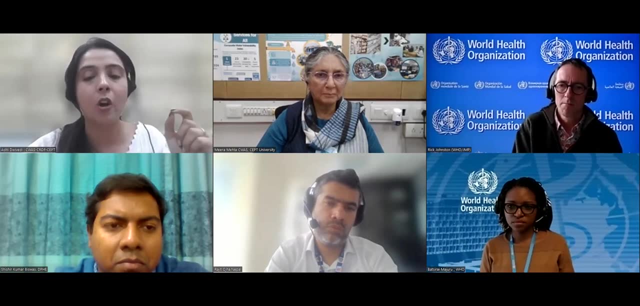 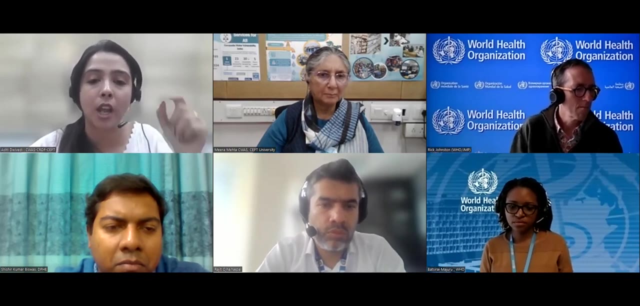 and monitoring the, The dislodging services. in a few cities they used to work with logbooks. Or even you know the provision of water supply. They work with logbooks with you know how much time the water has been supplied. 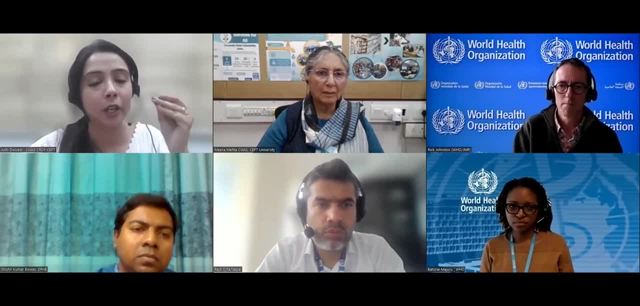 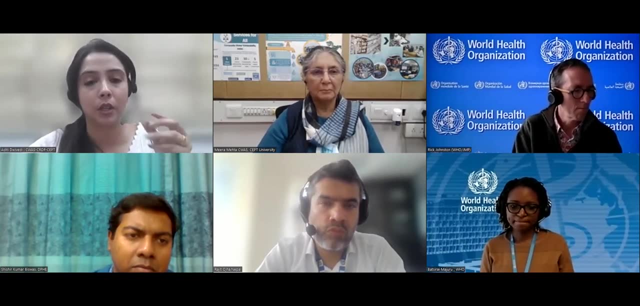 how much time the pumps have been working or how many times the dislodging, The dislodging truck went to this house. But then, as soon as we introduced an app to monitor this service, we could you know- suddenly start collecting. 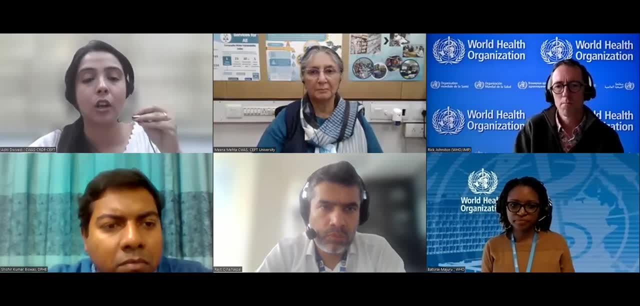 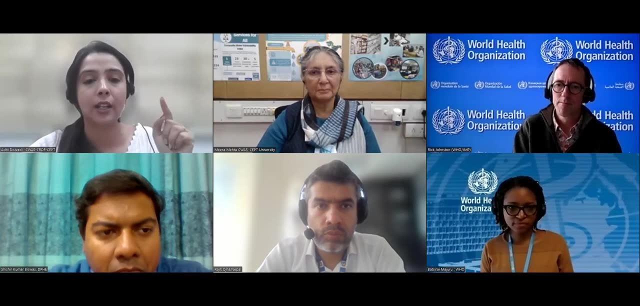 automate collecting the geolocation and then we could track whether this dislodging has happened and whether it has gone to the correct place or not. We could automate checking that and we did not have to physically check it. So it provides pathways. 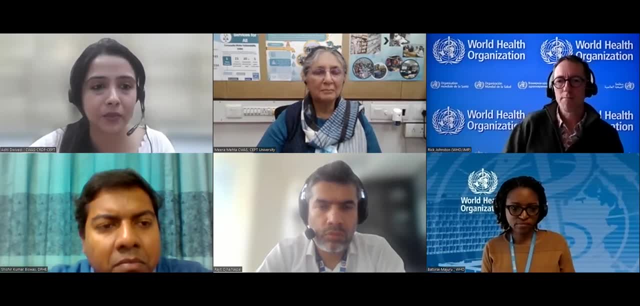 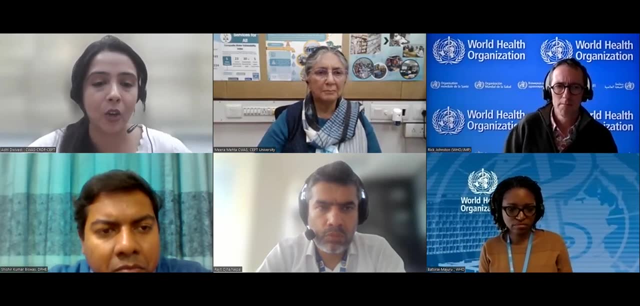 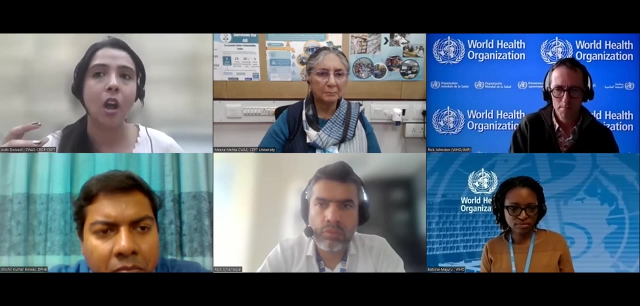 And to touch on the aspects of climate. while climate is a very important topic right now and there is still, you know, evidence building on how sanitation contributes or is helpful in mitigation efforts, while there is, you know, evidence is still building. 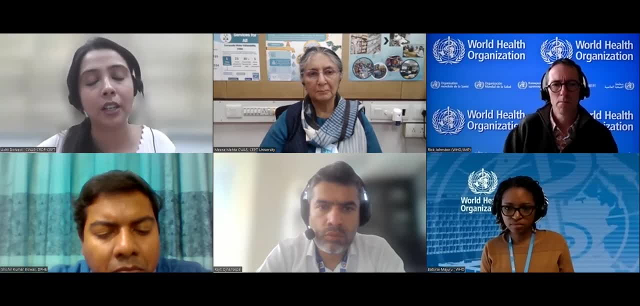 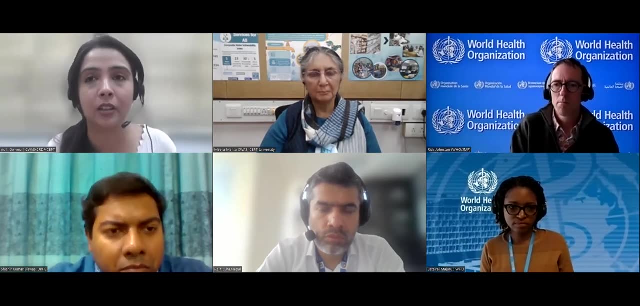 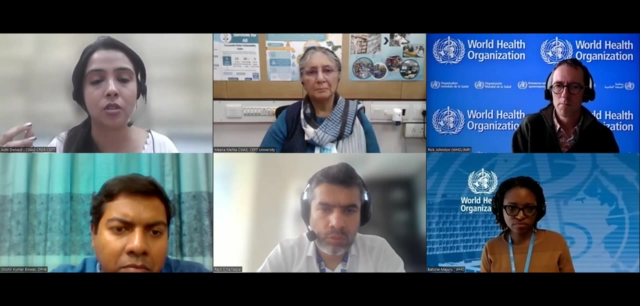 we do know that. you know, work in sanitation would be very, very much important in climate adaptation And at this point there is a big need to focus on that because the ill effects of climate change are very much visible and impact sanitation and water. 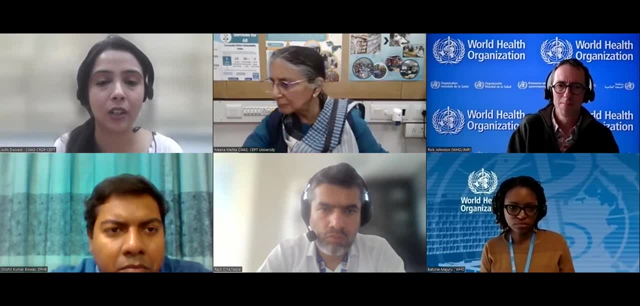 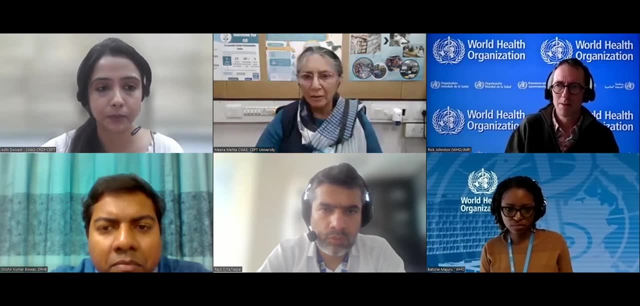 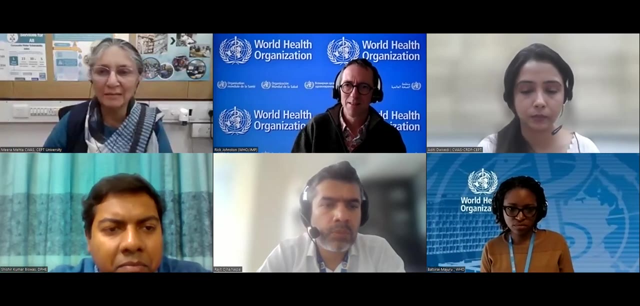 So that is how climate comes in in this sector at this point. Thanks, Aditi, I don't see any hands up. I had a sort of small query to put to all the panelists that everybody talked of the need for household survey. 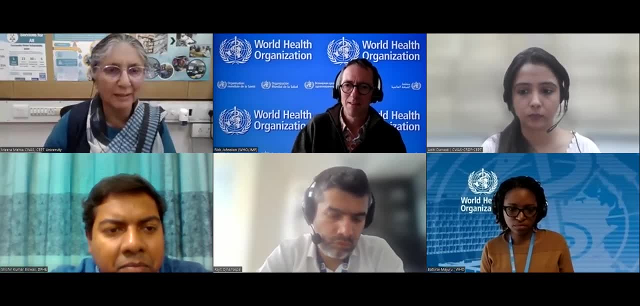 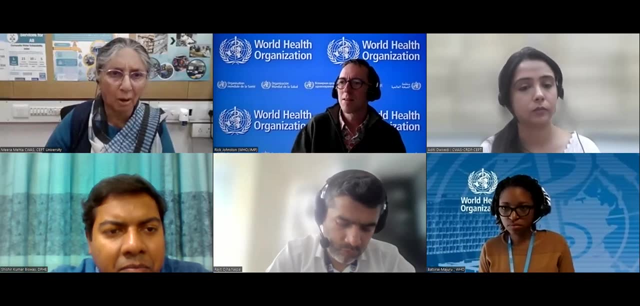 on a regular basis and that they should be good. there should be local data available In all the three countries that we looked at and I assume even in Africa this would be true- that property tax is a major source of income and there is regular household surveys. 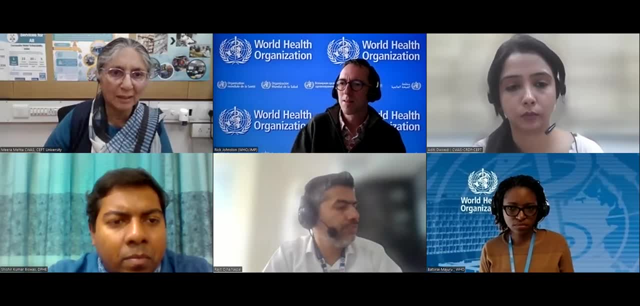 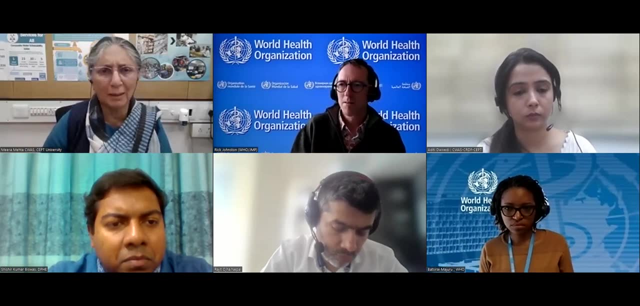 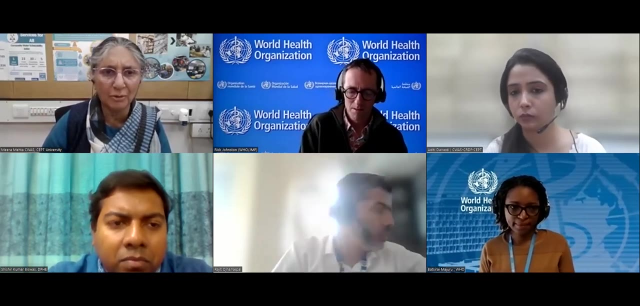 that are done for updating property tax database. It's once in three years, once in four years. This is taken up across all cities, in India at least, I assume that this will be true in Nepal, Bangladesh and so on also. 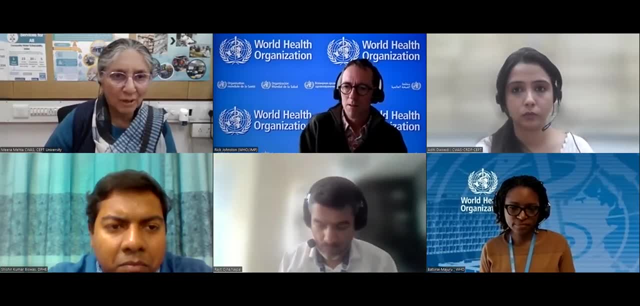 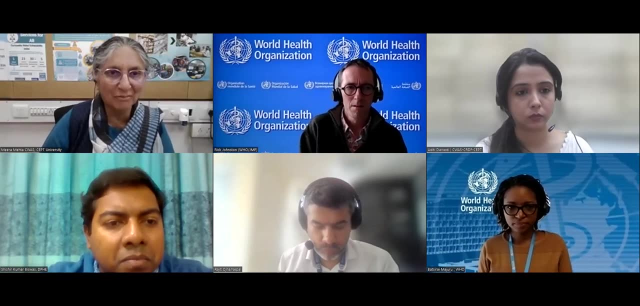 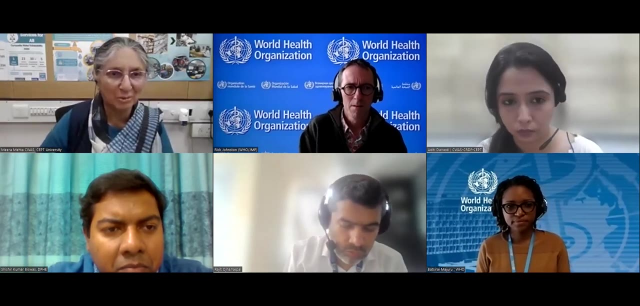 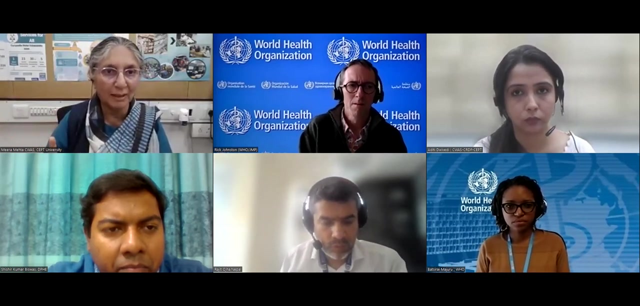 Would that be a possibility to consider? So it's not the kind of surveys that Rick and team depend on. in terms of surveys that are- how do I say representative? representative of through appropriate statistical method- selected, but property tax is 100% survey that you will get. 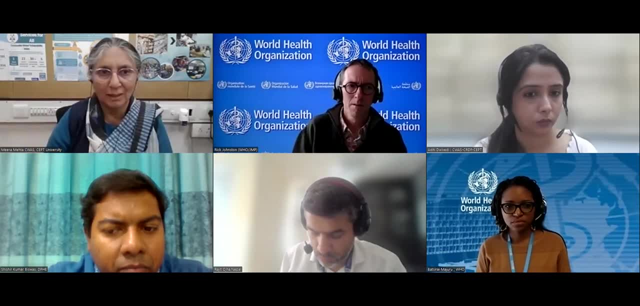 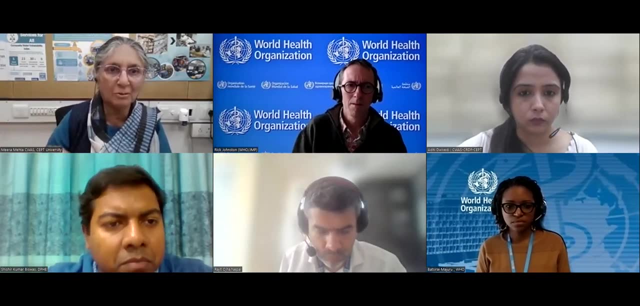 And it's done every three to four years in all in India, across all six states, all cities. this is being done, But we have never attempted to tap this source to gather more and better information about water and sanitation, not only san. 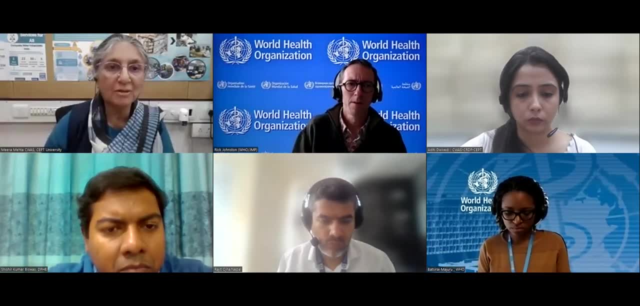 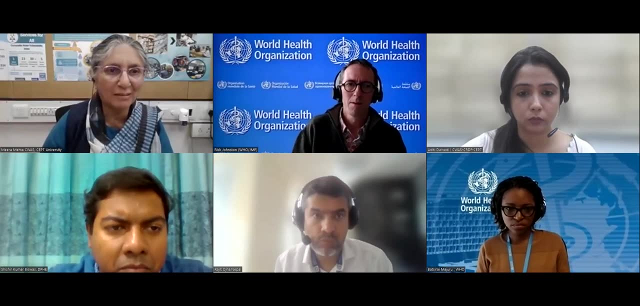 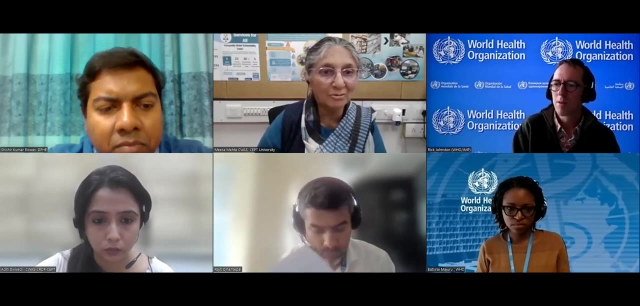 And, in fact, to some extent, solid waste also- it would be possible to do, And whether any thought has been given to this. we've made some attempts but still need to do much more, But it would be interesting to hear whether something like this would be possible. 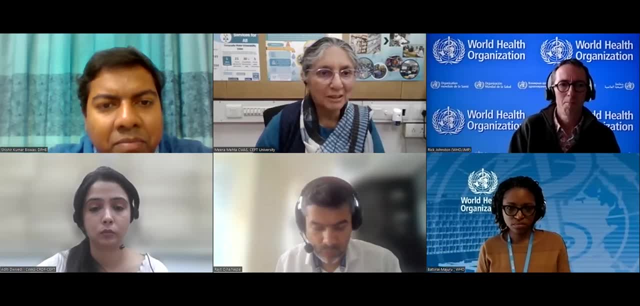 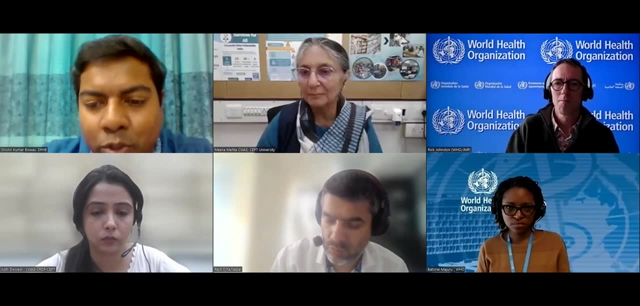 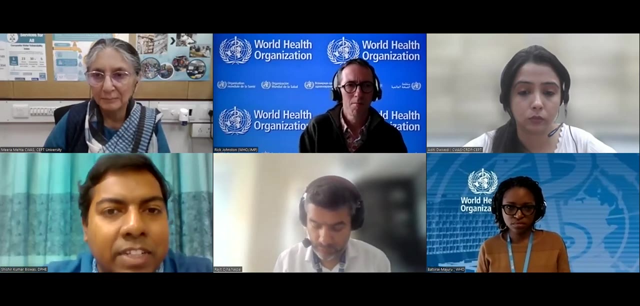 in Bangladesh and Nepal also, Shishir go ahead. Yeah, you have rightly mentioned. actually, you know that first time- because, where there is no service, household survey is the primary tools to get information and collecting data, preserving the real. 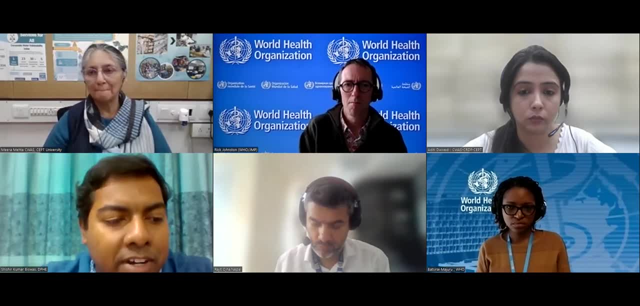 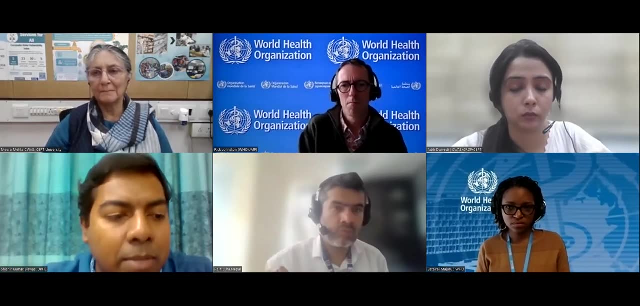 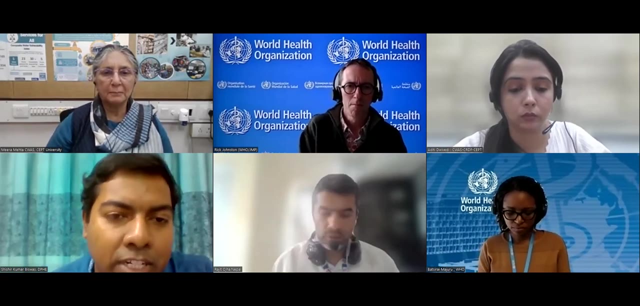 You can say the situation analysis. So when, after getting this information, when development activities actually we are conducting, let's say, not so huge scale, but gradually in one project. according to my experience, in 23 municipalities project we have established the complete value chain. 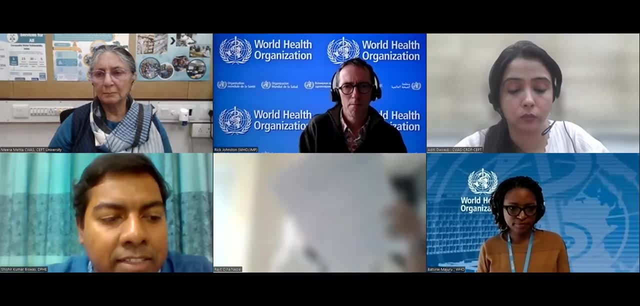 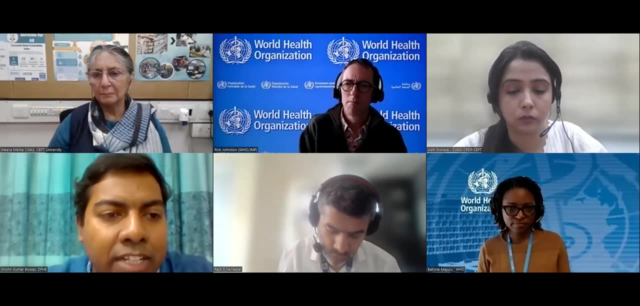 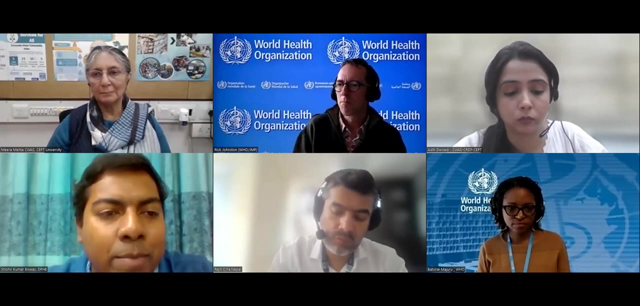 for 11 municipalities. So now, after getting the baseline database, so now establishing this complete value chain automatically. the information are coming from the municipalities, So no need to get the information by again. household survey. So yes, we are thinking that at a certain stage. 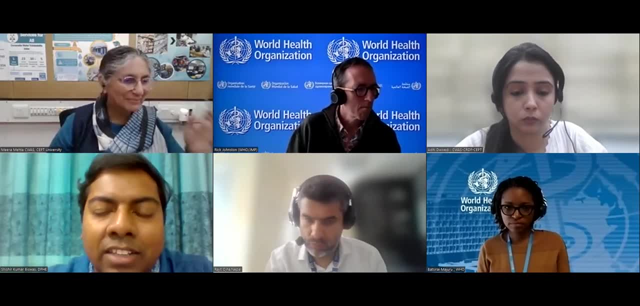 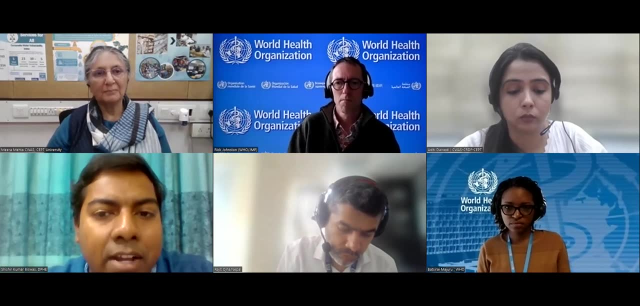 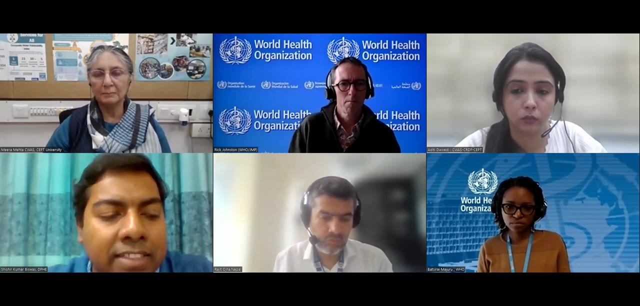 we will provide the service and gradually those information automatically will come from every household and from every component of the value chain. That's why we have the expanded version of the IMIS for the every municipalities, collecting the household data whether they are getting quality water. 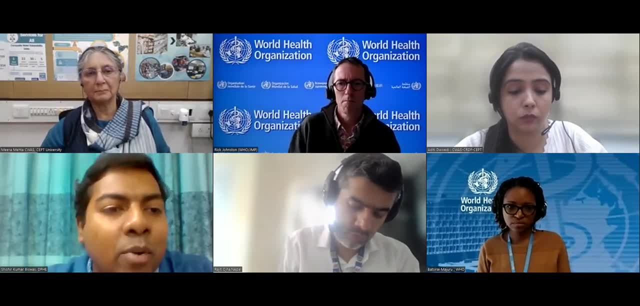 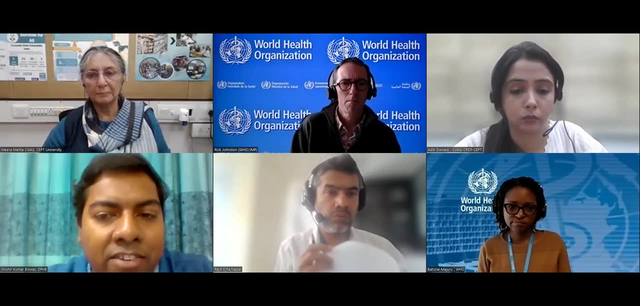 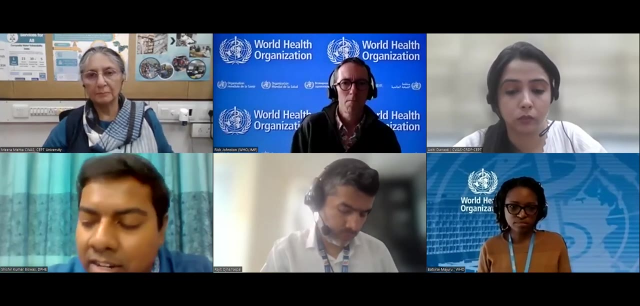 whether they are getting the waste management services, both the FS and municipal solid waste. So these are under a trial basis. already We have completed around 10 municipalities. they are doing well And, based on this survey, some other interpreters are coming forward. 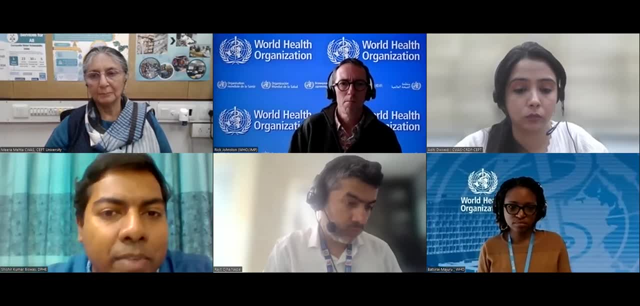 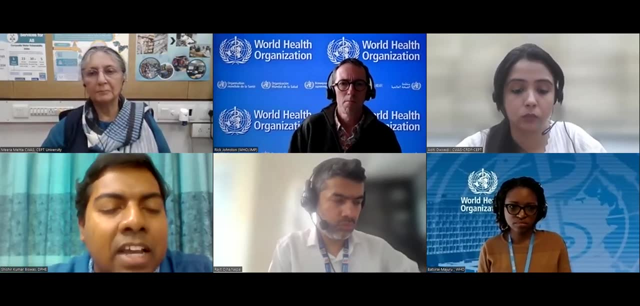 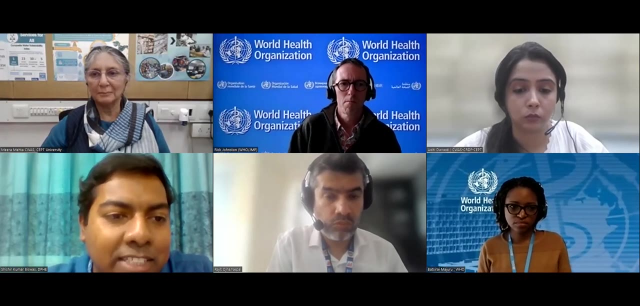 And the municipalities also getting habituated on it. So I think if this concept can be expanded to other municipalities, I think the better information will be gathered and collected, preserved, and no need again and again the baseline survey. Yeah, thanks. Yeah, that should certainly be looked at. 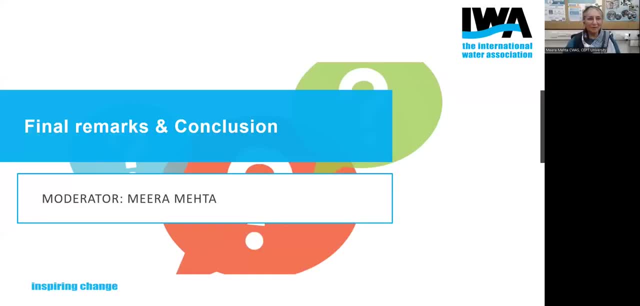 I think I'm being told to do final remarks. I thought it was better to get final remarks from all of you, but maybe I am supposed to do I think it was. Can you please remove the slides so I can at least see everybody's faces? 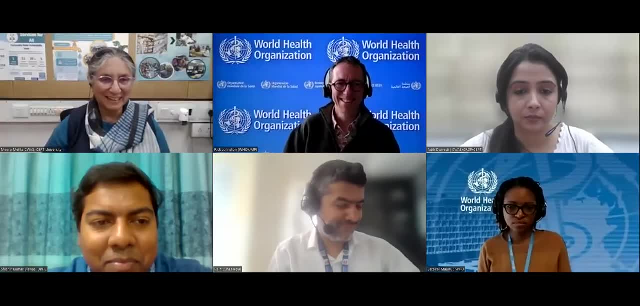 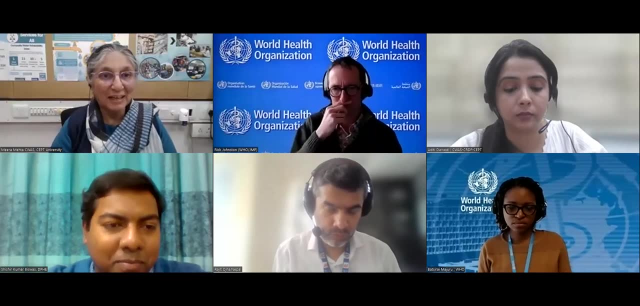 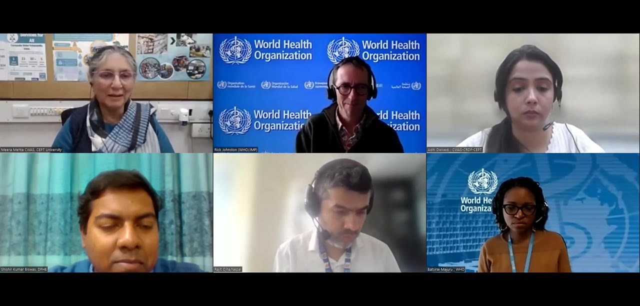 It's much better. I think it was a great discussion. I don't think that we've come to any conclusions And I don't think it was expected that we would come to a conclusion through just one webinar like this, But I think it raised many important questions. 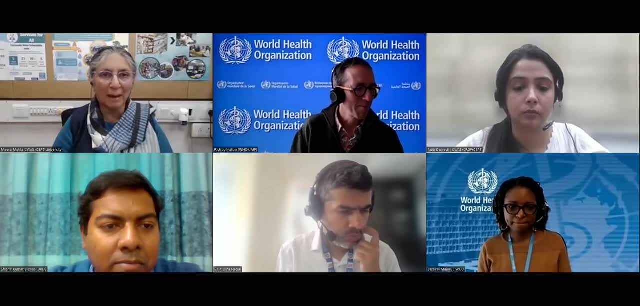 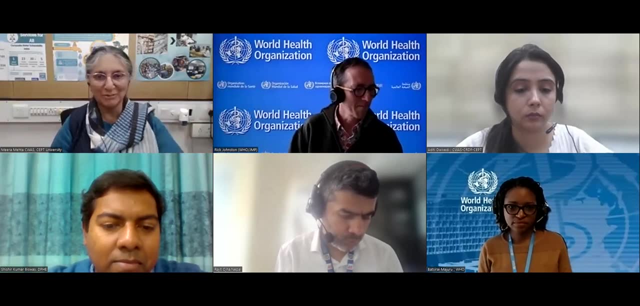 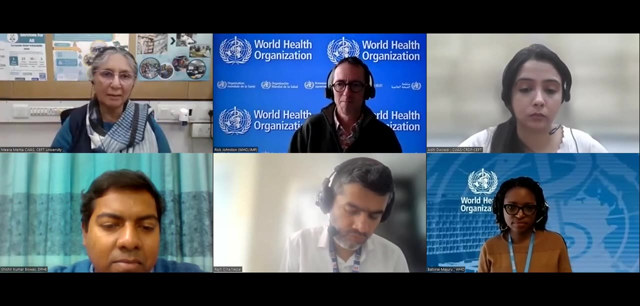 and it is excellent to learn about what's happening, both at the global level from JMP, which we know about, but it was good to hear Rick say the kind of processes that they've also adopted, as well as the country level experiences, And I hope that IWA and our institute 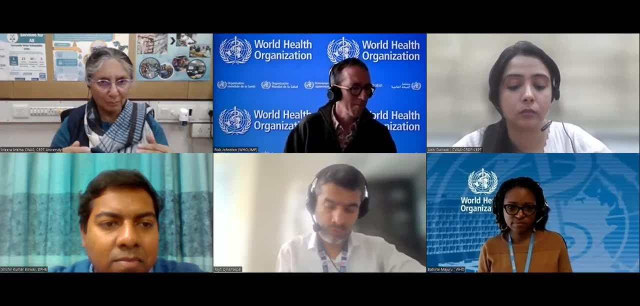 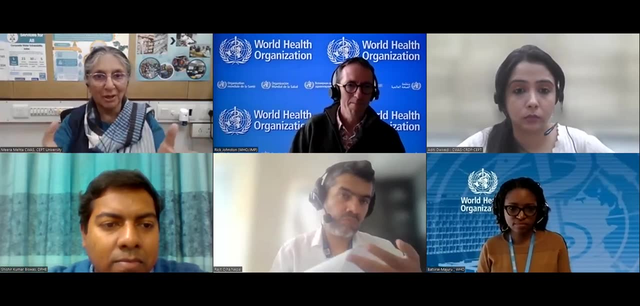 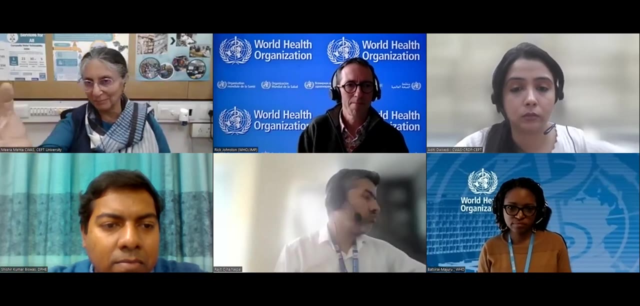 will take this forward in terms of how do you build on the kind of discussions that we had and how do you go one step forward in terms of whether it is through a regulator or whether through some kind of a reporting agency, whether through household surveys or IMS that you were talking about.